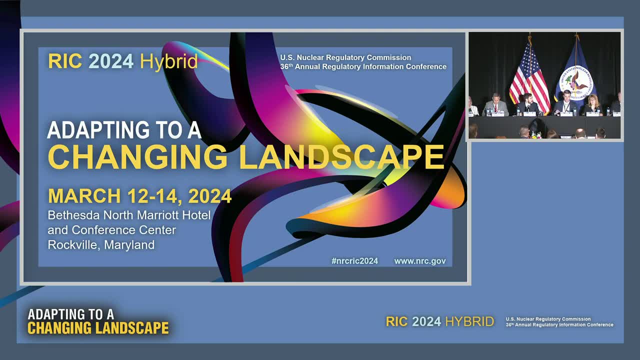 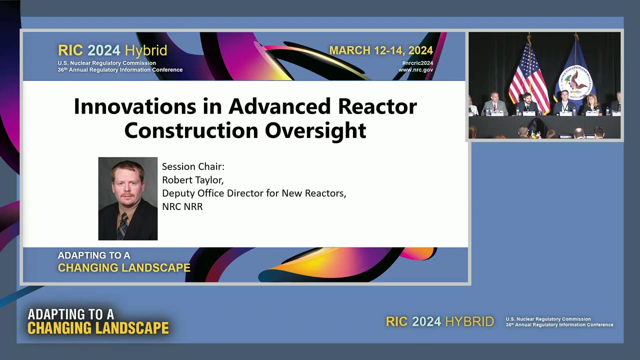 Good afternoon everyone. Go ahead and take your seats and we'll get started here. I want to welcome you to this session where we're going to talk about innovation and advanced reactor construction oversight. My name is Rob Taylor, I'm the Deputy Office Director for New Reactors at the NRC and I'm joined by an esteemed panel that I'll introduce as they make their presentation. So thank you for coming today and joining us at this session. I'm looking forward to a good discussion and we look forward to your insights, perspectives and 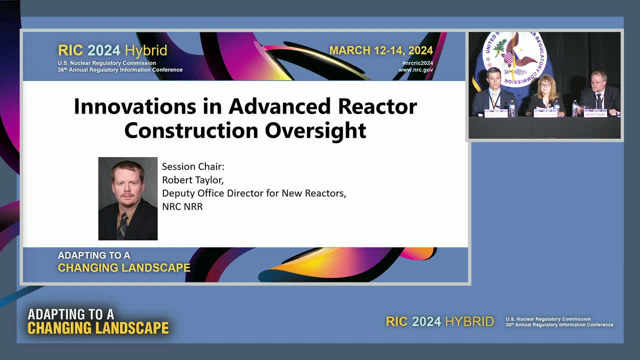 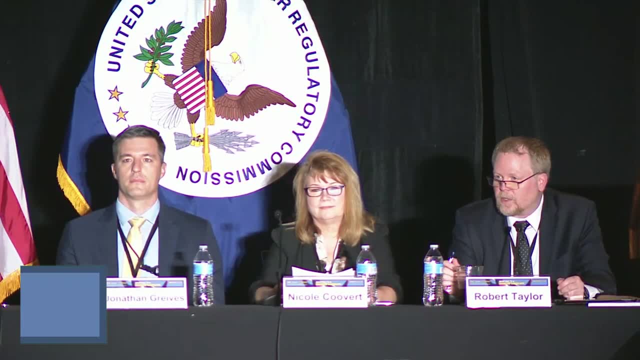 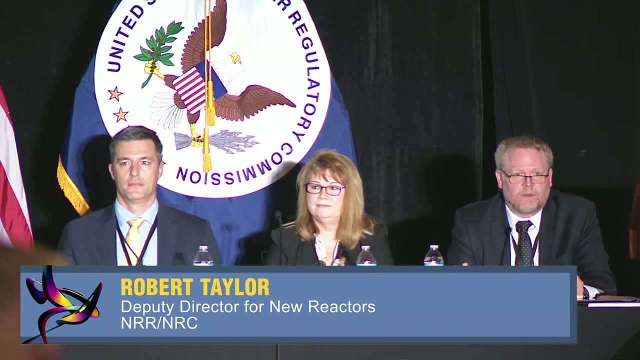 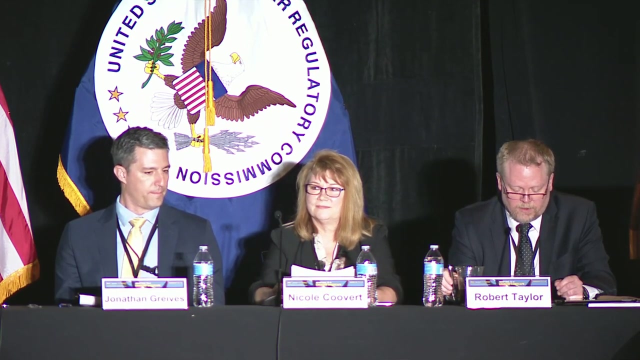 questions as we go. So we're going to follow a moderated panel discussion format. Following the presentations from our panelists, we will have a guided discussion and take questions from the audience with any time remaining. So please use the QR code for the session to ask any questions, because if you don't, I have a bunch lined up for them and I'd rather get to your questions and make sure that we have plenty of time to ask those So you may submit them at any time. There's no need to wait for the QA portion of the session. 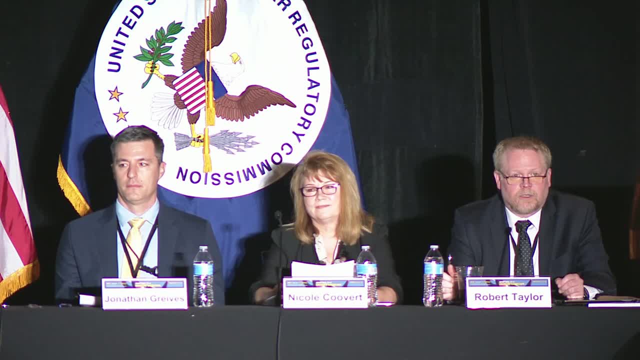 So, as you've heard, a major theme for the NRC and the industry is the deployment of SMRs and advanced reactors And in looking at that we have to take a holistic look at all the aspects that are needed to support the transformation needed to deploy these technologies. And we recognize that advanced reactors are going to pose new and unique challenges in a number of different areas, including construction oversight. So as we undertake these activities, we need to make sure that they're commensurate with the risk profile. 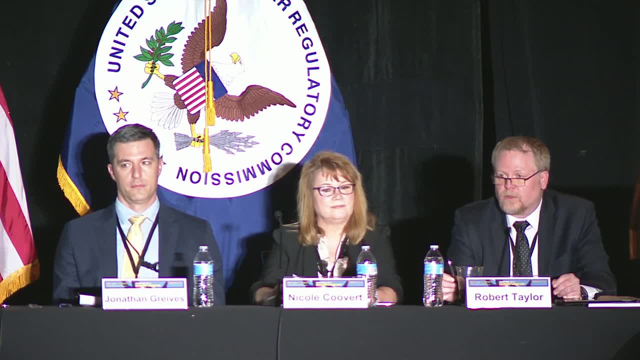 of these designs And I'd ask what inspections are truly necessary for us to implement and ensure that the plants are constructed as designed. As you'll hear from the panelists, we issued a commission paper in June of last year to share our vision for construction oversight for advanced reactors, including the seven key principles that are vital to the effective design and implementation of such a program. We're committed to hearing a variety of stakeholder inputs to ensure the program is designed consistent with these principles. 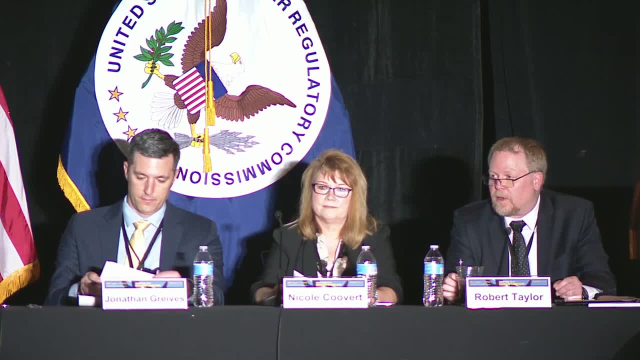 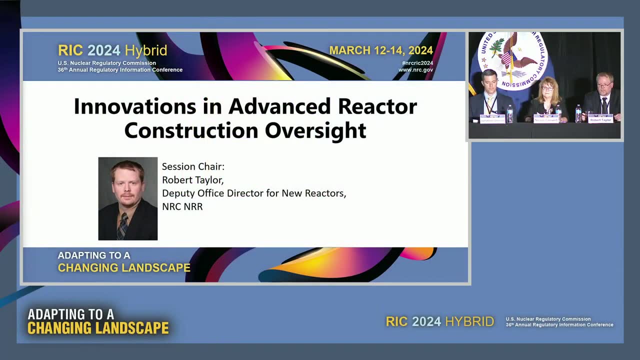 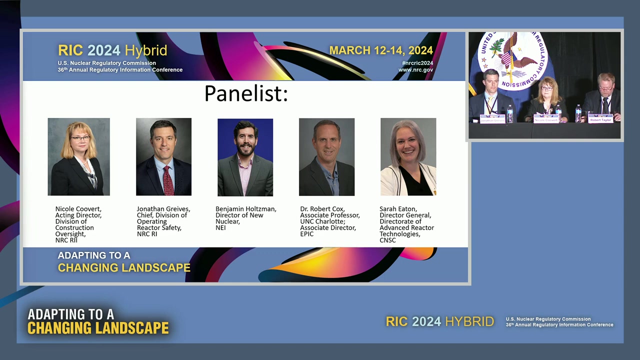 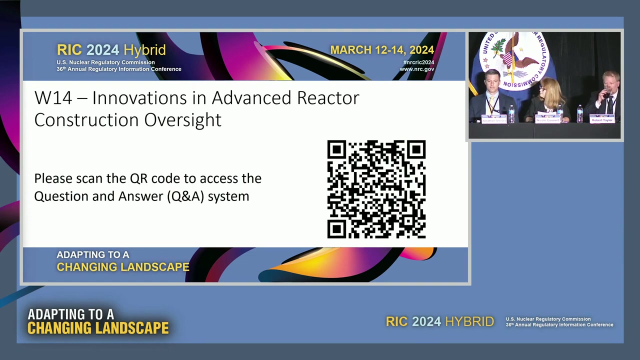 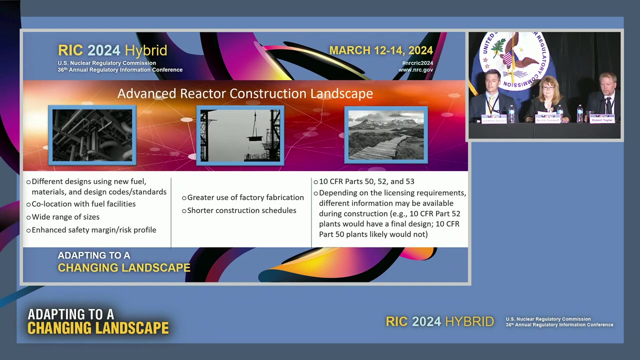 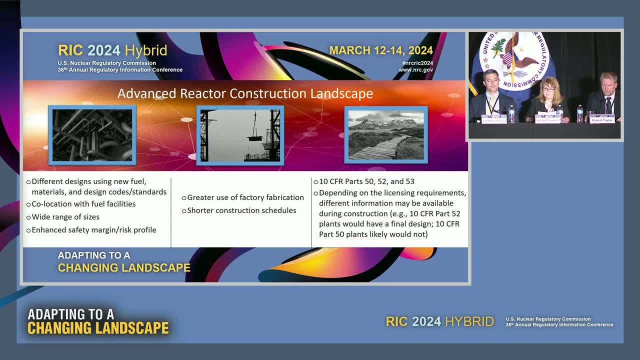 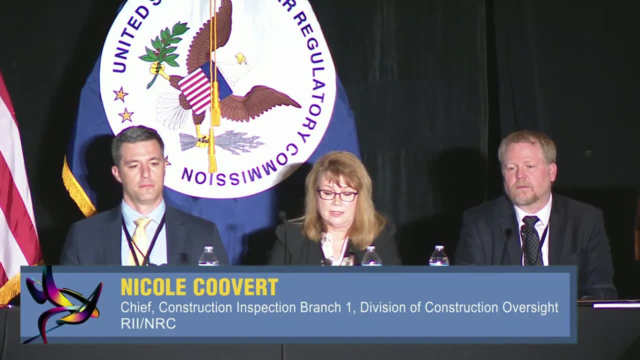 This diversity includes different reactor and containment designs that may be entirely new designs or may have had limited or no prior commercial applications in the United States. I would like to provide a disclaimer that the potential designs that I will discuss have not been licensed and or these designs may be. 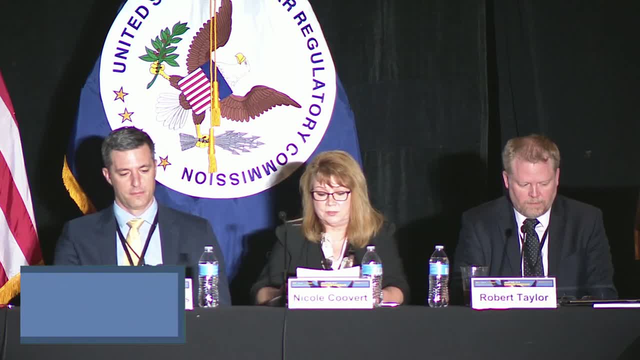 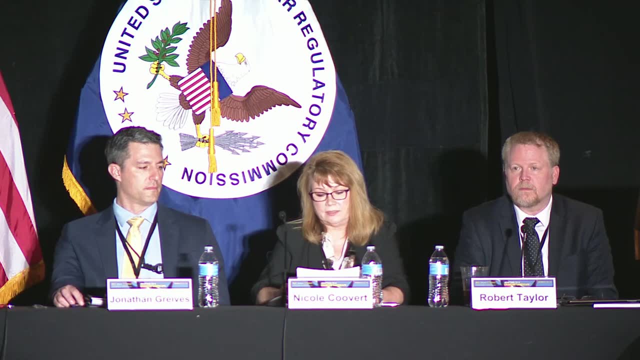 And some cases conceptual, and are subject to change, But for the purposes of this discussion, it's important to highlight the diversity that is on the horizon, And how does the agency consider this input when developing and implementing construction oversight framework? Advanced reactors can be small module reactors, micro reactors, and include light water and non-light water designs. 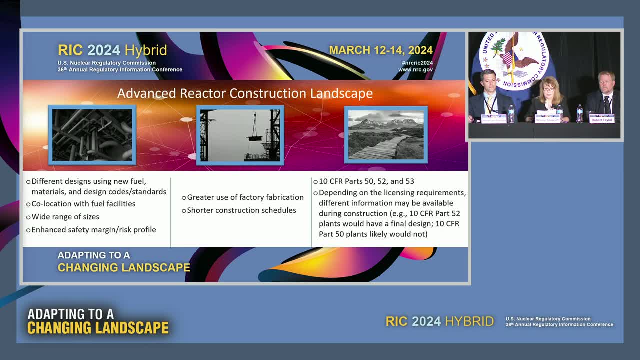 But in general, these designs are anticipated to be simpler, with enhanced safety margin and risk profile, And, as a result, they are not advanced. As a result, require less safety-related structures, systems or components or SSCs and, as applicable, 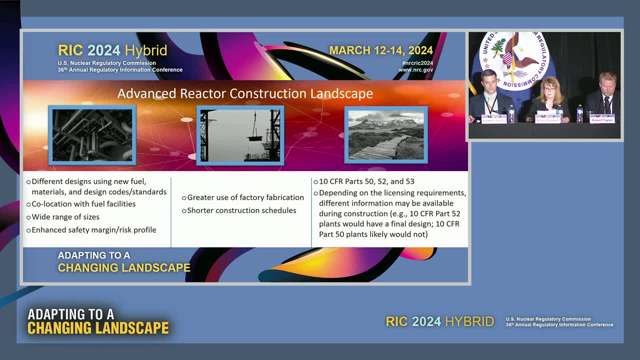 less ITAC, which is inspections, tests, analysis and acceptance criteria, compared with the traditional large light water reactors built in the US in the past. Additionally, some general design criteria, which is listed in Appendix A of 10 CFR Part. 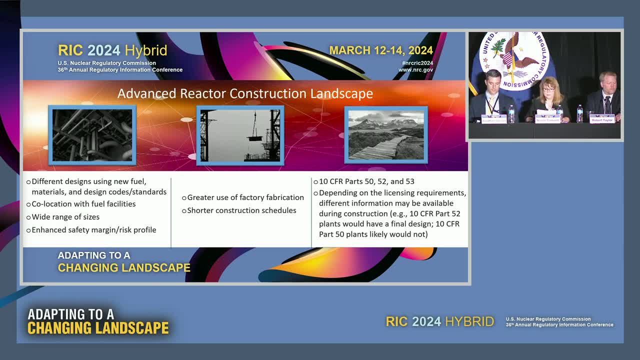 50, may not be applicable based upon the proposed licensing and design basis. For example, a reactor and coolant system may be designed such that a potential accident scenario is not credible. One proposed design may not need to consider a loss of coolant accident as a credible event. 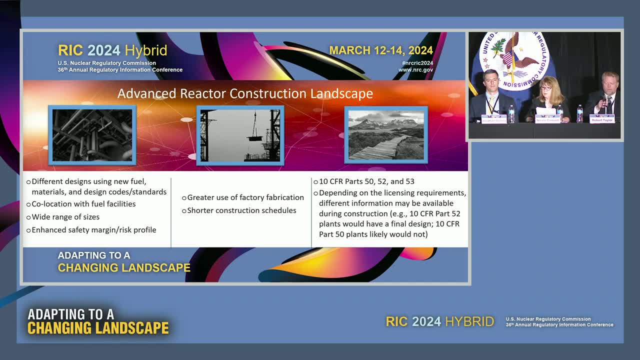 or may not need a containment structure for the purpose of containing fission products. Proposed advanced reactor designs may have minimal or not required active safety systems, have minimal or no safety-related electrical systems, or have minimum or no operator actions needed. These designs are needed to mitigate the consequences for an event while still ensuring. 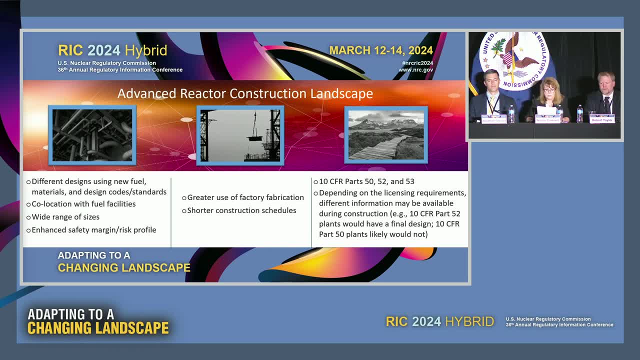 reactor core safety and public health and safety. For example, one passive design feature uses natural circulation with no electrical power or active pumps, and provides decay heat removal during normal operations and post-accident response. These potential designs also foster new reactor fuel types to be used in commercial plants. 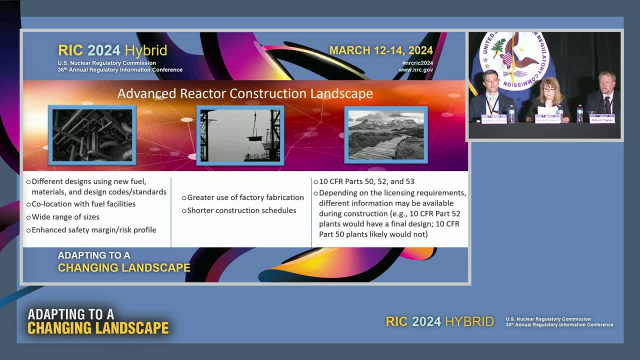 in the US, like triso fuel pellets and molten chloride salt filters. In addition to the standard light-water reactor fuel standard, industry construction codes may also be different. Additionally proposed designs may introduce new initiating events or material interactions, like interactions with sodium and water steam or air interactions that may result in unintended 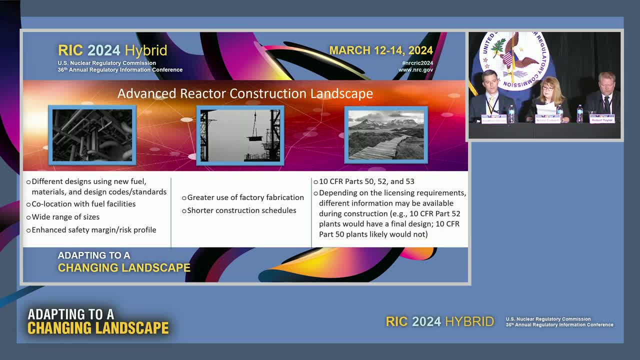 reactions. All of these examples might be considered as new inspection actions. The construction of advanced reactors may include new construction attributes to incorporate into construction inspection programs. Other items to consider for oversight framework include wide range of sizes and locations for nuclear reactor sites, including co-location with fuel facilities. 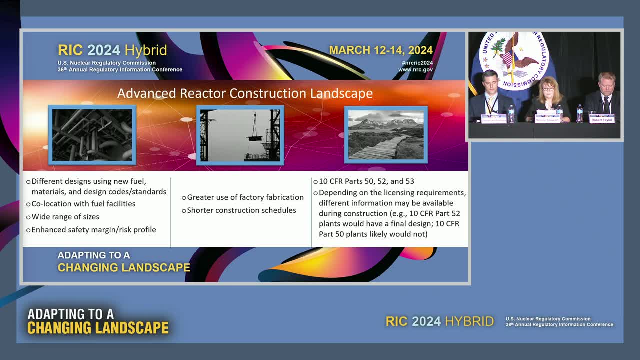 The construction of advanced reactors may include higher uses of modularization, including greater uses of system installation and testing off-site locations, like manufacturers. However, the expansion of the reactor may also include further progress in the manufacturing process. Next slide, Slide 4.. 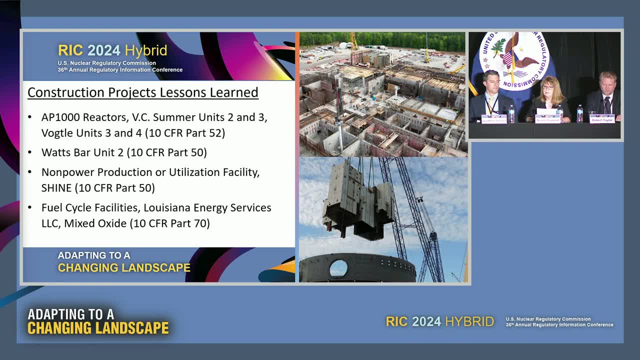 Slide 4.. In addition to design and associated margin and risk profiles, it is important to consider previous construction projects, lessons learned and best practices. Some of the oversight framework that the NRC has utilized since 2010 are for the AP1000s reactors, licensed under Part 52, Watts Bar Unit 2 construction under Part 50, licensing non-power production and utilization facilities or NPUFs for shine, also under Part 50, and fuel cycle facilities under Part 70.. 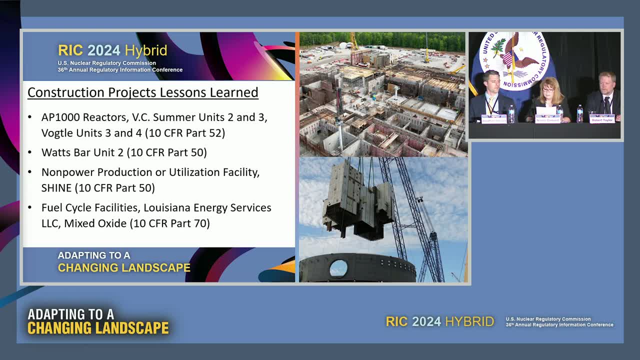 The NRC construction inspection staff that conducted these inspections for fuel facilities, NRC construction facilities, NPUFs and reactor construction projects are working together with the program offices to identify the best practices across the different NRC business lines to develop consistent inspection guidance. 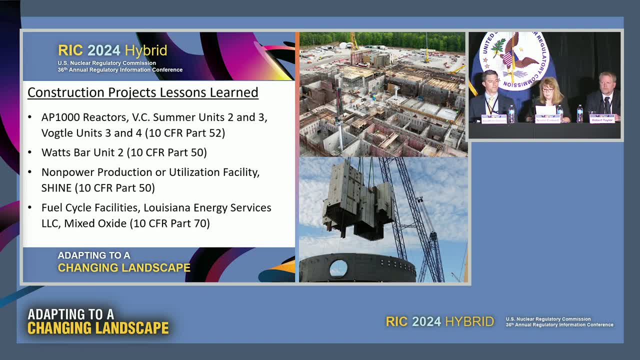 And by taking this approach, lessons learned and best practices are leveraged across the different areas, which results in more efficient and effective oversight programs that also benefit in cost savings across the agency, the industry and the US taxpayers. Next slide, please. 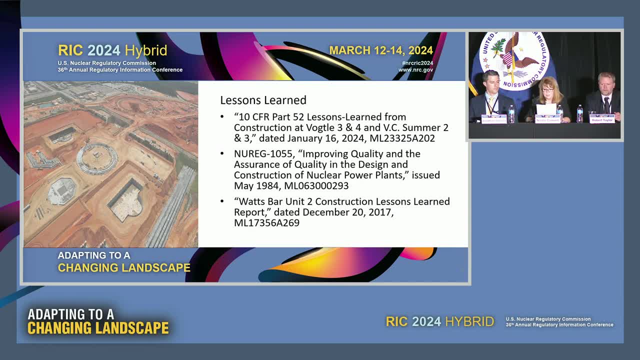 The staff is considering construction recommendations from both external and internal lessons learned. For external lessons learned, the NRC is collaboratively working with international regulators, along with reviewing lessons learned from international projects, industry working groups and industry stakeholders where appropriate and applicable. 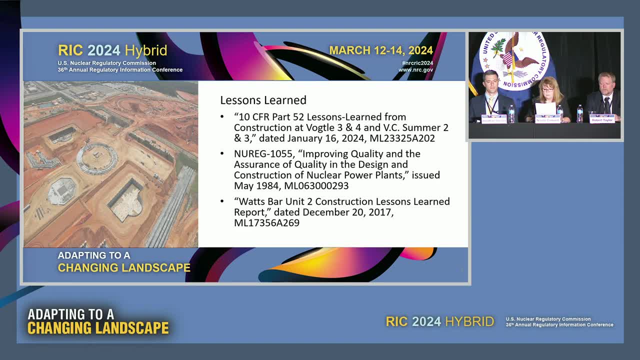 The staff also leveraged internal lessons learned, reports And through some technical support. they 사람 falachmalbour exhibiting months of research and development by behalf of NRC. The NRC's development authority was capable of hoping to improve energy efficiency in the energy sector acquired by this opportunity, but its powers were limited to Japan and other countries. 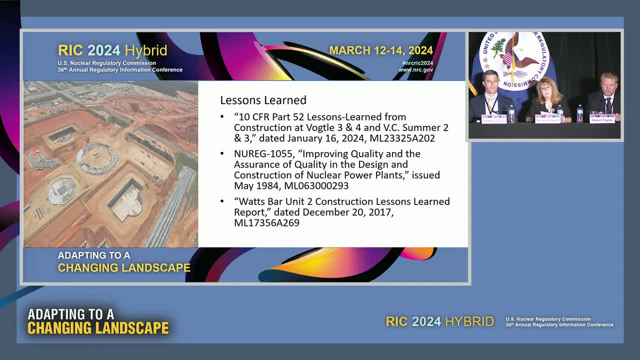 Thank you, Thank you. Thank you for the first-of-a-kind AP1000 plants in the United States. The NRC's process for targeting ITAC and the programmatic requirements for their inspections were found to be too prescriptive and did not provide for a flexible or user-friendly means. 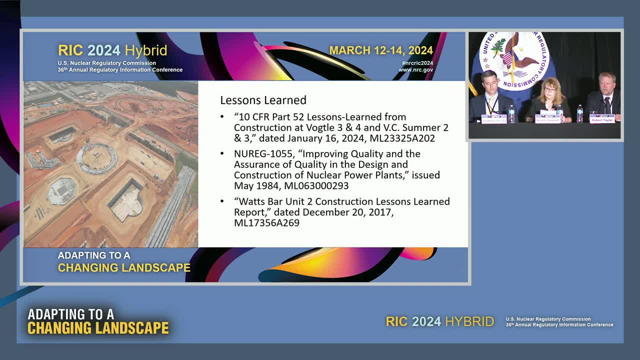 to adjust when plant inspections could not be performed due to the changing construction schedules. The working group recommended for future oversight programs there should be a flexibility to select a representative sample of inspections throughout any construction area and not require pre-selected ITACs to make up the baseline inspections. 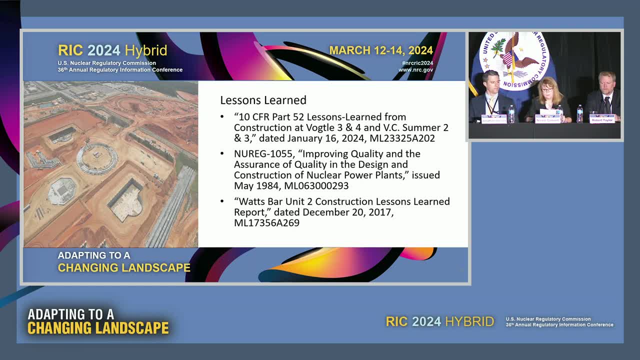 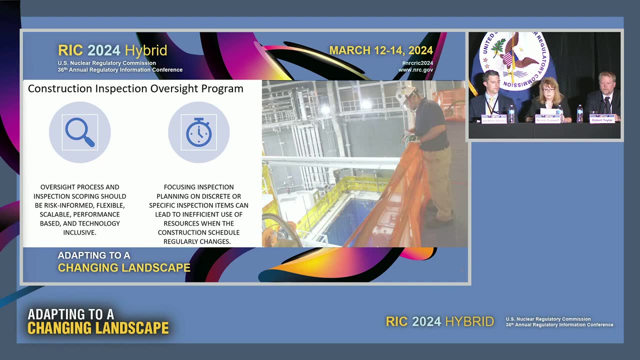 This would promote more agile inspection coverage, while continuing to maintain reasonable assurance that facilities are built and will operate in accordance with their approved designs and licensing basis. Next slide, please. The NRC is taking a holistic approach to the revisions and the development of the NRC. 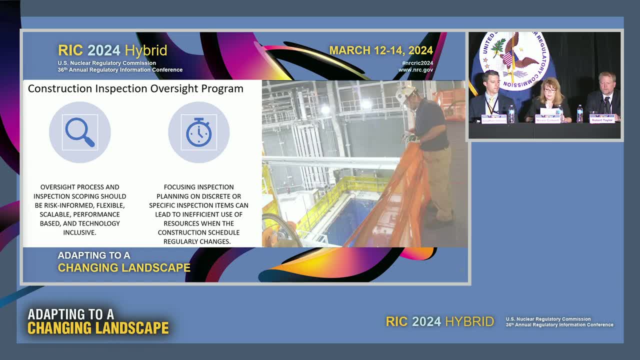 The NRC is taking a holistic approach to the development of the construction oversight framework Where, in the past, inspection program guidance was written for the specific project occurring at the time, now staff is intentionally considering future oversight processes and inspection scoping that is risk-informed, scalable, performance-based and technology-neutral. 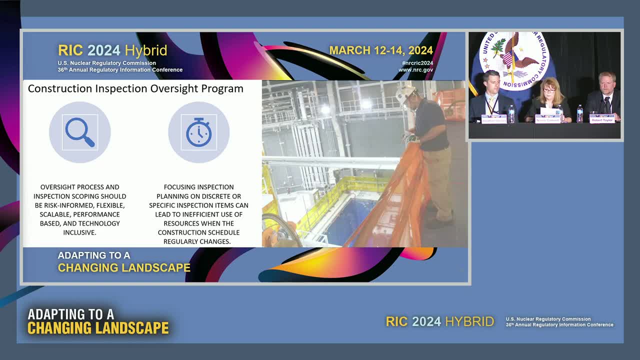 that can accommodate different types and sizes of projects. Additionally, future oversight processes and inspection scoping needs to be flexible, without focusing on inspection planning on discrete or specific items. that can lead to inefficient uses of resources, especially with changing construction schedules. Next slide, please. 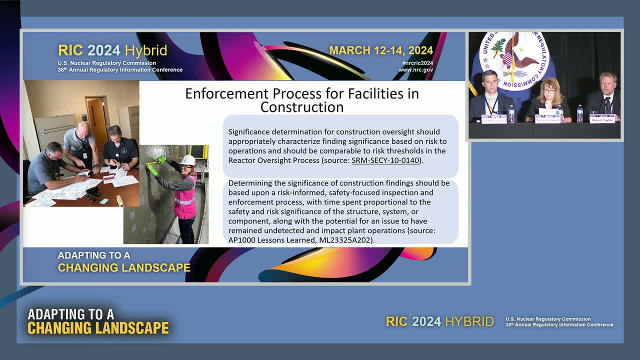 In addition to inspection, oversight framework includes enforcement and assessment. Lessons learned for the enforcement process for facilities and construction are first, significant determination should appropriately characterize findings significance based upon risk to future operations and should be comparable to risk thresholds in the reactor oversight process or ROP. 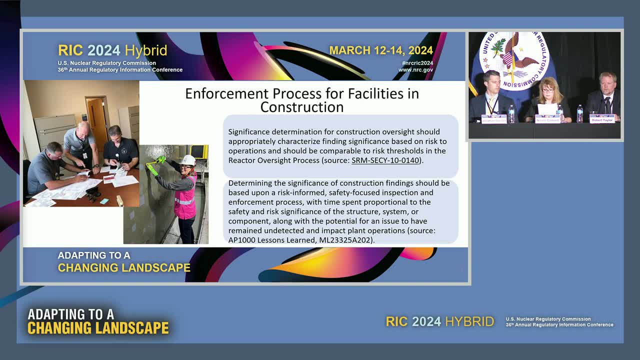 Second, determining the significance of construction findings should be based upon a risk-informed, safety-focused inspection and enforcement process, with time spent proportional to the safety and risk significance of the SSC, along with the potential for an issue to have remained undetected and impact plant operations. 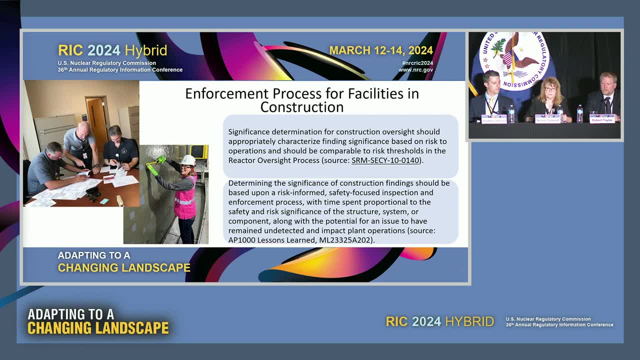 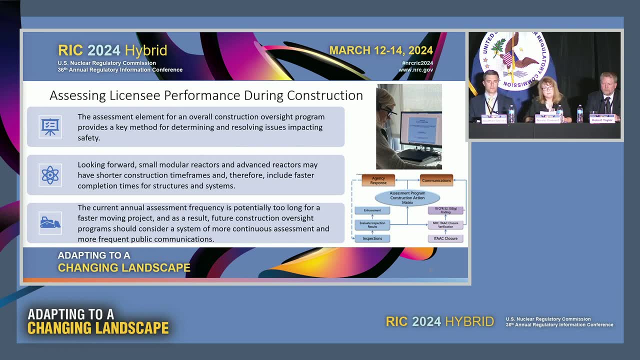 Next slide, please Last. the assessment element for an overall construction oversight program provides a key method for determining and resolving issues impacting safety. Looking forward, advanced reactors may have shorter construction timeframes and therefore include faster completion times for structures and systems. The current annual assessment frequency in the CROP was based upon an annual assessment. 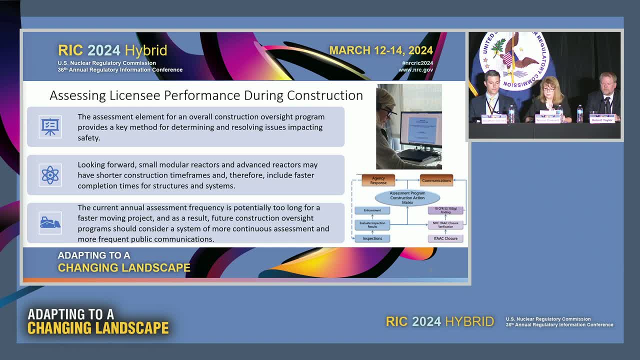 period. Unlike the ROP for operating reactors with consistent annual baseline inspections, facilities under construction have dynamic schedules and performance. From one year to another, the amount and type of work, including different contractors and vendors involved, will differ, So one year's performance comparison to another is not always equal. 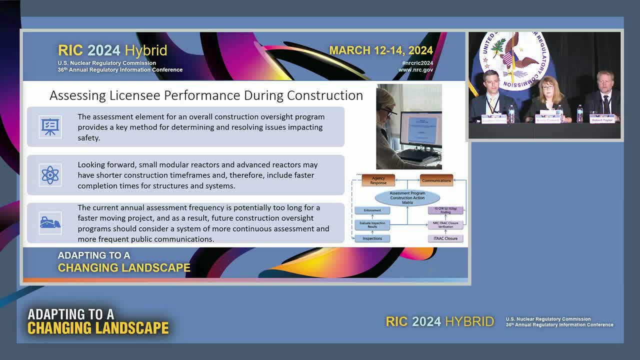 Additionally, assessment periods may potentially be too long for a faster moving project. As a result, future construction oversight is not always the same. As a result, future construction oversight programs should consider a system of more continuous assessment and more frequent public communications. I will turn it over to John Greaves to discuss aspects and considerations for the future construction. 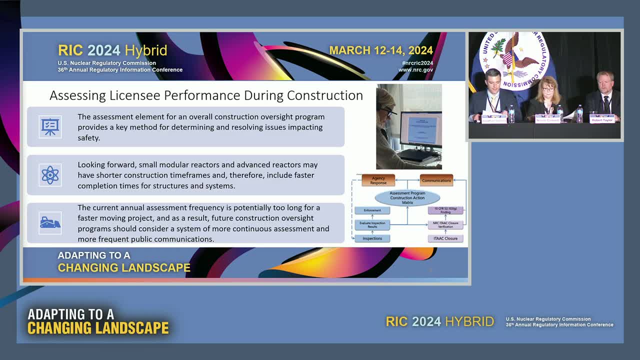 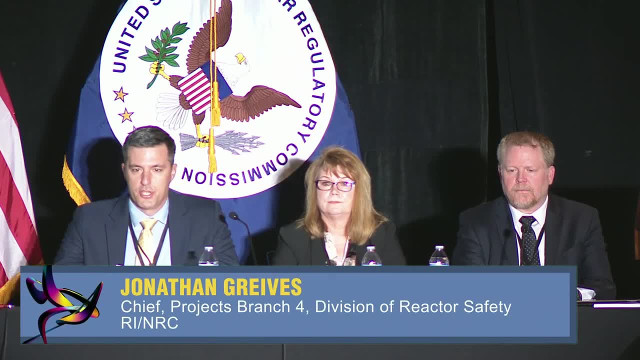 oversight process for advanced reactors. Thank you, Thanks, Nicole. Next slide, please. The objectives of the construction oversight program remain unchanged in that it supports the NRC mission by providing independent verification that facilities are verified and that the built and will continue and will operate in accordance with their approved licensing basis. 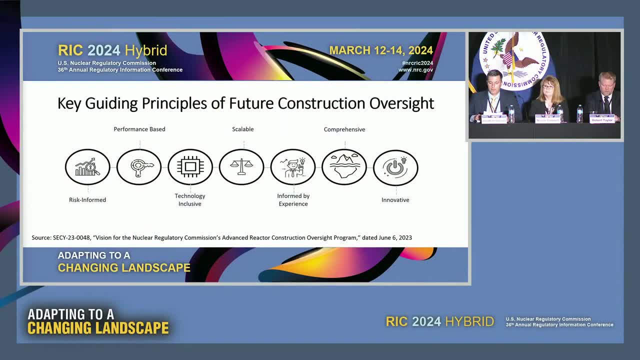 To do this? oversight for advanced reactor construction focuses on the verification of the quality of those SSCs that are integral to the safe operation of the facility and verification that security and other operational programs are in place to support operations. Said another way, the construction oversight program supports the NRC's licensing decision. 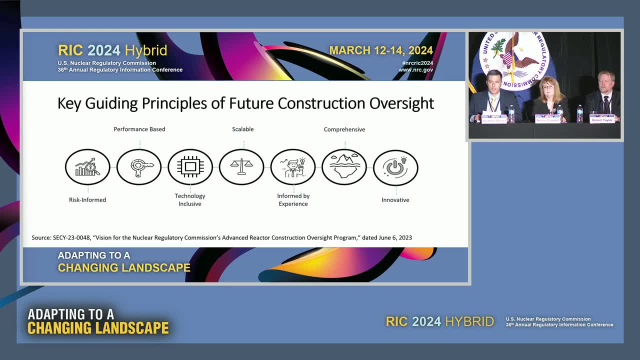 to allow operation of the facility through either issuance of an operating license for Part 50 applicants or 103G finding for Part 52 applicants, by providing an independent verification through a risk-informed performance-based sampling program To meet the objectives of the construction program. in June of last year, we documented 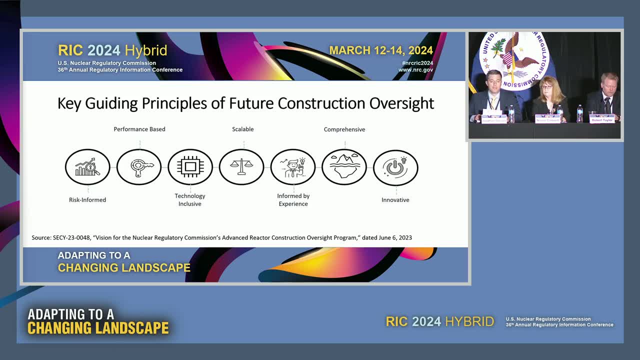 seven key principles that are key to development of the oversight program. We documented that in SECI 230048.. Of those principles, risk-informed and performance-based- remain pillars to any oversight program and will guide us to ensure that we focus on the most risk-significant aspects of design and that we consider the observation and review. 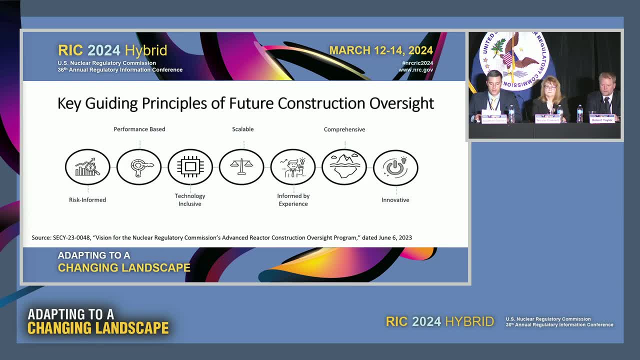 of infield performance in addition to paperwork reviews when appropriate and possible, and that we use our assessment process to adjust our oversight. footprint Technology inclusive refers to ensuring that the program covers the full spectrum of reactor technologies that Nicole described earlier that are being considered for NRC licensing. 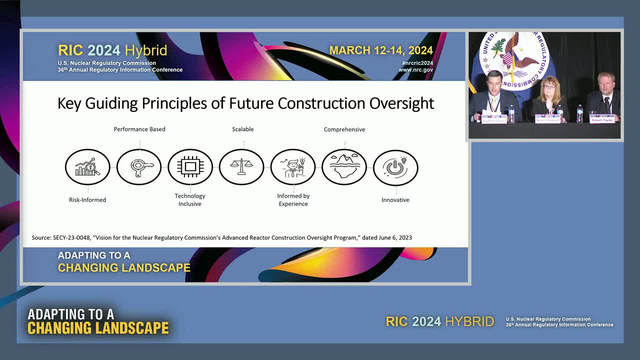 Scalability is important because it ensures our inspection efforts remain commensurate with the facility's public health and safety risks, Informed by experience, such that it implies the construction oversight experience and leverages lessons learned from past and current NRC inspection programs and other external 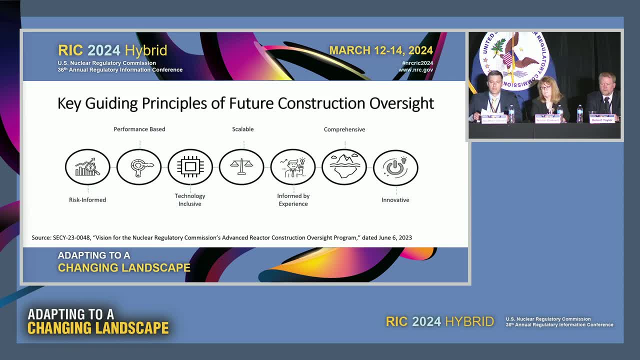 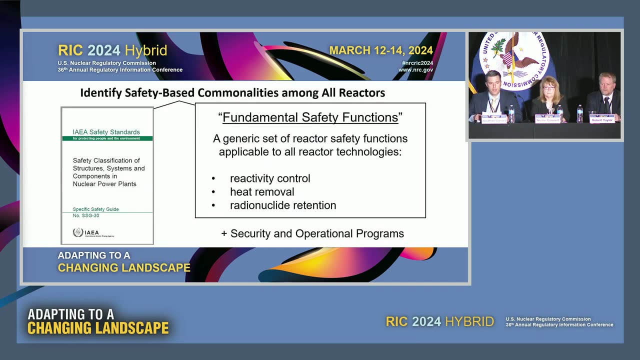 sources. Comprehensive in that the program is designed to consider all possible manufacturing models and diverse licensing approaches. And, lastly, innovative in that it leverages new inspection tools and approaches to enhance efficiency and effectiveness whenever possible. Next slide, please, To construct a technology-inclusive program that can be used to address the needs of the 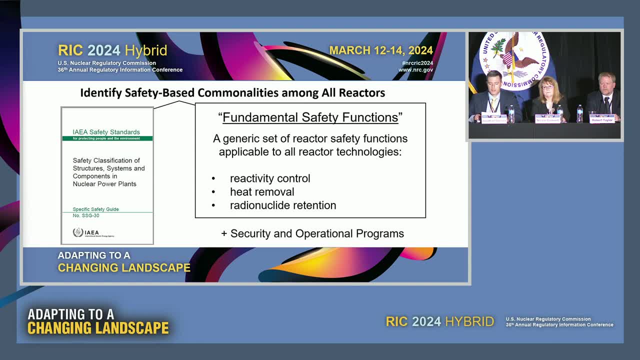 entire facility To develop inspection plans and assess construction performance for all new designs. we started by looking for safety-based commonalities across all reactors. While each designer will develop their own methodology for SSC classification in accordance with standards and guidance applicable to their design, we found that orienting the 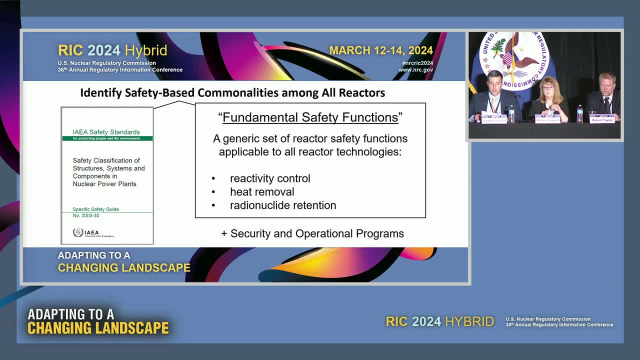 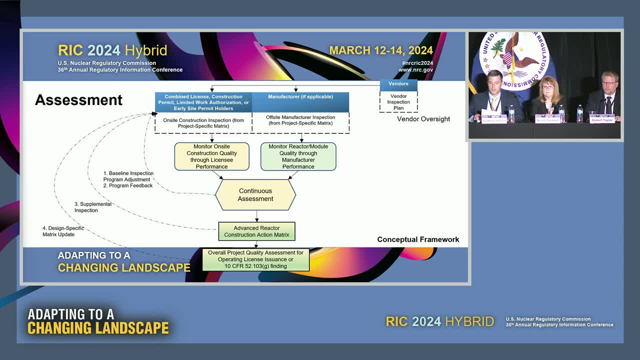 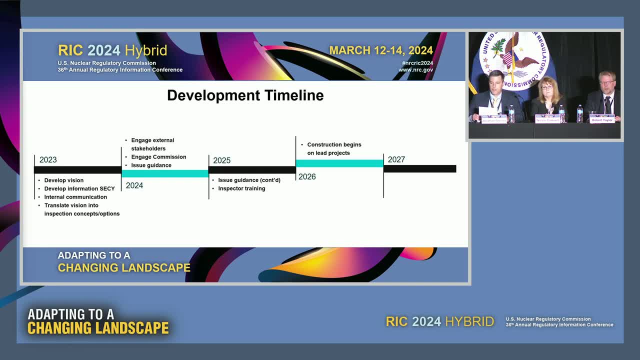 and intend to leverage that feedback to build the best program possible. We are committed to keeping all stakeholders informed of our progress, including the Commission, and will engage on potential policy issues early to provide clarity. 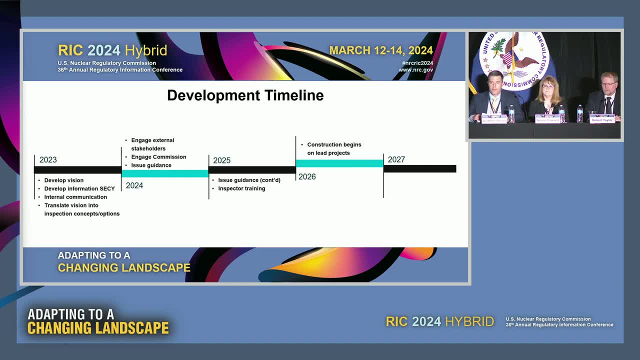 While we recognize the need for a working program in time for these early projects, we also acknowledge that the program will continue to evolve in the future as new technologies are introduced, both for licensees and manufacturers, as well as for inspectors and experiences gained during construction of earlier builds, and we remain committed to the evolution of 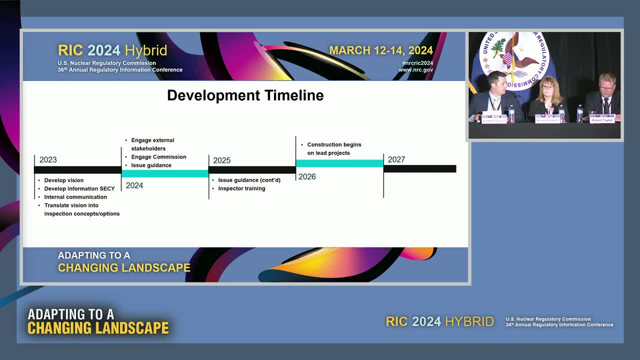 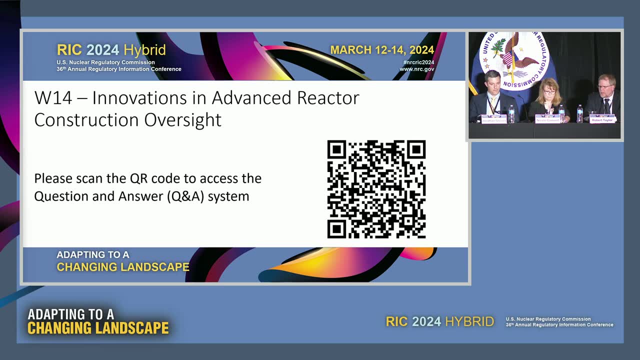 the program into the future. Thank you for your time and I'll turn it back over to Rob. Thanks, Nicole and John Appreciate that overview of what the NRC is currently thinking and, as you indicated, we're early in the process and now is the opportunity for stakeholders to really engage. 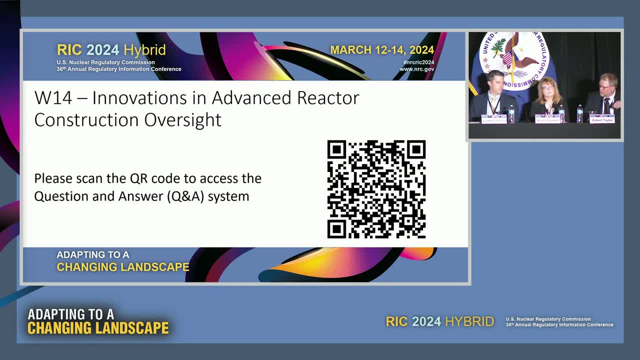 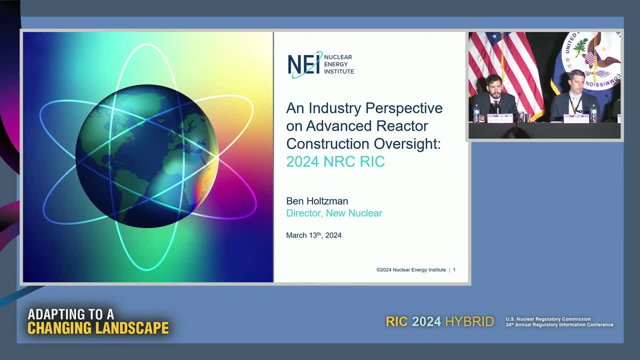 us and help us shape the program as we go forward. So, with that in mind, it's my pleasure to introduce Ben Holtzman, who is the Director of New Nuclear at the Nuclear Energy Institute. He is currently focused on developing a more efficient risk-informed range. 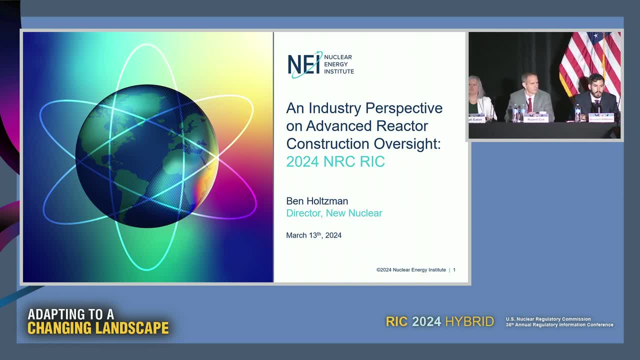 He's also working on developing a more efficient regulatory framework, accelerating industry deployment readiness and engaging with investors and new end users to understand new nuclear opportunities. Ben, please, Thank you. Thank you Good afternoon. I'm Ben Holtzman, Director of New Nuclear at NEI. 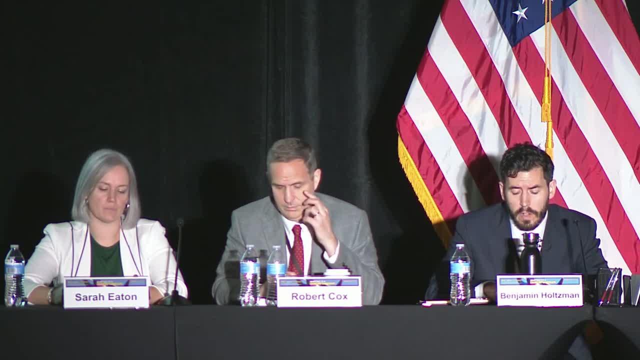 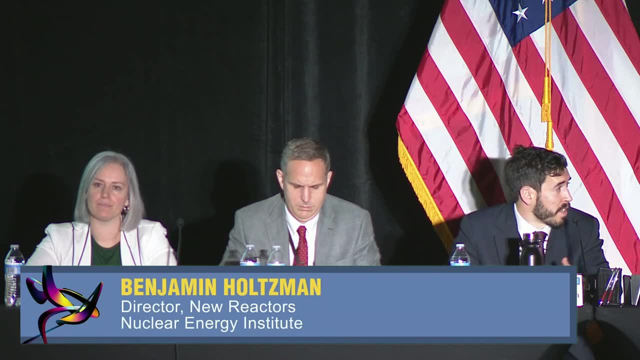 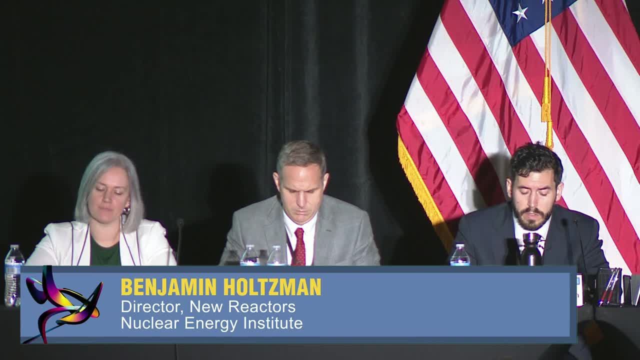 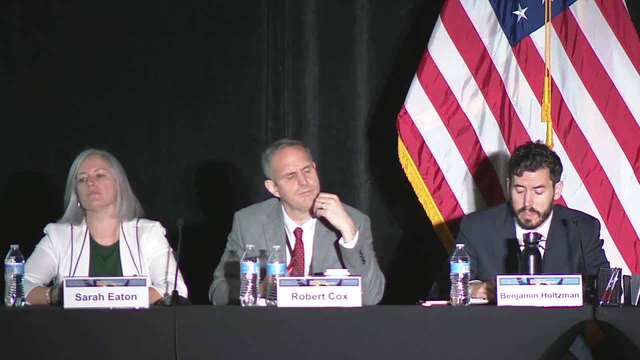 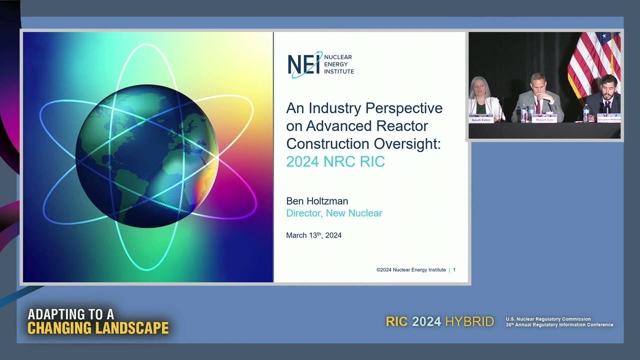 It's an important function that is needed to ensure new reactors are constructed in accordance with their approved design and licensing basis, thereby providing reasonable assurance of their safe operation once completed. As part of this presentation, I will impress why developing a more efficient construction oversight process is important for both the NRC and industry, as well as highlight a few. 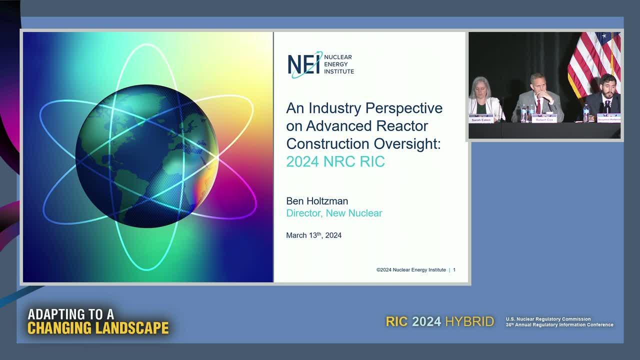 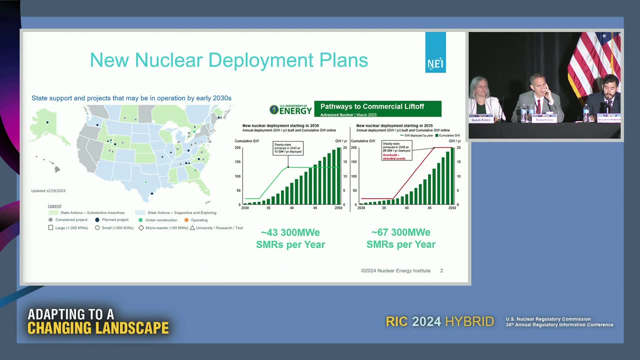 key considerations that we believe should be in a successful program. Next slide, please. As seen on this North American deployment map, there are over 25 nuclear power projects in development today. Vogel Units 3 and 4 are leading the way for new nuclear 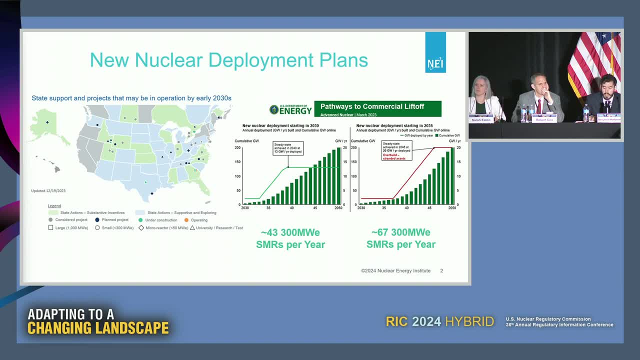 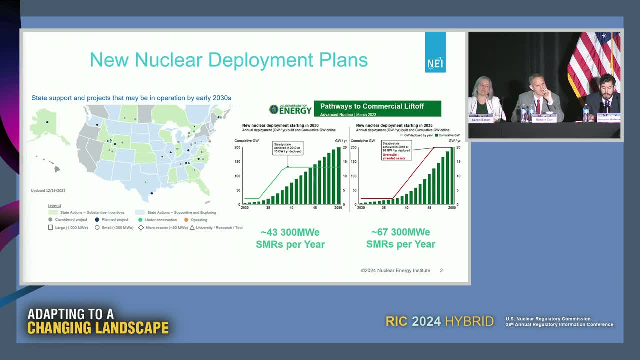 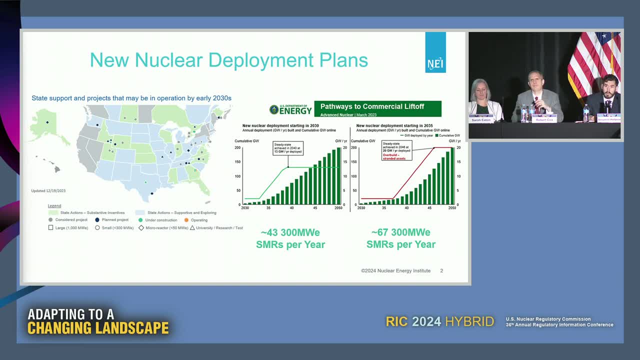 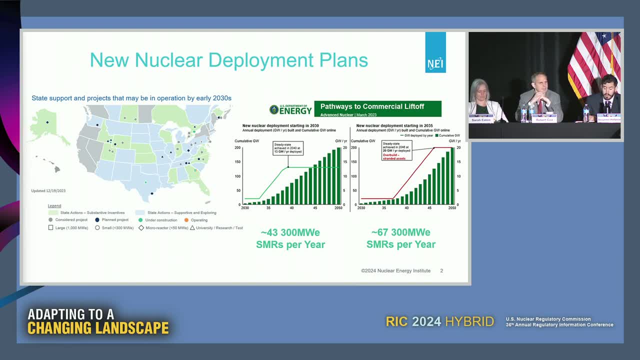 The second figure shows new nuclear deployment starting in 2035 at a rate of 20 gigawatts per year, corresponding to about 67 300-megawatt electric SMRs coming online. This would mean over 100 SMRs are in construction at any given moment, since it takes more than a single year. 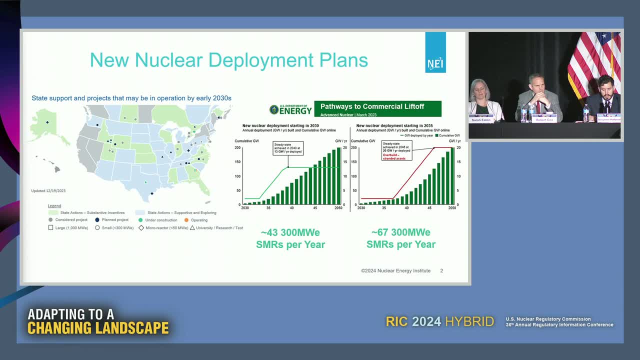 to construct a new plant. If we think that some of this new nuclear growth will be micro-reactors, then there's even more reactors per year And, of course, if we think some of them are large lightwaters or larger reactors in general, then there's fewer. I don't want to focus on the 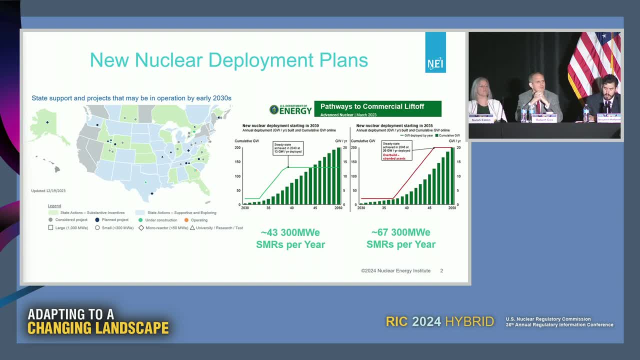 specific number of new reactors per year, for two reasons: First, because all models are wrong, although some are useful, And second, while we may not know the exact number of new nuclear plants per year, we're looking at a lot. We're looking at a lot of new nuclear, not one or two. It's no longer a matter of whether to build. 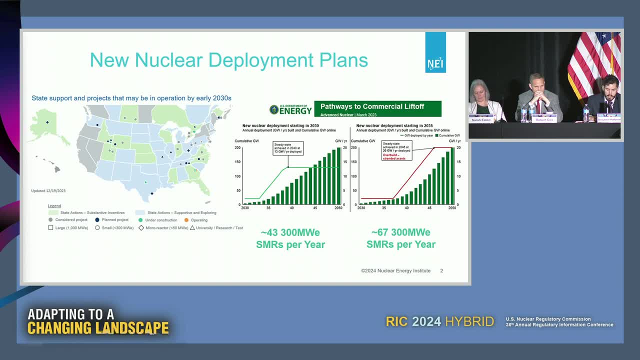 these versatile, reliable and clean reactors. It's a matter of how fast we can build them. Of course, the future is a big place. Anything can happen. In 2008,, no one saw the price of natural gas falling from $10 to $3 due to fracking, But there's a real opportunity here, if we can. 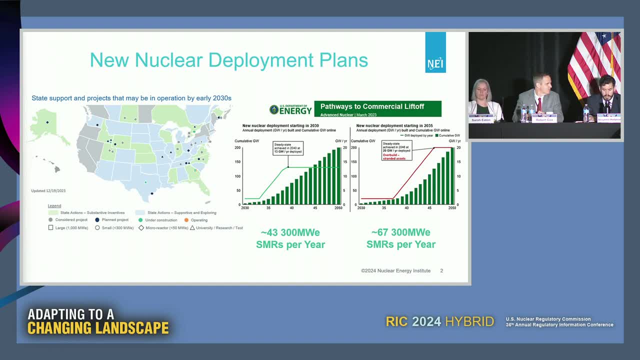 seize it, And part of how we can do just that is by rethinking construction oversight, Because if we do things as we've always done, we would need an unreasonable number of workforce for both the industry and NRC As such. let's talk about how to do things more efficiently. 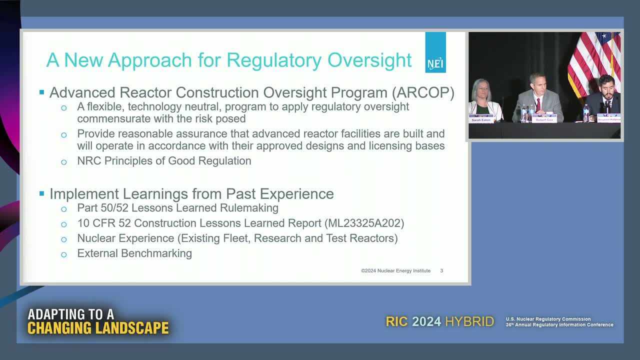 Next slide, please. The NRC also realizes that the status quo is not scalable. to support the deployment of hundreds of reactors, Risk-informed thinking is required. As such, the NRC developed R-COP to support the realization of large-scale deployment of nuclear reactors. 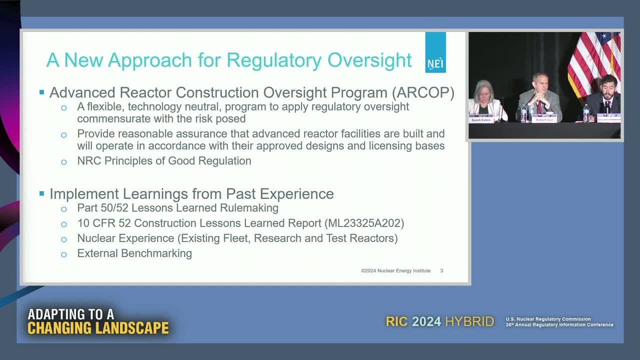 And part of how we can do just that is by rethinking construction oversight, Because, if we do things as we've heard, new nuclear is a diverse set of technologies which requires the oversight program to assess the relative risk in a technology-neutral manner. Furthermore, R-COP should incorporate the lessons from 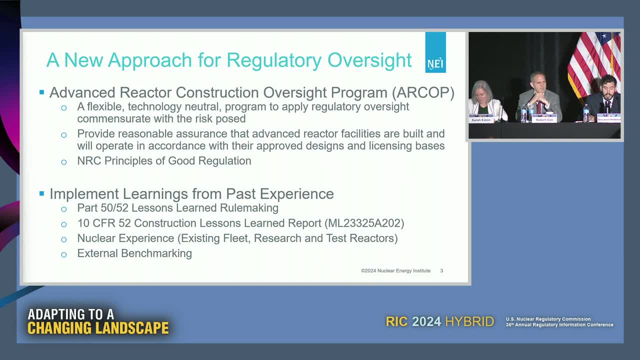 construction experience, both domestically and internationally. Applicable lessons can be gleamed from the existing fleet, research and test reactors, the AP1000 experience and even international projects such as Baraka New nuclear designs come in a variety of shapes and sizes, and the best practices from one experience 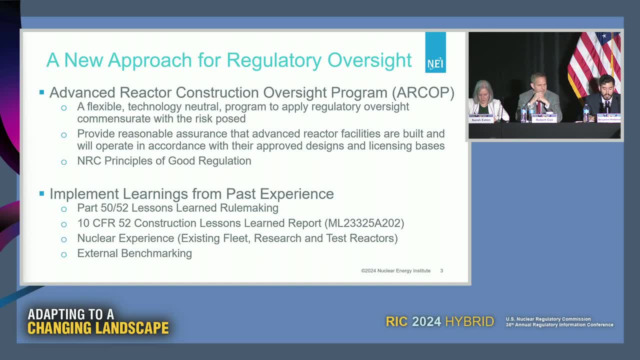 may or may not be applicable to a specific new design project. For example, non-LWR micro-reactors may be much closer to a research and test reactor than a large light-water reactor And, as the Commission noted yesterday, the hours spent on oversight should reflect the safety significance. 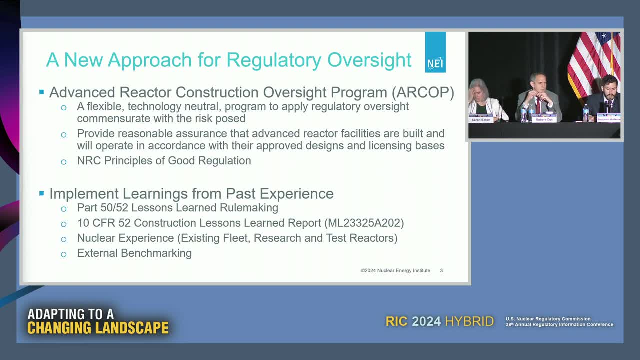 and risk associated with the activity. Some of these best practices and lessons learned are already being documented in the NRC's research and test reactor, and the NRC's research and test reactor is being documented, but will still need to be incorporated into the R-COP program The most recent. 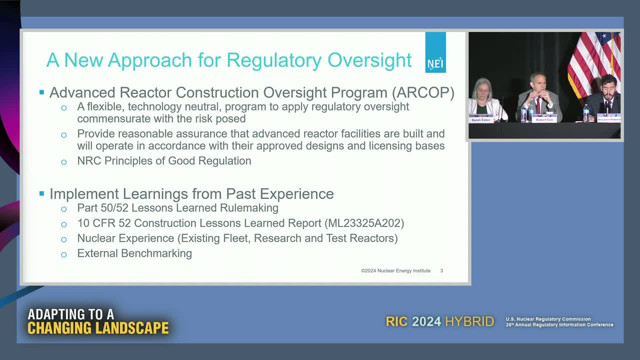 construction: lessons learned report came out this January. It discusses the lessons learned from the Part 52 construction for Vogel and Vesey summer projects, focusing on potential improvements for the oversight of future construction projects using the same Part 52 licensing framework As it's already. 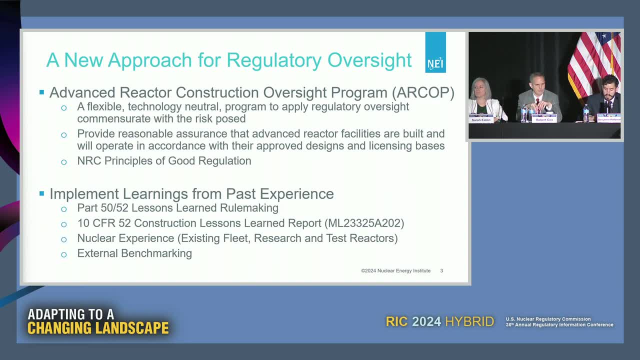 been discussed more specifically of what this covers. it highlights again ITACs and licensing activities during construction. Additionally, NRC has the opportunity to improve the construction regulatory process by incorporating improvements as identified during the 5052 lessons learned rulemaking activity. These changes can also improve regulatory efficiency during construction and play an important role in 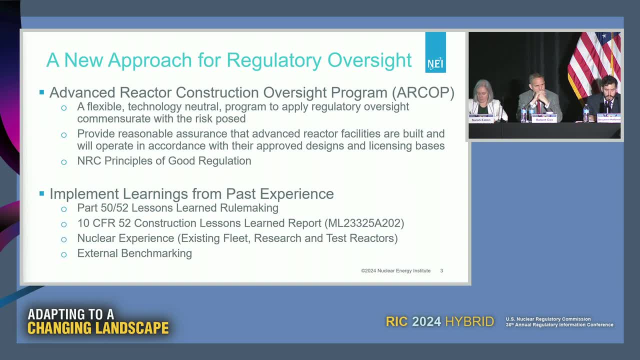 enabling widespread deployment of new nuclear. It's important that the risk-informed R-COP program work through and articulate how oversight would actually change between different deployment scenarios. We encourage engagement and discussion with industry to ensure that the program is indeed scalable, technology neutral and comprehensive. There are many key questions that still need to be. 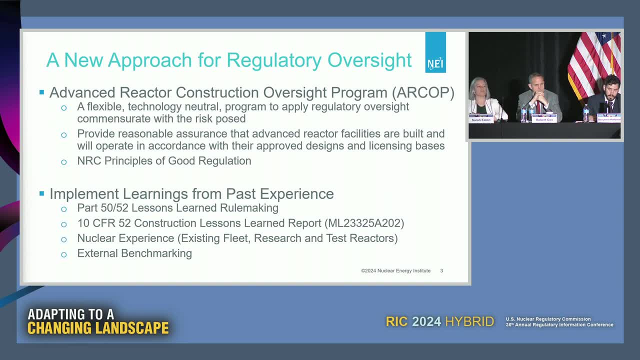 worked on? Where does enforcement and oversight get applied? How does offsite manufacturing and assembly interface with a facility's QA program? In the past, all construction activities were done onsite, so it was straightforward that the licensee was responsible, But it's less clear what happened. 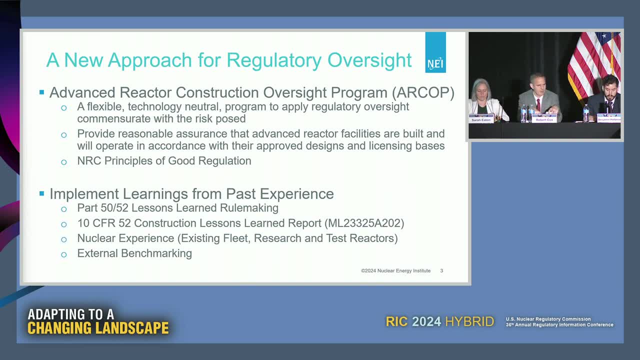 in the past. There may be a lack of compliance as work shifts to offsite locations, as parts modules and even reactors are completed in advance, potentially without even knowing their destination. Our takeaway message here is that a flexible strategy to right-size construction oversight would be a benefit to both industry and NRC. 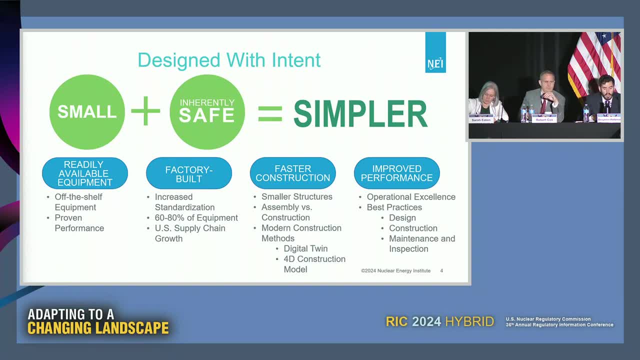 Next slide, please. I also want to highlight some of the things that industry is doing to ensure that we can deploy new nuclear reactors more efficiently. First, the NEI is establishing an advanced reactor oversight task force to act as a focal point for industry to engage with NRC on the development of advanced reactor oversight. 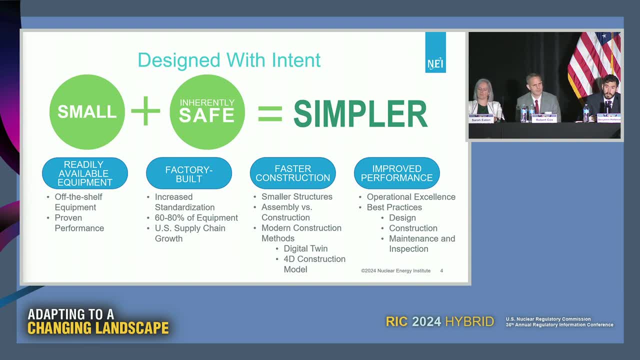 guidance. But success really starts from the beginning and new nuclear being designed with intent, by designing with construction, inspection and oversight in mind from the start. Industry is also learning from the past. These implemented best practices in design, construction, maintenance and inspection. 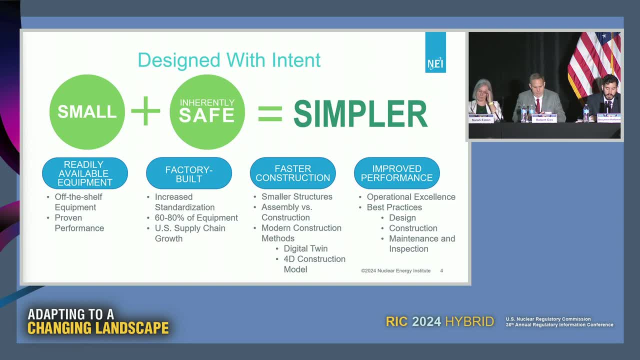 These best practices will help industry ensure that designs can be constructed and inspected faster, resulting in less upfront capital before revenue is realized. These include the NEI construction best practices documents, including our latest implementation guide, which was posted this week and discusses three primary topics. first of a kind, managing 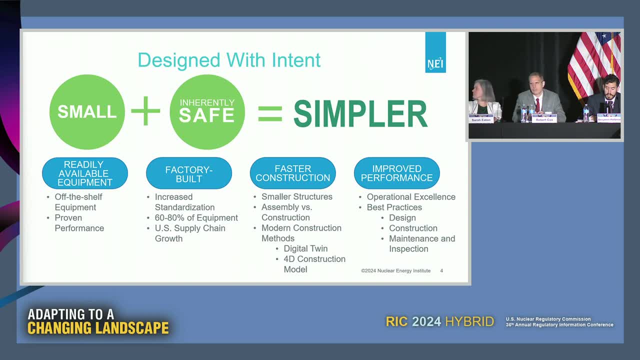 construction, labor efficiency and modularization. benefits and drawbacks. These documents will help industry deploy new nuclear projects safely, on time and on budget. But one of the first documented best practices is the importance of design maturity. The design isn't the largest cost component in new nuclear projects, but it casts the 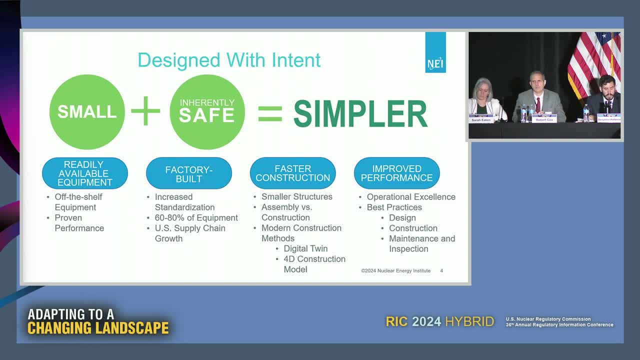 largest shadow in that, if the design needs to be redone, a lot of other downstream work also needs to be reworked. A detailed, completed design enables better projects to be built, And that's why we're here today. We're here to talk about project planning and execution, including using more detailed 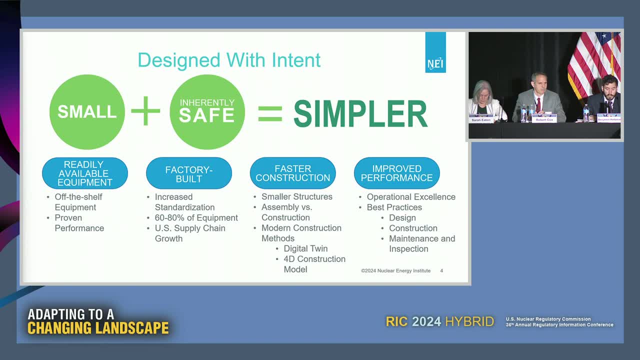 construction methods. Tools like Digital Twin and 4D construction models do require upfront capital investment, but will enable more efficient construction and inspections. Faster construction not only saves money, but it also helps resolve the Gordian knot of workforce, as faster construction means less plants in construction at any given moment. 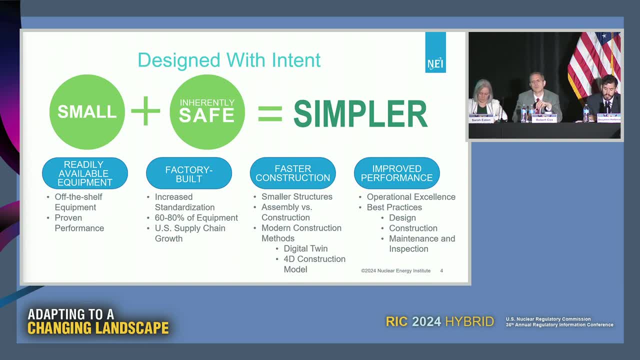 and therefore less workers. Similarly, shifting modules and manufacturing activities offsite will further reduce the onsite construction workforce requirements. Other best practices are more generally applicable. EPRI developed a report last November that provides information on maintenance and inspection that can provide insights not only for industry but also NRC, as it can help streamline pre. 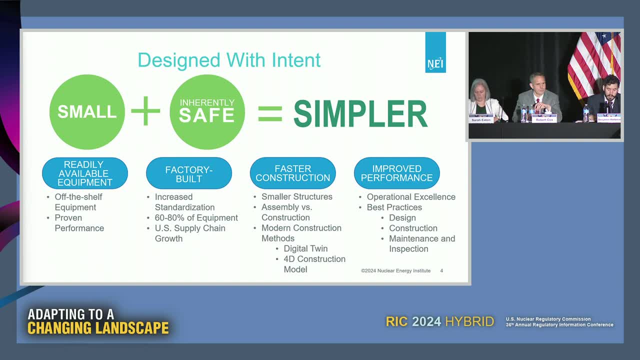 and service inspections and oversight. Another key aspect that will both increase the efficiency of both construction and oversight is increased standardization. We need to build airplanes, not airports. Standardization is not only building the same plants numerous times, enabling improved outcomes due to moving down the lessons learned learning curve, but it is also improved supply chain. 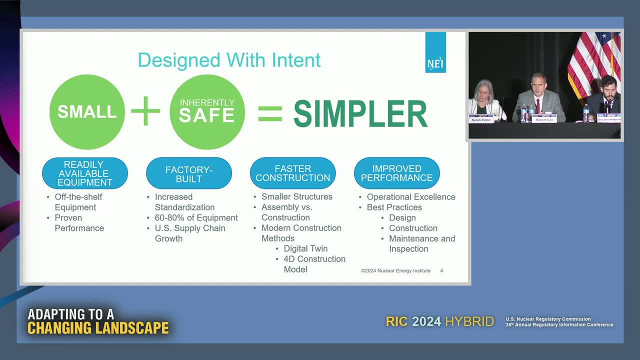 procurement by getting the same components. This results in easier inspection, not only because it is the same plant design but the same components that are in that design. So it is the same process as E3.. E3.. E3. E3.. 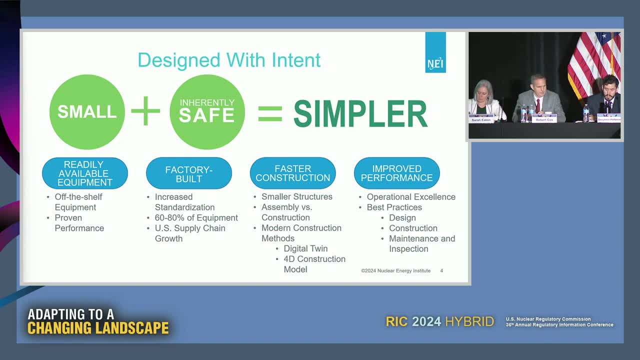 E3. As those plants go forward for inspection. This in turn helps standardize how RCOP is applied across multiple deployments of the same design. Through these efforts, industry and NRC can ensure this flexible program will yield regulatory predictability and certainty for oversight activities, while being grounded in safety. 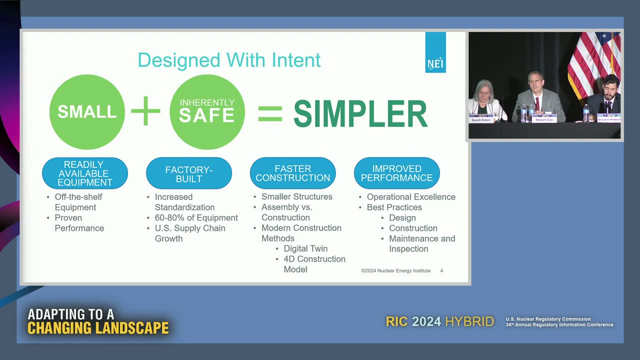 to reach a reasonable assurance that these designs will achieve safe operation once completed, Predictability and certainty being two key enablers for new nuclear to achieve economies of numbers and realizing the widespread deployment that so many models, industries and experts see in our future. 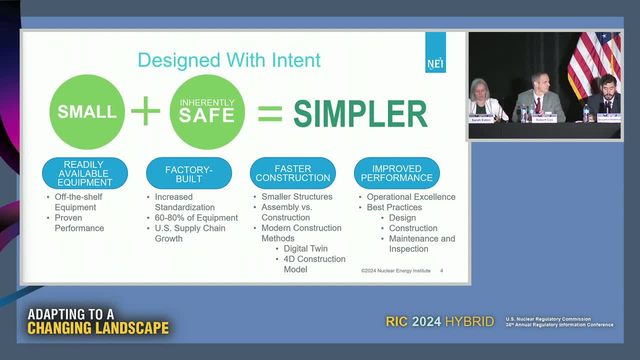 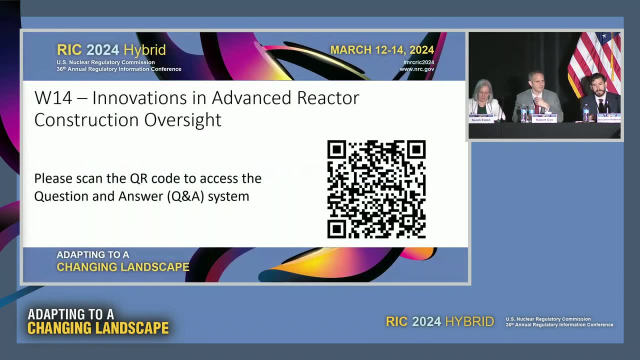 I never said it would be easy. I only said it would be worth it. Next slide, please. And with that, thank you, and I look forward to the rest of the discussion. Thanks, Ben, Really appreciate those perspectives and we look forward to the industry's insights. 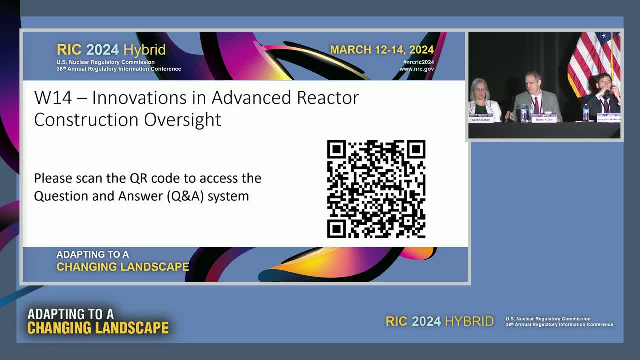 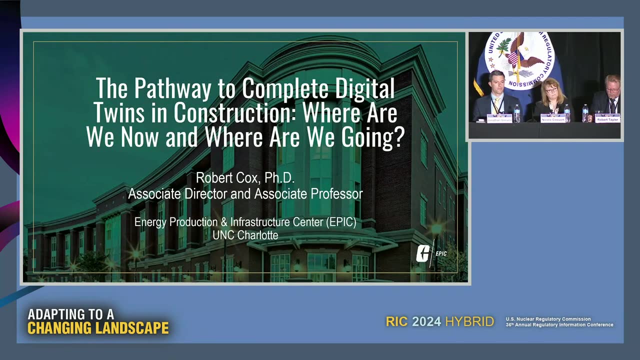 as we continue to build this and get into the specifics of some of the key elements and activities that you discussed. So we recognize the importance of looking at two different audiences for input and perspective, because we may not have all the right ideas within the traditional nuclear family. 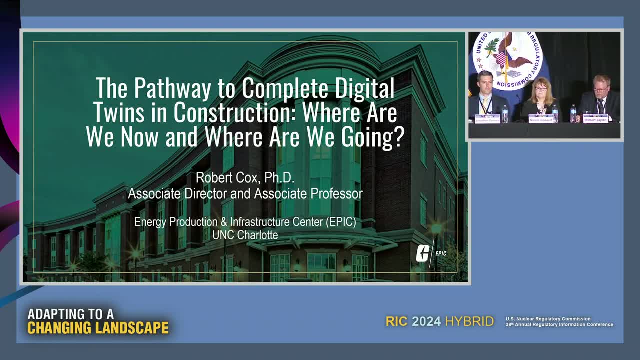 So with that, it's a pleasure to welcome Robert Cox to our panel. He's the associate professor of electrical and computer engineering at the University of North Carolina at Charlotte, where he also serves as the associate director of energy production and infrastructure center. He focuses his research on applying digital engineering to various problems. 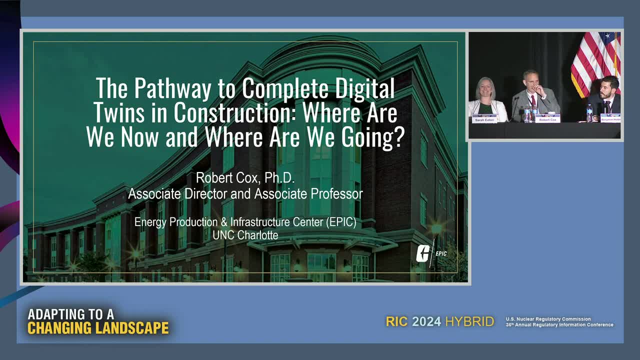 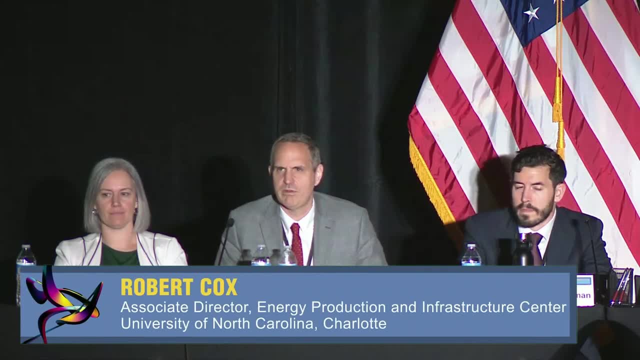 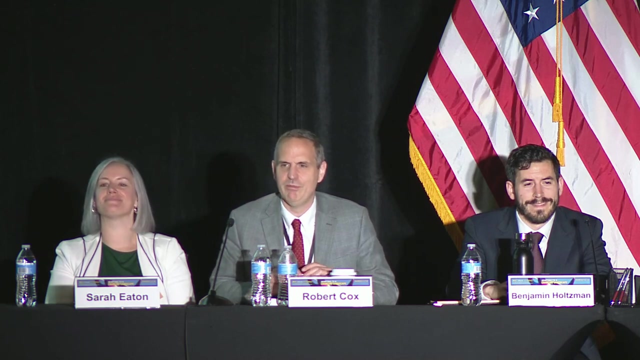 Robert, All right, Yeah, Thank you very much. Yeah, So a nontraditional contributor to this conference, but really welcome to be here. Next slide, please. So what I wanted to talk about here today is basically digital engineering. So Ben here spoke a little bit about building the airplane rather than the airport. 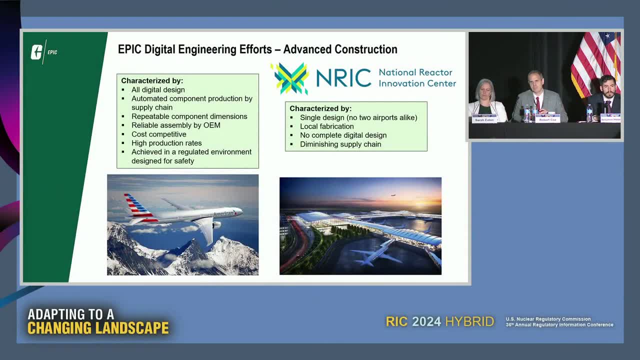 So, for context here, what we're talking about is applying digital techniques. Everybody talks about digital twins These days And I'm going to use terms, I apologize in advance. digital this or that throughout this whole thing, But I'm going to try to level set at the beginning a little bit. 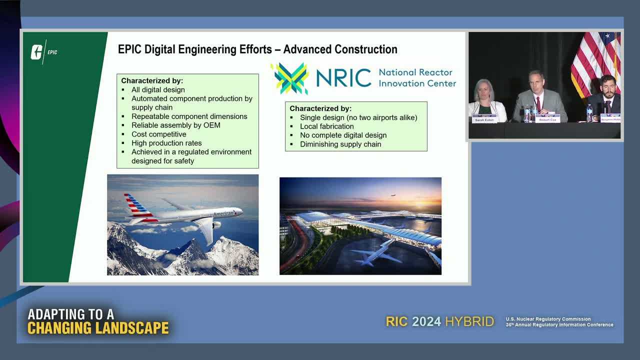 Going back about five or six years ago, our team at University of North Carolina, Charlotte, and our team focuses on issues related to energy production, but going back about five or six years ago we were looking at a lot of what we were doing in the advanced manufacturing. 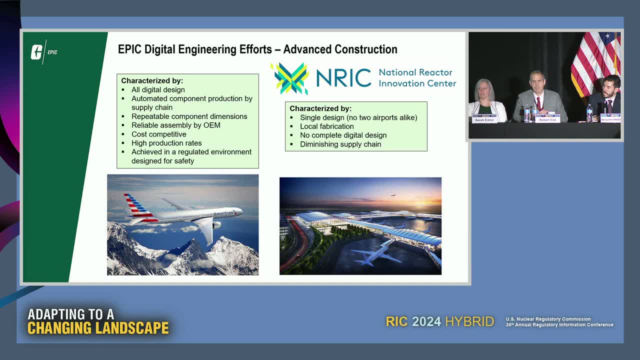 space and beginning to think about how some of the digital engineering techniques that are used in advanced manufacturing Could begin to be applied to construction generally and nuclear construction specifically. A lot of the issues that we see in building nuclear plants I always say kind of relates. 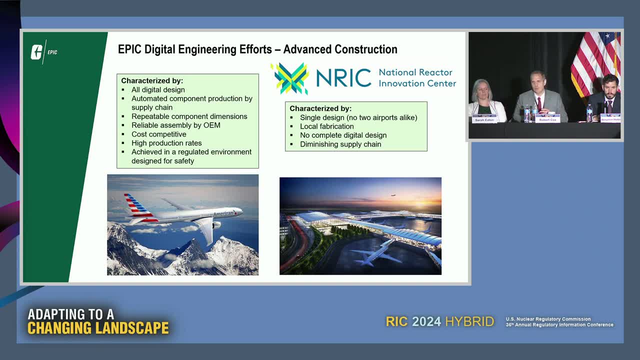 back to moving dirt and pouring concrete. Those are a lot of the issues that affect schedule and cost, And the issue with building an airport is that everything's sort of one of a kind, But given the move towards really using advanced manufacturing techniques to prefabricate a 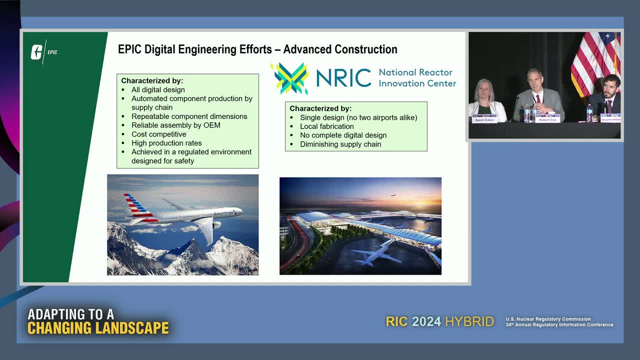 lot of parts of the plant. we have the ability to potentially leverage some of those digital tools in a better way, And so some of the work that we're doing right now- that my team is doing- is part of the advanced construction technology initiative under NRIC, and that's why I mention it here on this slide. 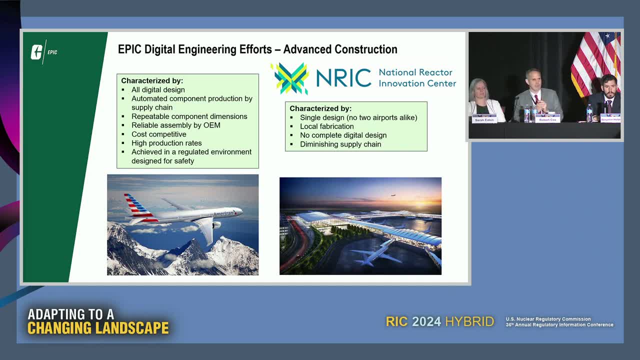 So I want to talk a little bit about how we do that. So I'll roll through the next couple of slides real quick here. On the next one, what we talk about with respect to what is a digital twin: it's always a two-way. 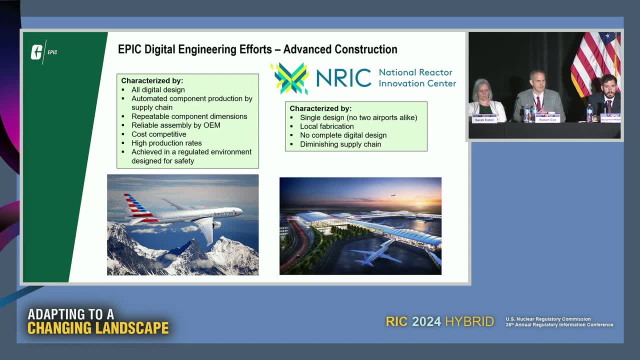 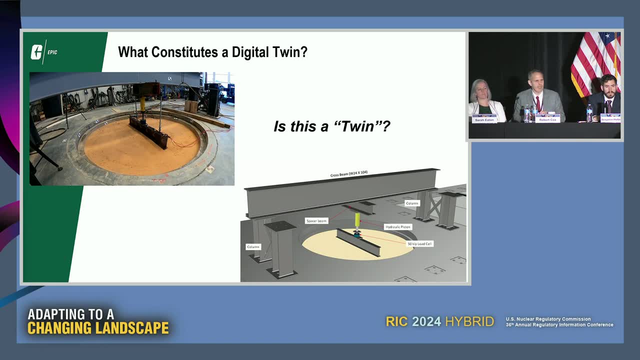 question. It's a tricky question. Next slide, Is it? There we go. So when I talk about what is a digital twin, just a level set, what you see there on the left is an actual physical object and what you see on the right is a model of that. 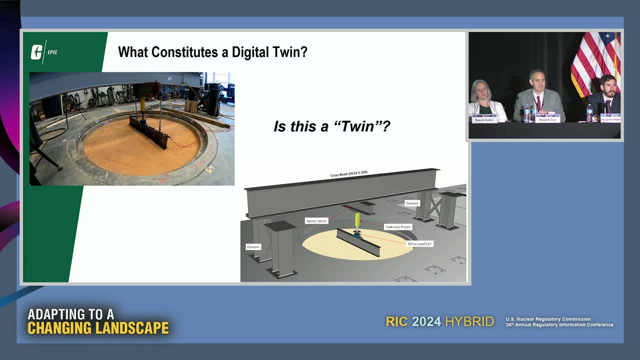 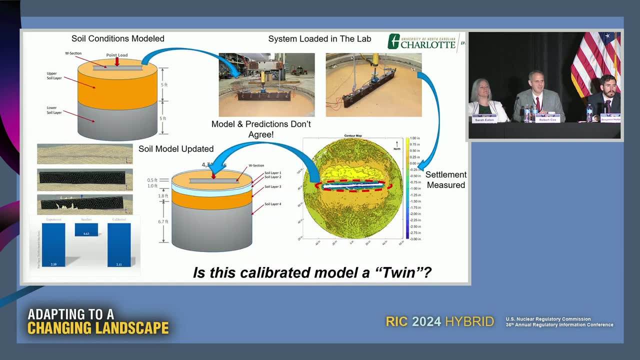 Now one question we ask: is that a twin? And I would say no, it's not, It's a model. That model looks like the real thing, but it's not quite a twin. Next slide And the next question I always come up with: 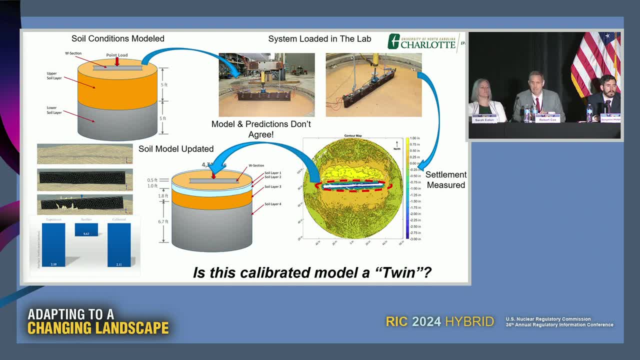 This is the same sort of structure. If I have a model of that structure and that model can be updated to match reality, is that a twin? That's approaching much more like what I would say is a real twin, But ultimately the bigger picture if I talk about what is a true digital twin, if we go. 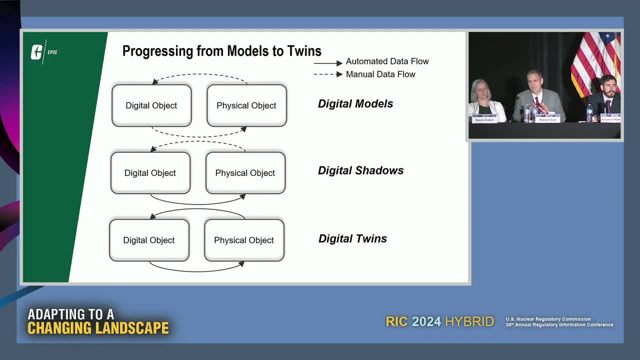 to the next slide. what we ultimately talk about in the research context is ultimately a digital twin, is that bottom picture where I have the physical world and I have a model of the physical world and those two things are seamlessly interchangeable And there's automated data flow from the real world to the model and from the model back. 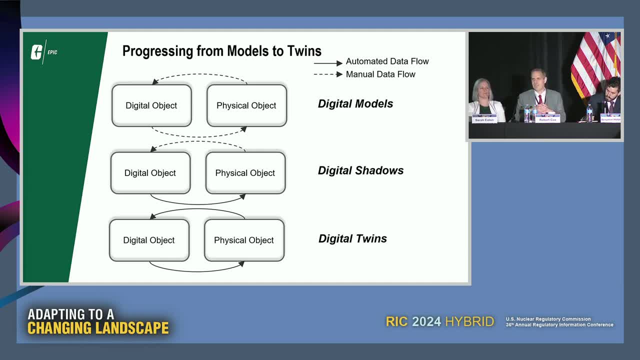 to the real world. We're nowhere near that yet. right, That's the highest level of digital twin. What we're really trying to do is to begin this sort of pathway of using digital tools to really improve. I don't like the term twin, but unfortunately everyone's using it and so we need to talk. 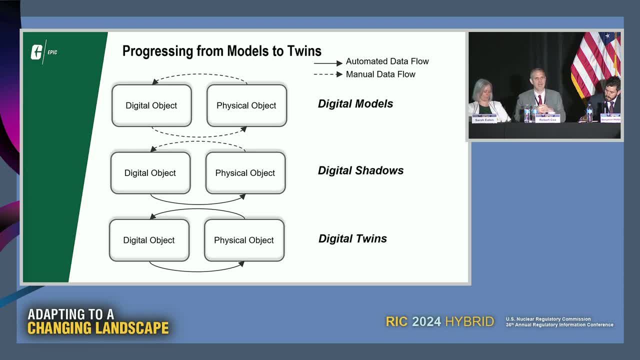 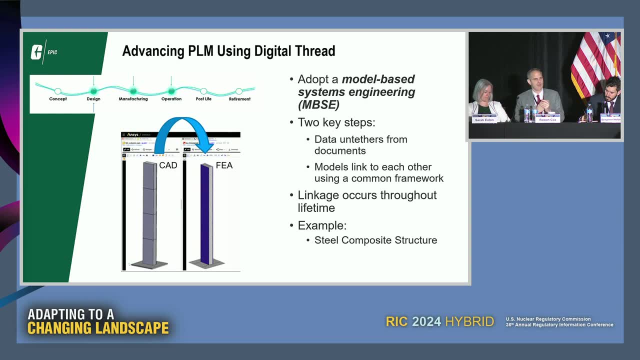 about what that means. So where are we on this path? So next slide. What we kind of talk about in general- The term that I like to use- is in the manufacturing world. we talk about product life cycle management, And if we talk about aircraft, everything kind of fits into this product life cycle. 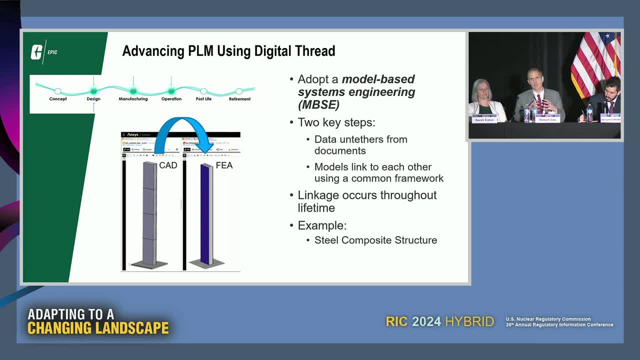 management world where basically what we do is we use model-based systems engineering. So essentially what we do is we have models that we develop at the design stage and we carry those models throughout the entire life cycle of a component. So at the top there is basically a chain where we go from design. 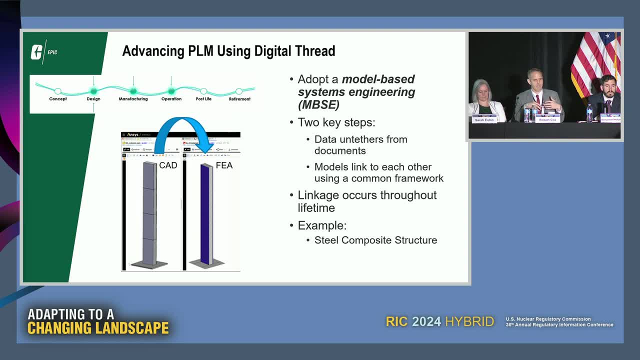 We go through construction all the way to end of life. What you can begin to do is if you use this model-based systems engineering approach, you develop models at the beginning of the life cycle of a component or a product, You map it across, all of the serial numbers of that product that you make, and you also 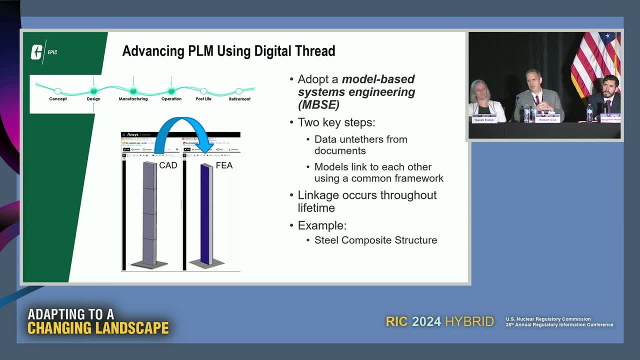 try to track everything throughout the entire life cycle of an individual component. There's two key things about that. One is that you begin to take data and you untether it from documents, which is important- right to make linkages between things. 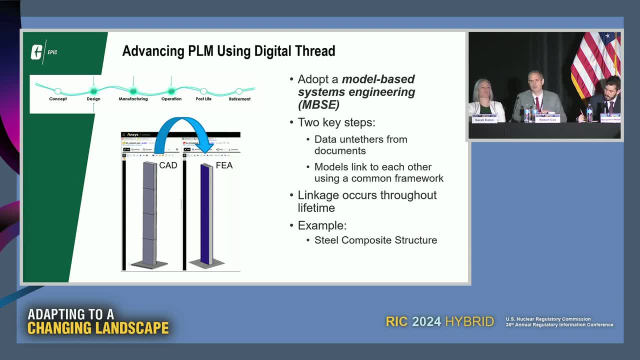 My second point there about I can begin to link models to each other. So here I've got a simple steel composite structure that we made in our laboratory where basically we have the CAD model and the finite element model for that thing that are inherently linked If I make a change in. 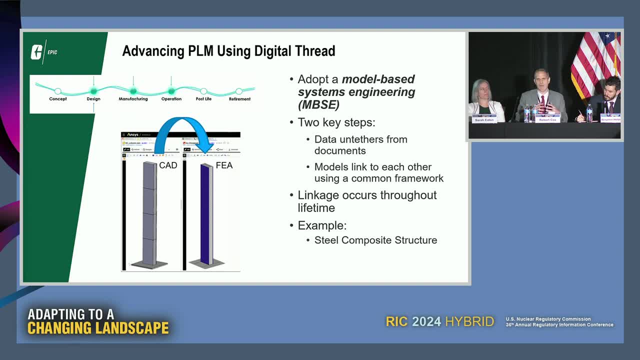 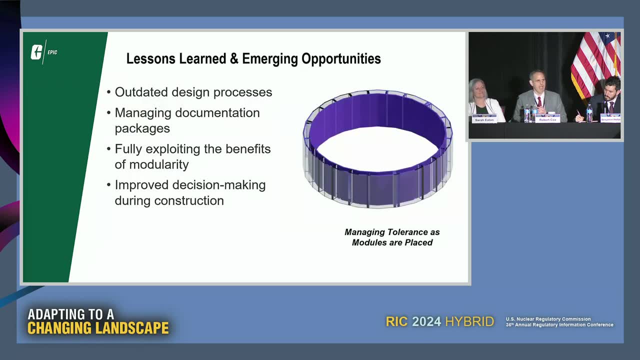 one, it makes a change in the other. That's one of the powerful things about these digital engineering techniques: Next slide, Next one, I guess There we go, Yeah. so a lot of what our team was trying to focus on was basically how. 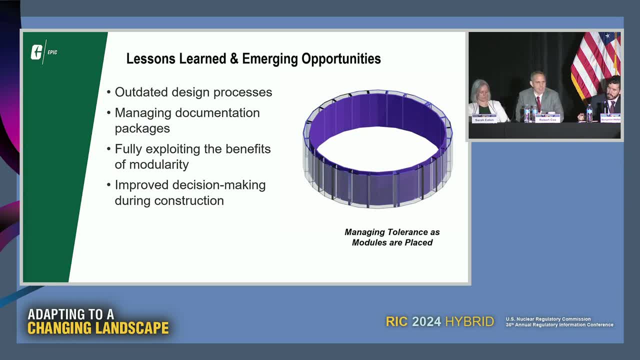 we begin to use those techniques based on some of the findings that have come out over the last couple of years with respect to opportunities to use digital tools. So, going back a couple of years, NEI report, EPRI report, MIT report that talked about construction specifically- 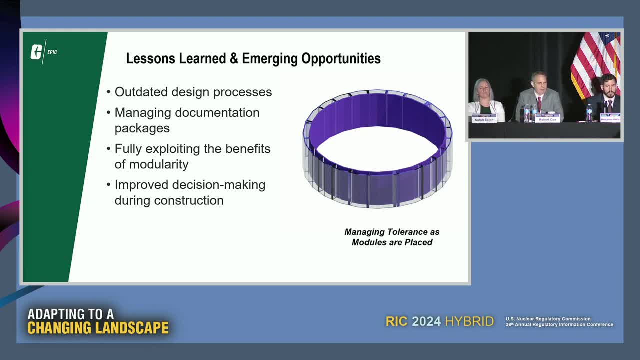 And sort of four key areas that we looked at. coming out of that was: first of all, there's been a long-standing history of using outdated design processes in construction in general, So how can we begin to introduce digital techniques into that? Digital techniques can help you to better manage. 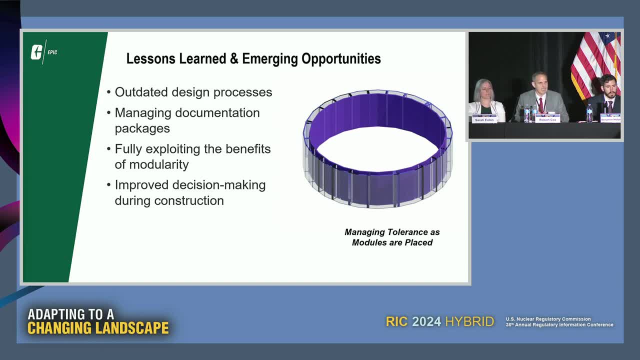 documentation packages and really begin to allow you to do better decision-making and really exploit the benefits of modularity. So what I have there is sort of an example that I'm going to talk about, But basically you know a lot of these structures. 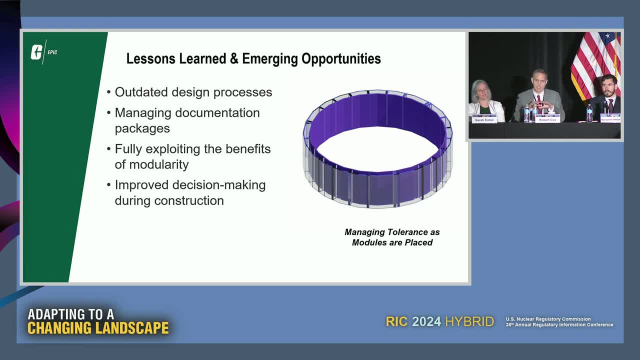 are going to be built, or a lot of. let's say, the reactor building is likely to be circular or likely to be underground for a lot of these newer SMRs. So what you see here is basically, if I you know, with steel composite. 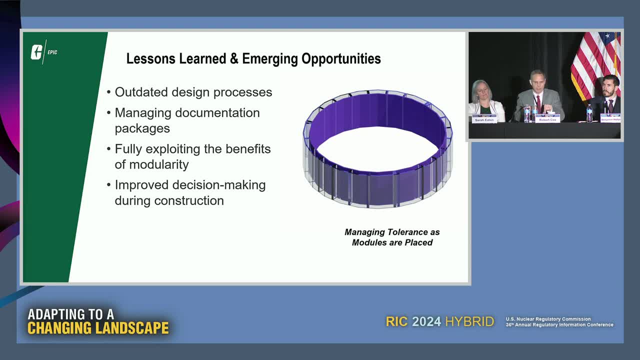 right. for instance, with the X300, one of the things they're looking to do is steel composite for the reactor building. You can begin to, because those are going to be those modules will be built off-site, right, you can begin to do some interesting things potentially. 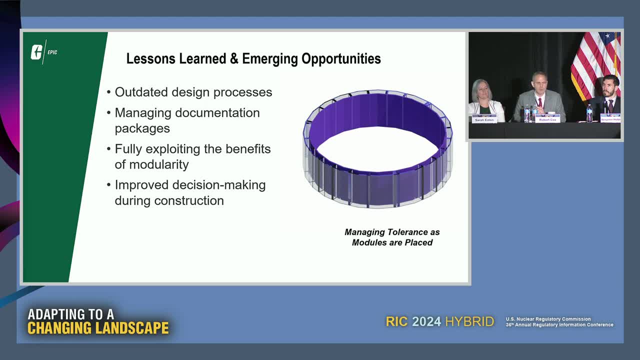 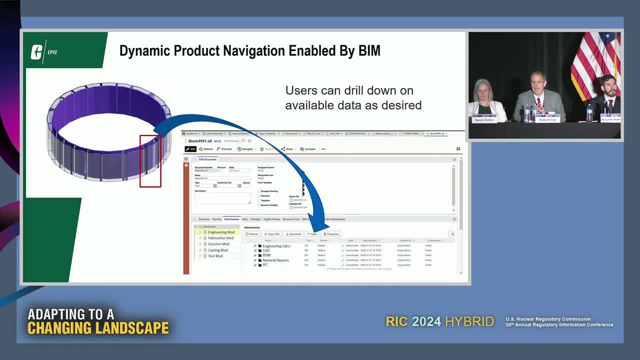 to track those modules as they move through their lifetime, And I'll use some examples of that as we go through Next slide. So one of the things that we look at trying to do, say so, documentation packages is a potential issue that's always been noted in the construction process. 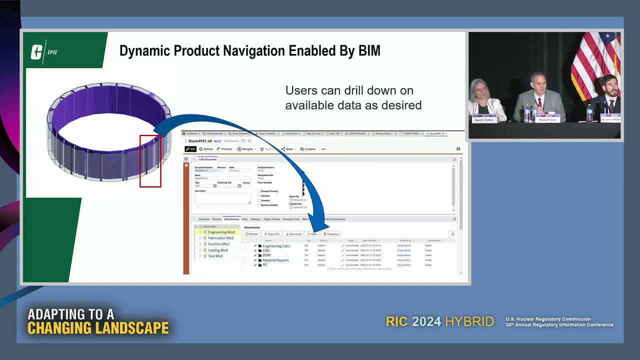 One of the things that we, you know we've done is utilizing basically something called dynamic product navigation. So basically, each of the modules that you have there, we've basically created it so that you have a clickable model of this particular, the entire structure. 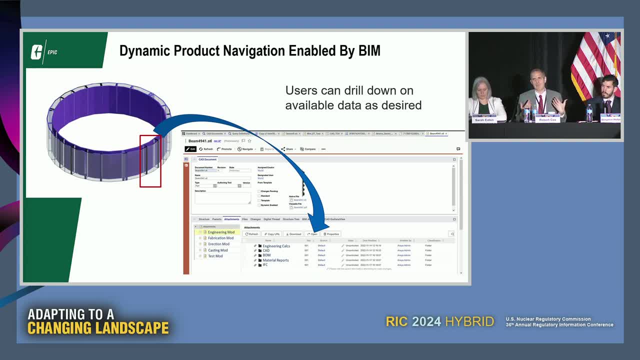 and you can basically drill down and track the entire life cycle of documentation associated with that particular module. So if you want to know what was happening at the fab, if you want to know what's happening on-site at some different aspect of the construction, 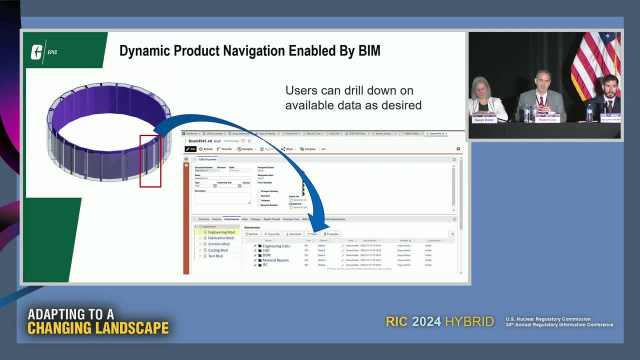 someone can pull up that information on-site, you know, if you want to know what's happening on-site, even on a tablet, right? So that's something that we can easily kind of leverage moving forward, and it's a pretty powerful technology. 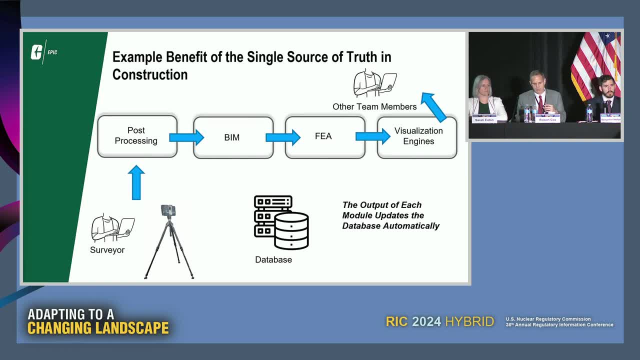 Next slide. Now we often refer to these things as kind of the single source of truth, because one of the concerns always is: if I have multiple documents and everything, there can be errors between those documents. So we begin to talk about a single source of truth. 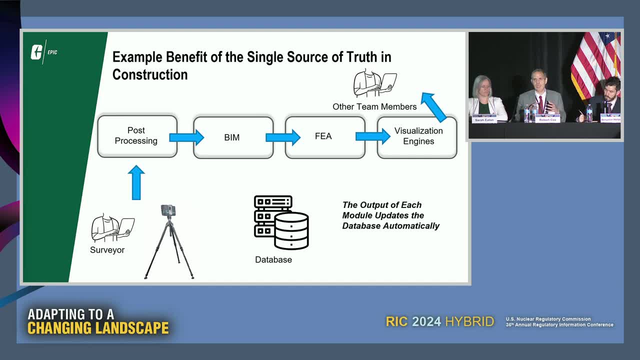 where essentially there's a single database where all of the key information is tracked. So, if you think about that image that I showed on the previous slide, if you clicked on one of the modules, I should be able to see all of the data for that module. 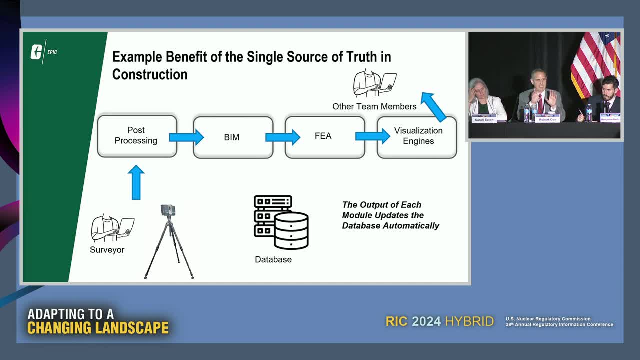 and be able to see how it's progressed throughout its entire lifetime, And that's tracked in a computer rather than in sort of a standalone hard copy document. So you know, essentially what we talk about is is. I could begin to, and I'll use this example here. 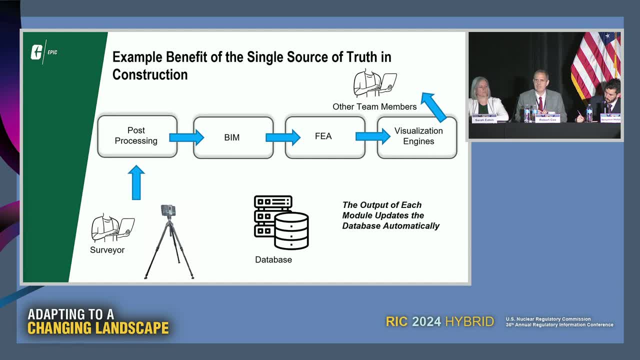 essentially I could have a surveyor that's on-site that is collecting information about the actual construction build. He could take data from a scan or a laser tracker measurement, something like that, post-process that data on-site and have it immediately update the CAD models. 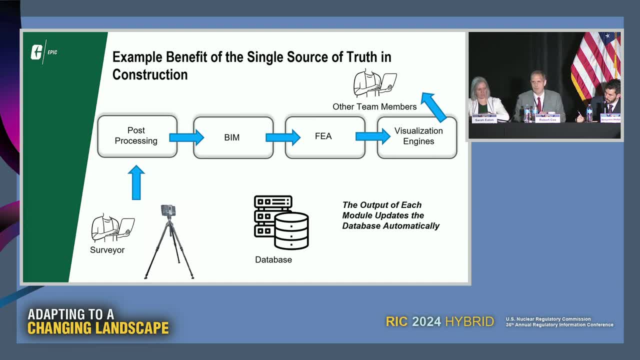 and the finite element models and to be able to share that information with team members broadly, And you can do that in a matter of minutes. okay, At least with some things that we'd like to do, You can do it in a matter of minutes. 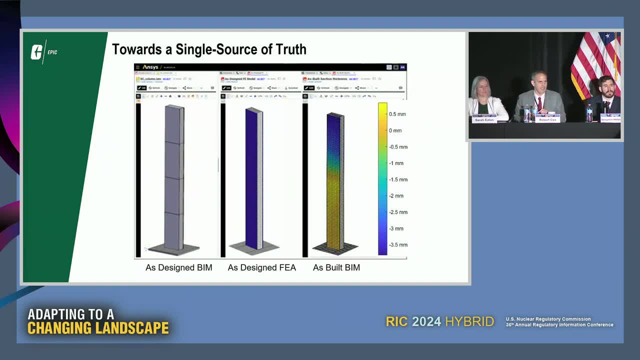 Next slide. So, as an example of that, what we do here is- this is again an example from our laboratory- where basically what we can do is we have our as-designed models and then our as-designed models. we can do this: as-designed models and then our as-designed models. 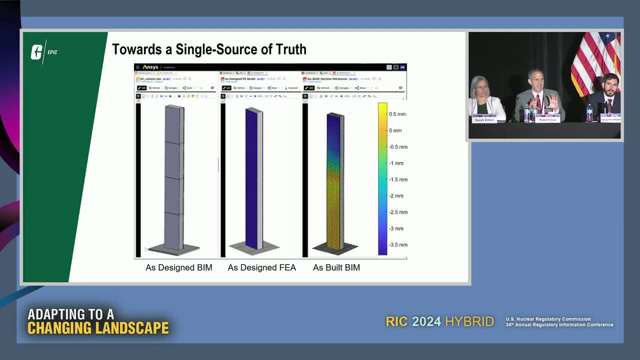 design, finite element and as-built models we can basically track using information that we've gotten from our scanners. we can go back and say: this is what we designed it to be, this is what it is right now, And we can update those two things and we can go back and forth interchangeably to compare. 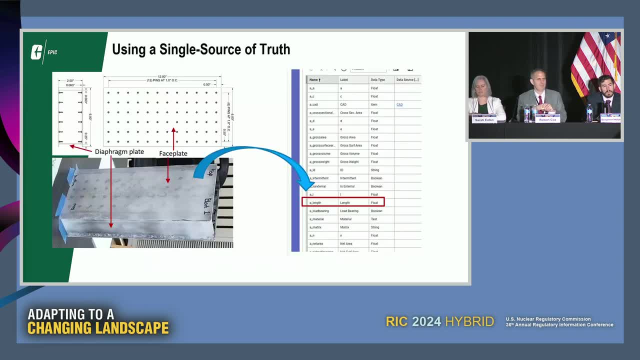 the design to what was actually built. Next slide Now, what is important about this, as I said, is a single source of truth. So essentially what we have is a database behind all of this where, as an example here I'm looking at sort of my example, steel composite module I've got in the lab where, basically, 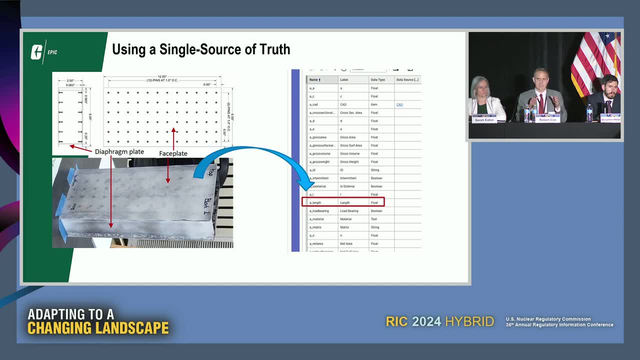 individual parameters like the length of that thing exist as individual parameters. I can track what it was on any given day throughout the actual life cycle of it, from the time it was designed to the time where it is right now today, in real time. 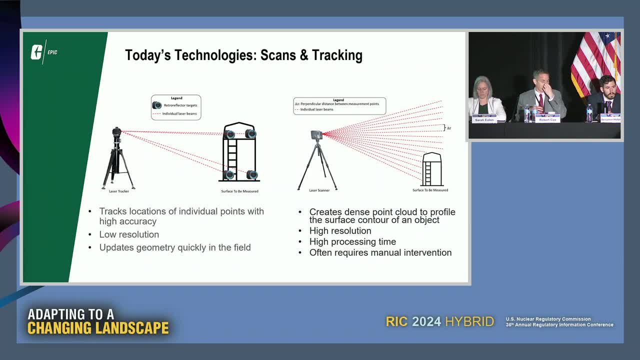 So with that, to my next slide. one of the things that we look to be able to do with this is to leverage technologies like laser scanning and laser trackers. So in my image there, I'm not going to go through all the gory details of this, but if I look at my image there on 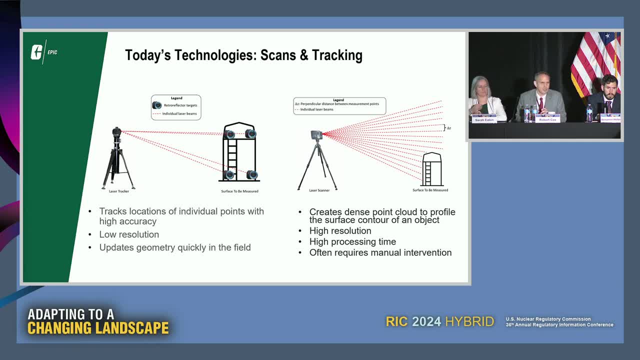 the left. what I have is something called a laser tracker right. So if you go on a construction site, you can see people with a laser tracking device. What I can do is basically do a quick scan and I can If I have targets on those modules. what we can do is we can actually track where the 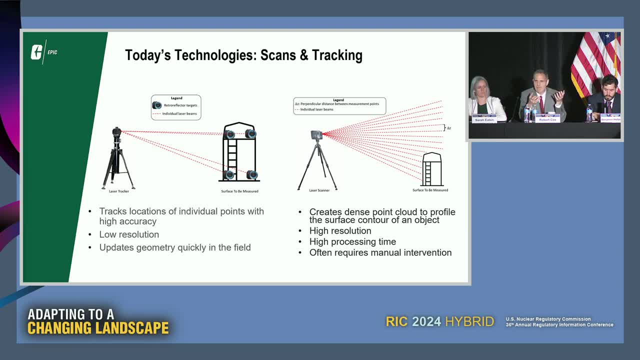 modules are placed in 3D space. We can take that information, feed that information back into our systems in the cloud and then update. you know where a module is placed. And we can also use laser scanning to be able to get a sense of how wavy potentially the 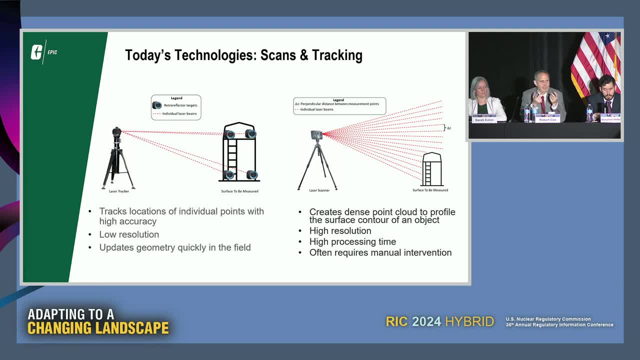 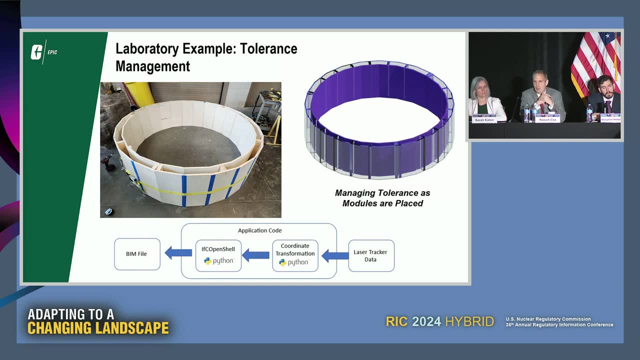 surface may be of one of those modules. So on the next slide there. So here's an example of where we might use that. So imagine if we're building a steel composite structure. So it should be a great benefit to use modular construction techniques. 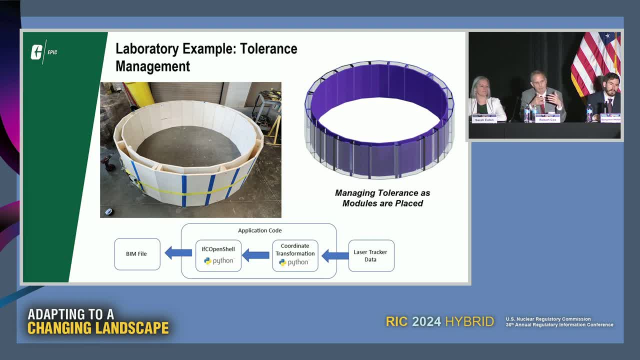 I can prefabricate things before I bring them on site. Well, when you begin to place those modules on site, there's a question of tolerance management, right? How do I make sure that when I place one module I haven't offset it too much, that I need to worry about where I place the next one? 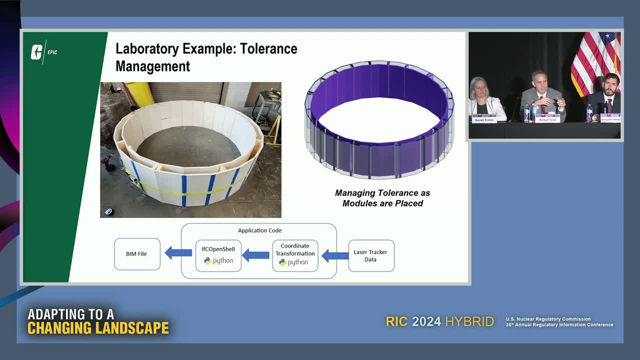 So what our team is looking to do basically is to take that image there on the bottom. basically, Again, this is a. Those are not, obviously steel composite modules. This is what we're doing in the laboratory right now, using plywood, but basically it's. 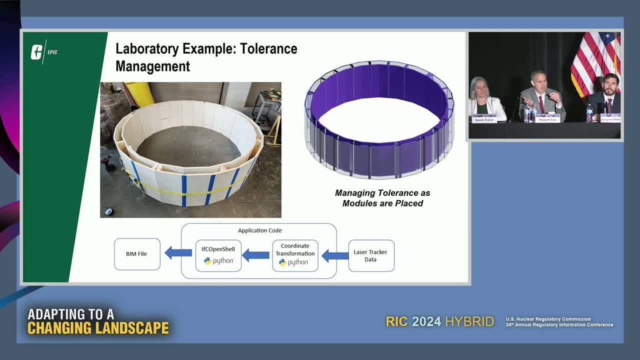 the same concept, Essentially trying to take the laser tracker data and be able to feed that information back into our models to update things and basically using that for being able to help us Implement a tolerance management program. So you can begin to imagine where this sort of thing might be useful in the construction. 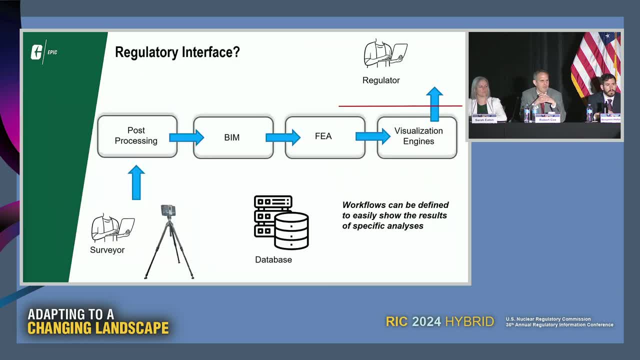 process, Next slide. Yeah, we'll jump ahead there, Yeah, So now the question as we develop this is the interface on the regulatory side. If we talk to folks in the construction world, they like a lot of the concepts associated. 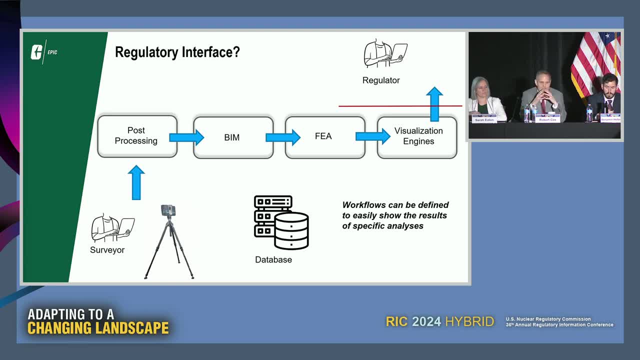 with this, but what scares, Frankly, what scares the crap out of them, I think, is that the regulators could see all the gory details of what may happen- Yeah, Of what may happen- in the process. But one of the key things that we need to think through is: how do you actually expose? 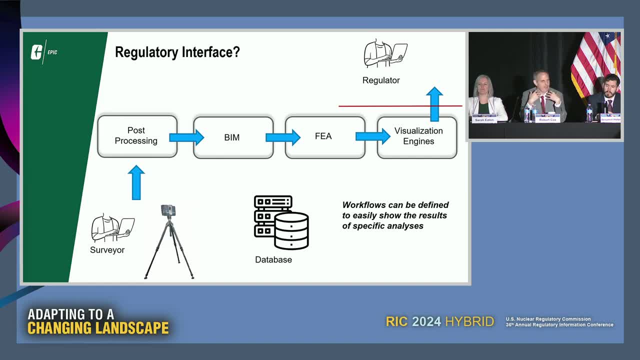 this information appropriately to a regulator. given that you- I mean you've got enormous amounts of data that you can track, It's got to be useful. but we don't want to track so much, potentially, or expose it at the wrong times, that if we get data that we're not certain about, we can begin to get into. 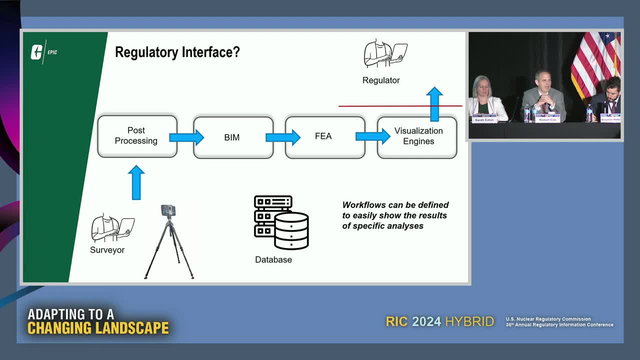 an analysis paralysis loop and I think that's the concern that a lot of folks have. But it's an exciting time to leverage some really new Interesting technology. So with that I will leave it there. Thanks, Robert, I know I learned a lot from that and I appreciate it. 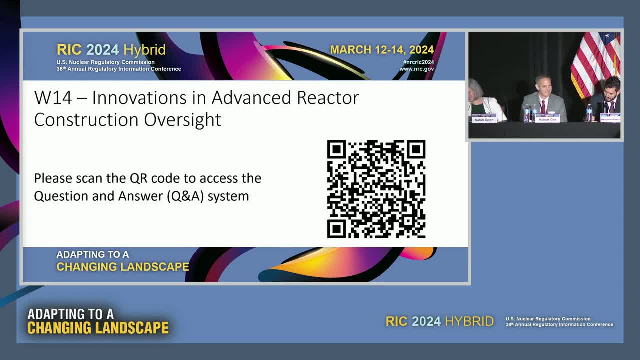 I now want to come down and maybe take a class from you and learn even more. so thank you for that. With that, I'd like to introduce our last speaker today, and some of you may be aware that the NRC and our Canadian colleagues at CNSC have been partnering on a number of 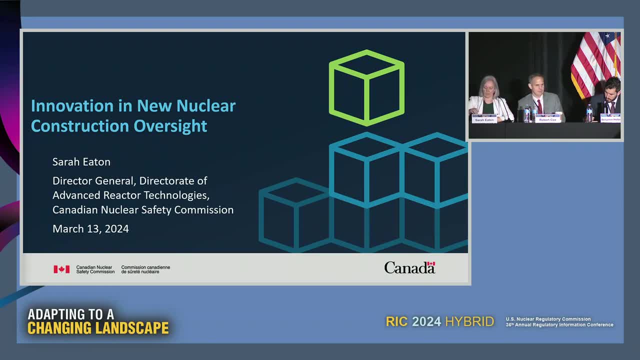 activities related to SMRs and advanced reactors, and so we welcome Sarah Eaton, the Director General of the Directorate of Advanced Reactor Technologies at the CNSC. Her directorate is responsible for licensing new nuclear reactors, pre-licensing activities, including the vendor design review and leading SMR readiness project for the CNSC, ensuring 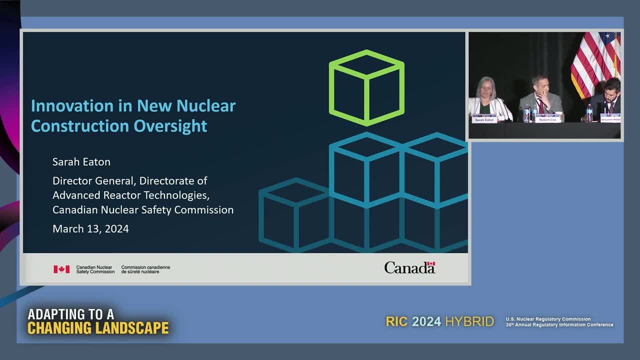 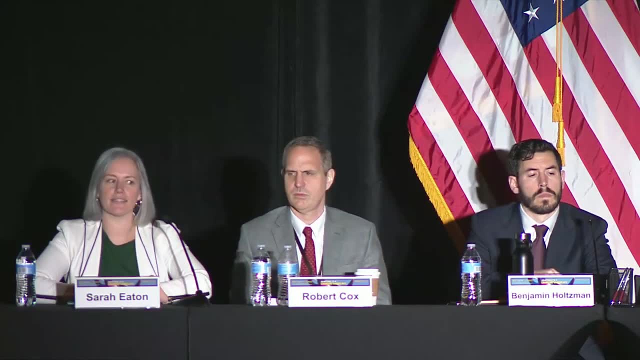 a coordinated matrix approach to organizational readiness for regulating SMRs and new advanced technologies. So with that, Sarah, please, Awesome, Thanks so much. The benefit of going last is, I can just say, agree with Nicole, Agree with Jonathan, Agree with Ben. 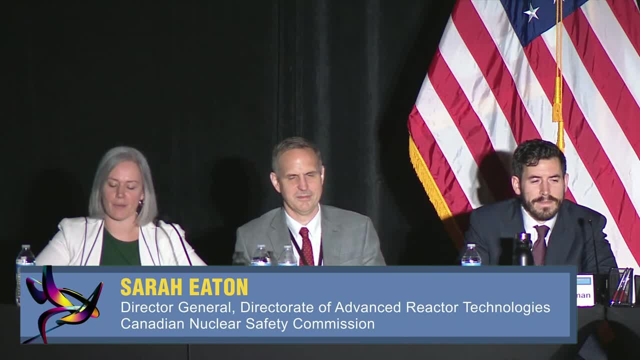 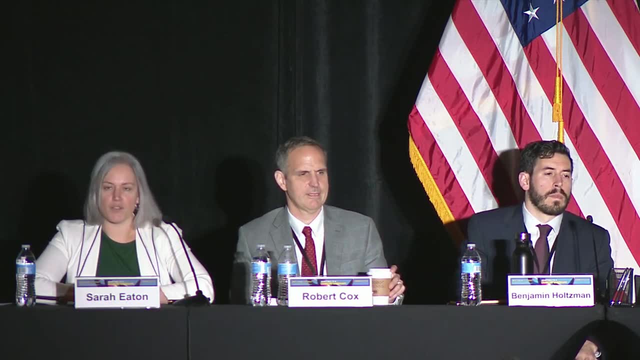 Agree with Robert and call it a day, But I am really happy to be here to talk about the Canadian landscape and the work that the Canadian Nuclear Safety Commission is doing in this space. Next slide, please. So I know every single one of you lie in bed every morning as an American and think. 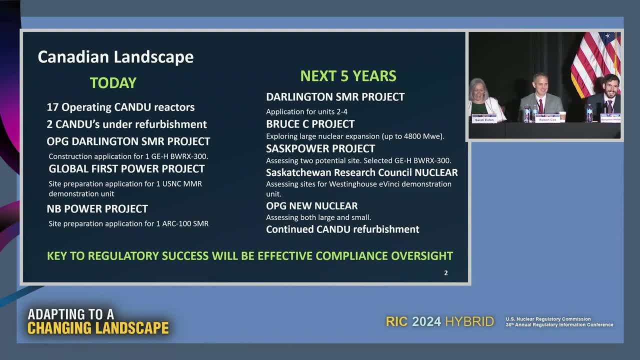 I wonder what is going on in Canada? Well, luckily, today you'll get your answer. So on this slide we have on the right where we are today and on the left on where we think we'll be in five years. 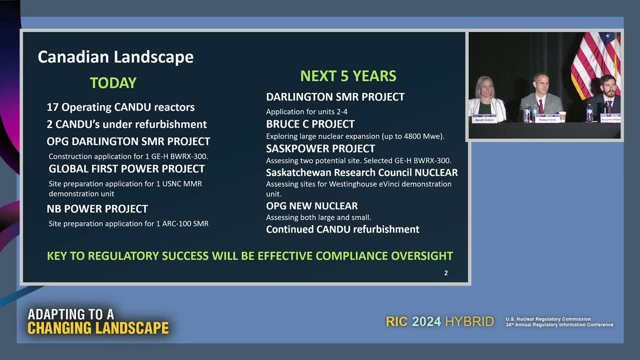 And even since I've finished this slide, I'm going to go back to the slide where I I feel like the five-year slide probably is out of date already. So today we currently have 17 can-do reactors that are either in operation or refurbishment. 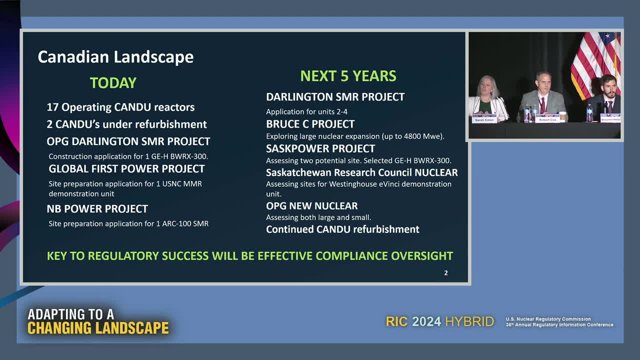 And then we have three separate SMR projects with three separate technologies. Looking out five years, we have additional SMR projects, likely some of the same technologies we're reviewing today, possibly some of the different ones. We have new advanced technologies and, we have to be determined, large nuclear power plants. 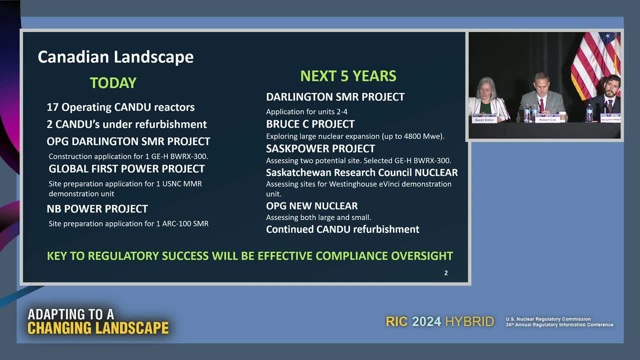 So I'm not going to walk through every project in the timelines, but I am going to draw focus on what's been mentioned before on Ontario Power Generation's proposal to deploy the BWX-300 at the Darlington site, as this is the project that's front and centre for us. 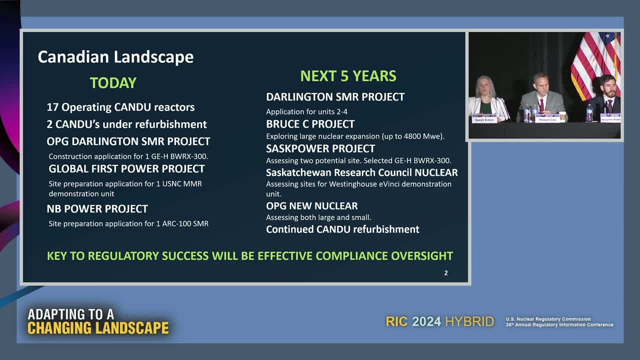 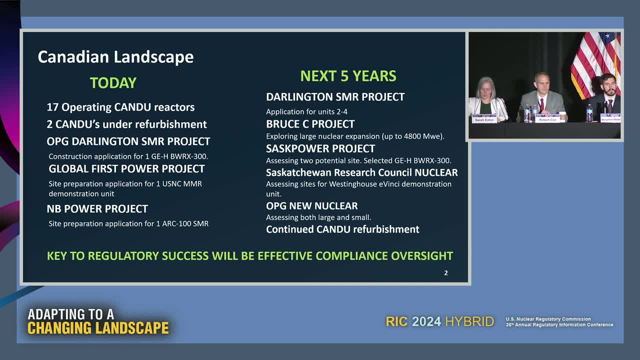 And, to be honest, industry probably is going to throw in at least one more. So of these technologies, Canada's posed to be potentially the first deployer in three or four of those technologies. So it's a little bit of an unenviable position as a regulator to have everything Ben's laid. 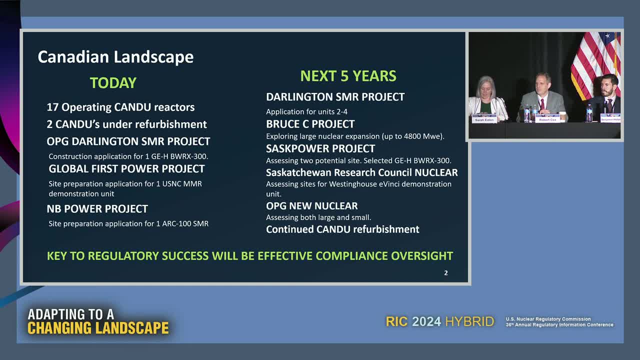 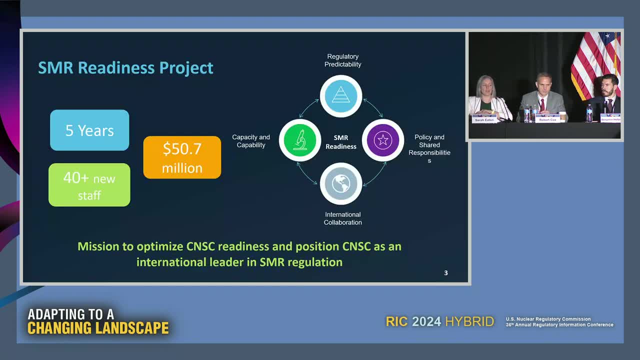 out in front of us on scale of deployment, on rate of deployment. But luckily, we've been thinking about this for a while, over a decade, And if we go to our next slide, it brings us to our SMR readiness project. 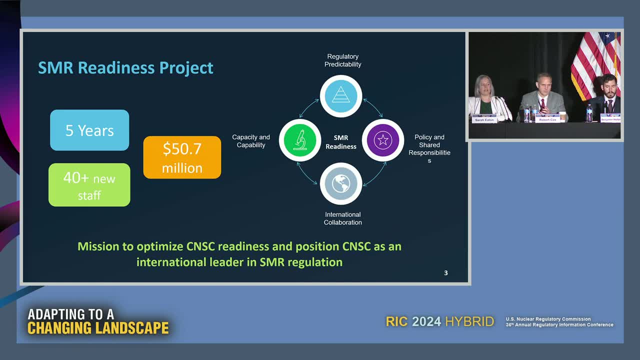 And so we talk about SMR readiness in how it will prepare us for advanced nuclear, for small module reactors, but it will prepare us for any new nuclear deployment that occurs in Canada. It doesn't matter about size. In 2022, we initiated this project, which represents an integrated approach to optimizing. 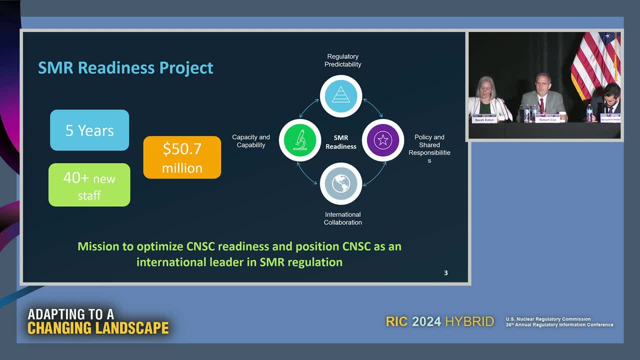 our regulatory readiness for small module reactors and advanced reactors. We have a budget of $50.7 million a five-year timeline and through that we aim to address 60 objectives Over 60 objectives, which will help us prepare for new nuclear. 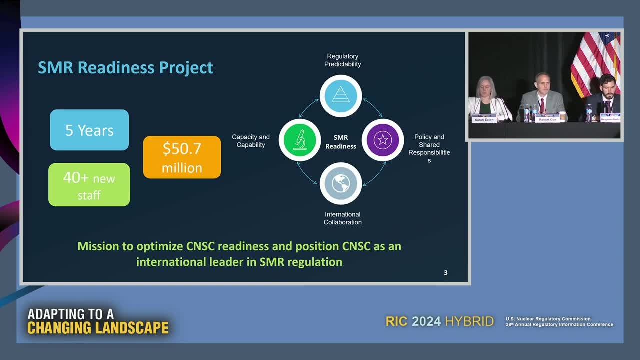 We've organized our project into four pillars, the first being regulatory predictability- everyone's favorite pillar, which really helps us be able to ensure that our regulatory framework is up-to-date, technology neutral and has the necessary guidance and information that new applicants will need to be able to navigate the regulatory space. 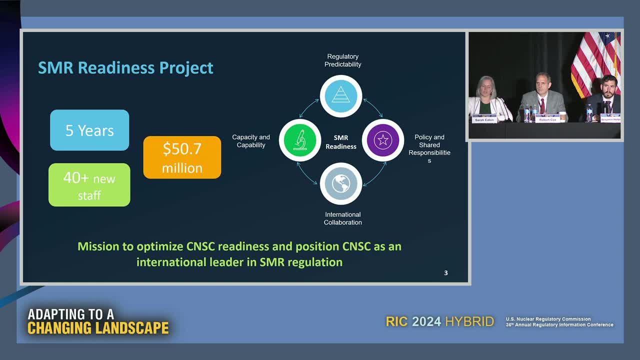 We have policy and shared responsibilities, which is our work with our federal and domestic partners to ensure that we are having a one-run program, We have a regulatory approach and that we're sharing and leveraging information where we can. We have international collaboration, where we talk about the work we're doing with many 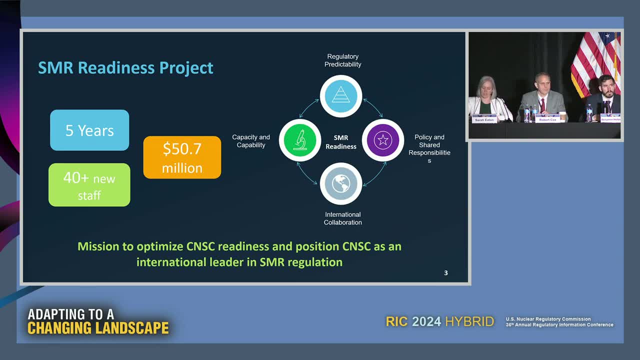 of our partners, including our very good partners here at the NRC, which helps us ensure that we are finding efficiencies where we can in our regulatory processes. And, finally, capacity and capability, which is really ensuring that we have the talent we need, that they have the skills they need to address what we have in front of us, which 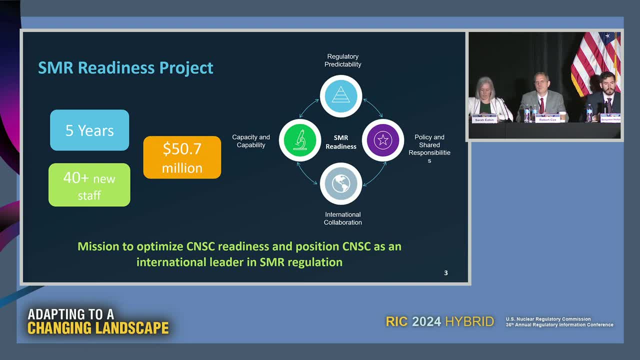 is a massive culture of change for us, And what comes next is a lot of work. What cuts across all of these pillars is that need for cultural change as we transition from expertise in one technology to expertise in multiple technologies, increased collaboration with other partners and the rate at which industry wants to deploy, innovate and change. 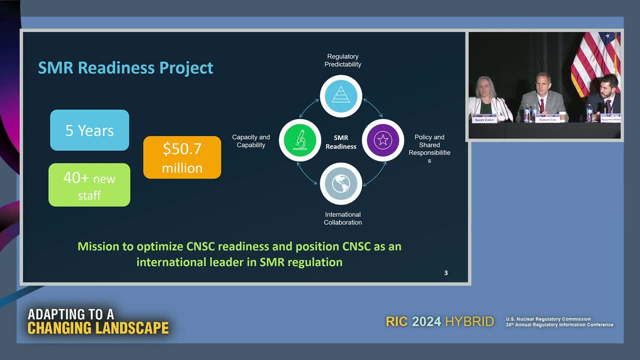 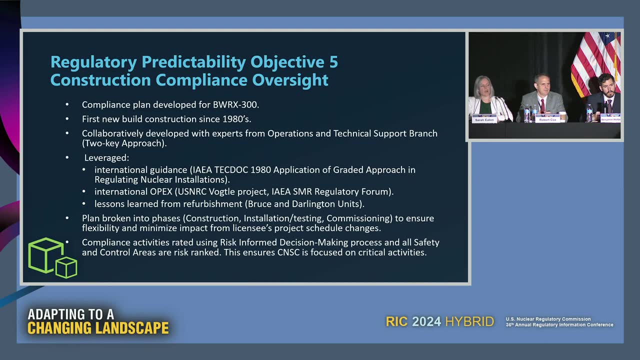 And so it's a culture shift for us and this readiness work really helps us build that culture change and be able to support it. Next slide, please. So I want to sort of bring our readiness project to the panel, the topic of our panel today. 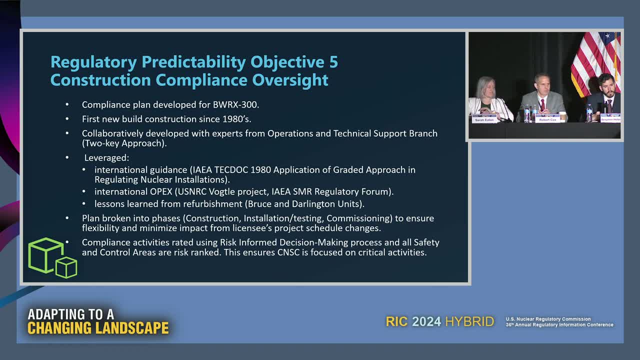 which is learning, And the first thing I want to talk about is looking at advanced construction. So, similar to what Jonathan and Nicole spoke about, their key principles also align with our key principles. So our newest can-dos, the newest can-dos- we have began construction the same year. 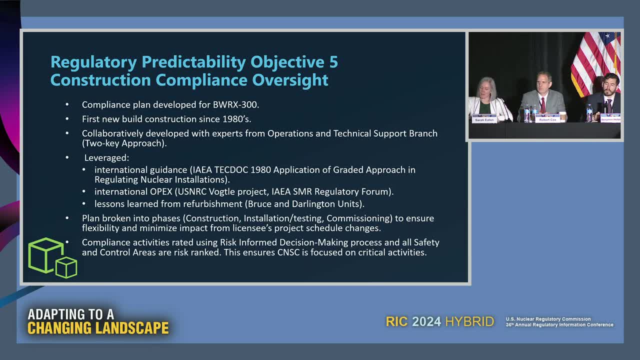 I was born 1981. And so, as today is my birthday, I really tried to link first concrete pour – thank you very much, thank you very much – I really tried to link first concrete pour to today, to March 13th. 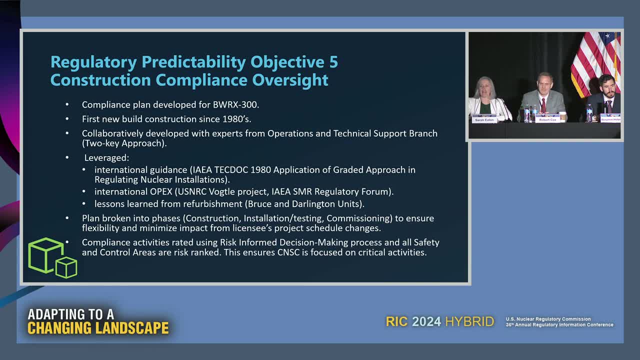 But sadly I could not Thank you. It was in June. So as a regulator we haven't overseen new reactor construction in over 40 years. So as a result, we have no modern compliance oversight plans and this objective deals. 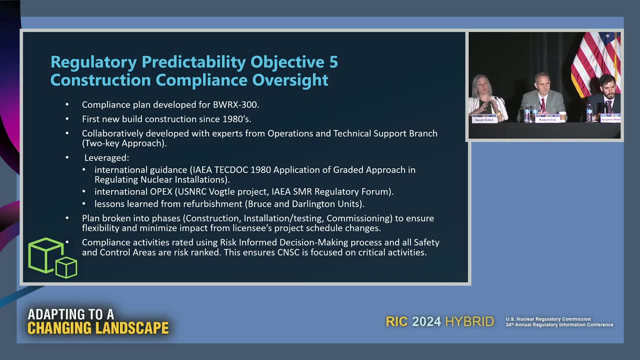 with that gap. This objective ensures that we have a generic plan that we can tailor for different technologies and we will use it should OBG be approved for the deployment of the BWX-300.. The team that developed this plan was – came from across the organization, ensuring a two-key 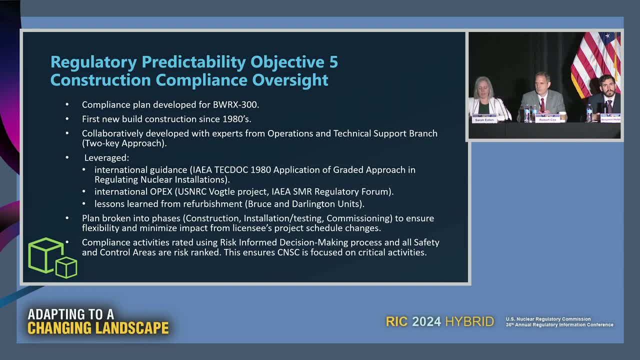 approach from our technical services branch and also our operations branch, And, while we don't have the recent experience as Nicole and Jonathan and Ben have described, there's lots of experience out there, So we've leveraged that experience to ensure that we can learn from those – from the 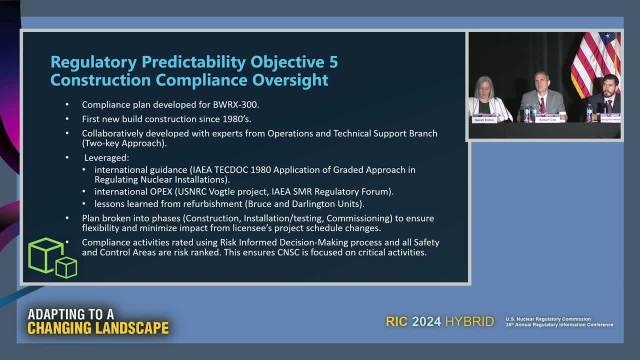 lessons that were learned and be able to find efficiencies in our program, And we also leveraged the lessons we've learned from our own can-do refurbishment, which has obviously been massive projects, which has allowed us to be able to modify and have agile. 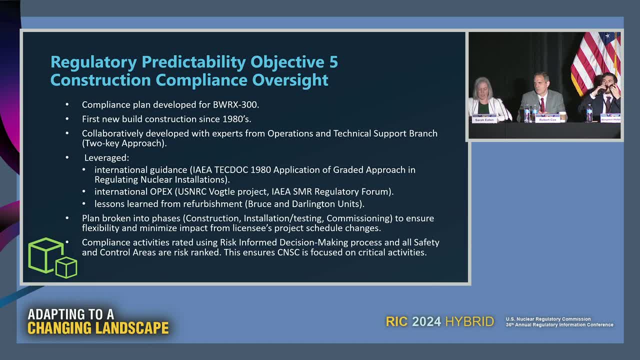 construction – sorry, agile construction. So we've been able to modify and have agile construction. So we've been able to modify and have agile compliance plans. And so, during this period of novel approaches to designs and the construction, it's critical for us to focus on the novel features, the first-of-a-kind features, using a risk-informed 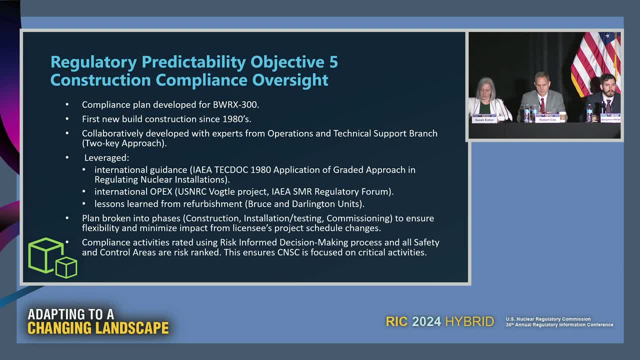 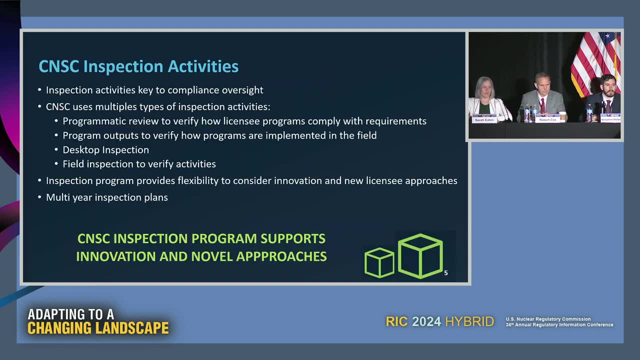 approach on what really matters. And this generic plan, as I said, will be tech-neutral. we'll be able to use it for multiple different technologies. Next slide, please. So our inspectors and our inspection program is robust and it's world-class. 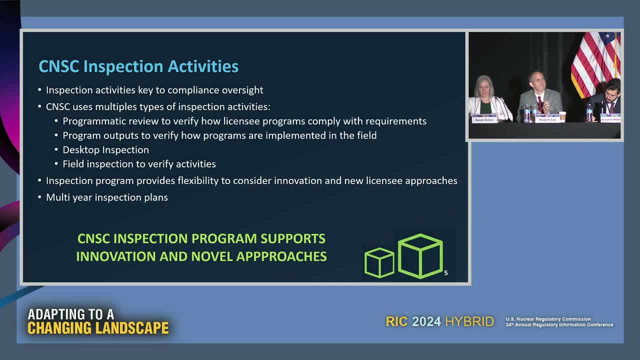 What we learned from COVID. that was, while virtual inspections, we were able to have a great tool to add to our toolbox. in-person inspections are critical for compliance oversight, and that is especially true for novel and new features. Like all mature regulators, we have a variety of inspection tools, and all of these will 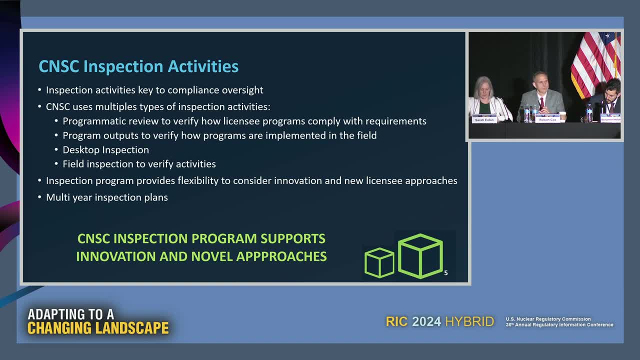 come into play for our current inspections and for any future inspections for advanced construction. We use a performance-based, risk-informed approach, multi-year inspection plan that allows us to consider – that allows the flexibility to consider for innovation and new license agency approaches. 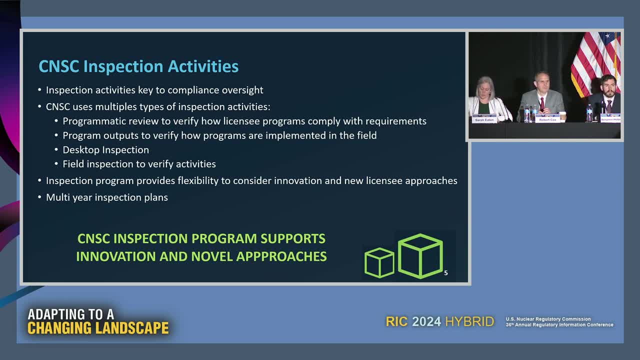 And these innovation tools for inspectors that we're looking at today, such as virtual reality, drones, artificial intelligence, are going to change at a rate that will be uncomfortable for us as regulators and will require, again, additional culture change. But burying our head in the sand and having a mouthful of sand isn't that comfortable. 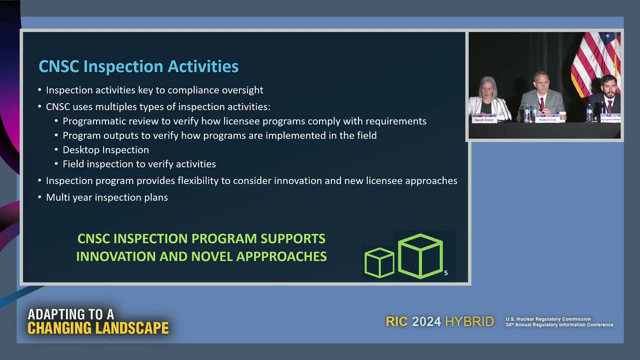 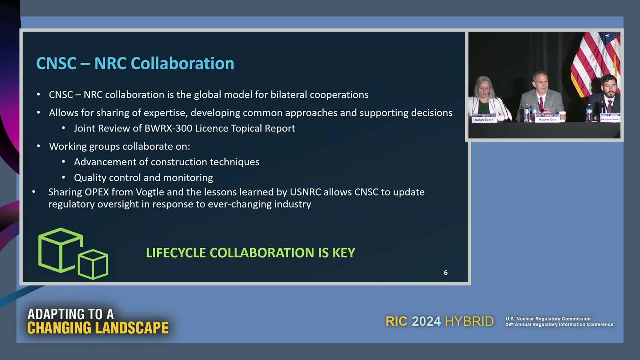 either, And so we have an expert group in our organization who's supporting us, working very closely with the Canadian industry to see how they are using innovation and how we can use those innovation tools. Next slide, please. So I'm not just going to talk about how much we love working with the NRC, because 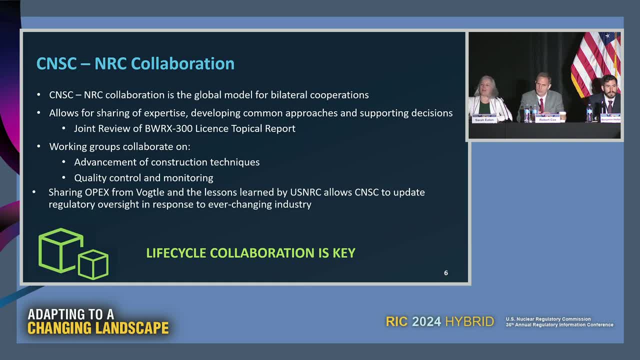 we love working with the NRC, but this collaboration really has been pivotal in our preparations for new nuclear in Canada. From our perspective, collaboration builds positive relationships among regulators, which for us is necessary for the safe and effective deployment – the broad deployment- of small 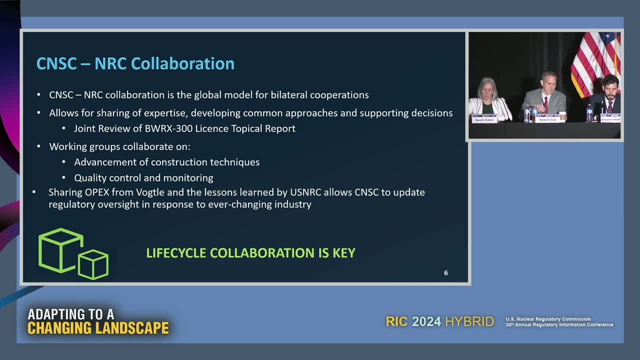 module reactors In 2019, we signed a memorandum of cooperation on advanced reactor and SMR technologies to enhance our bilateral cooperation, and last evening we were able to sign a trilateral agreement to bring the UK ONR into that as well. Our memorandum of cooperation allows us to do pre-licensing engagement, licensing reviews. 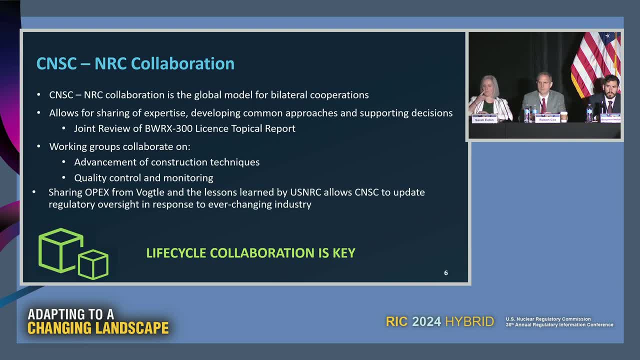 to share science, research and to develop common regulatory positions. For the BWX-300, we have a very unique five-party – it was five-party as of when I wrote these speaker's notes, now six-party – agreement which allows us to be able to work together. 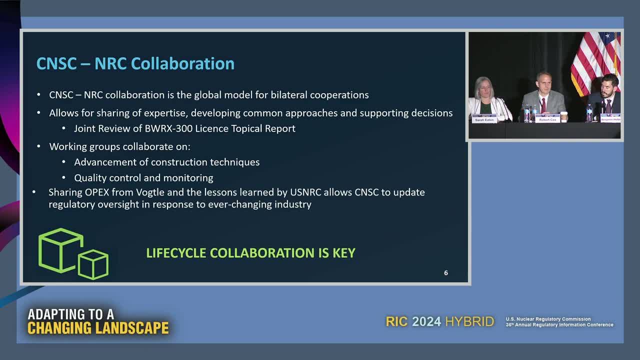 on technology-specific aspects. So we've been doing a joint review on advanced construction techniques and we're looking to work towards where we can harmonizing compliance plans, leveraging supply chain inspections, and this is really the lifecycle collaboration we need to be able to be efficient. 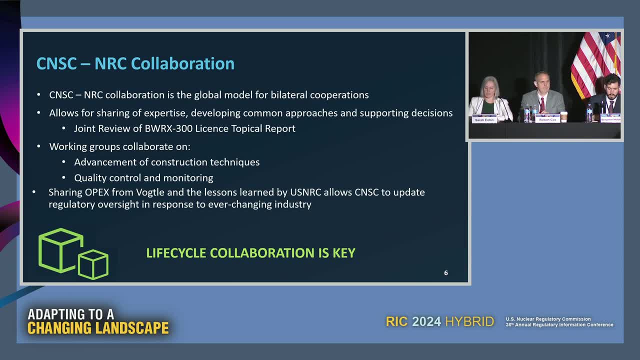 and effective regulators. once we have these standardized designs- And of course, our staff are learning from NRC staff- We're looking to be able to capture those best practices as we continue to update our new compliance plans but also our existing compliance plans. 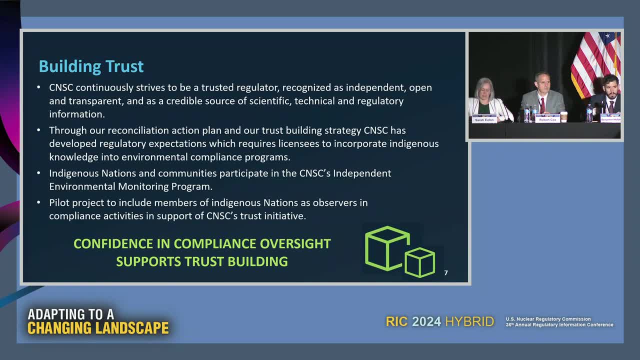 Next slide, please. So building trust, All of our readiness work, collaboration with international partners will mean nothing if we aren't seen as a trusted regulator and we are known for our independence. Through our trust strategy, we're strengthening our relationships with the public. environmental. 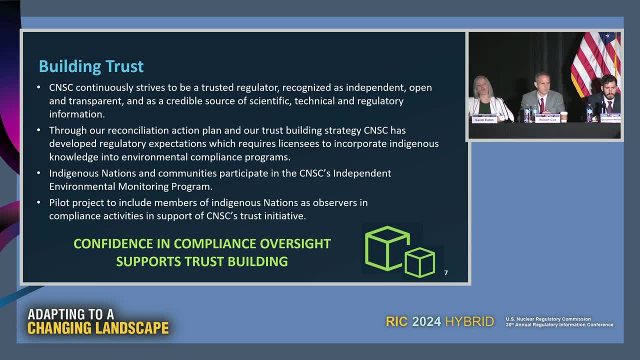 groups and Indigenous nations and communities. Developing strong relationships with Indigenous nations and communities is deeply important to the CNSC, and we're committed to building long-term sustainable relationships, And so part of that relationship building has been a request from Indigenous communities to participate in our independent environmental monitoring program and also to observe how. 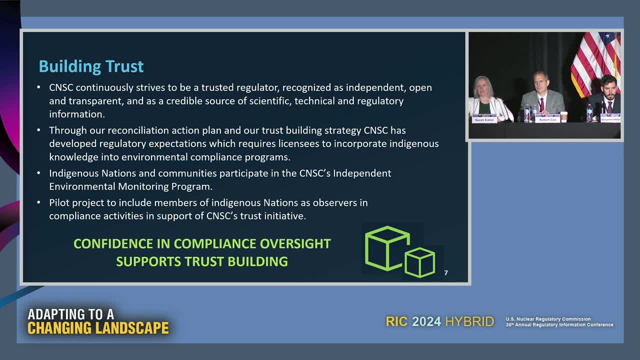 we conduct inspections And, from our perspective, this is a really important way for us to be able to share our experience that can help build a common understanding of the safety of our ongoing facilities- and the safety of our ongoing facilities, Thank you- And also the safety of these novel construction approaches. 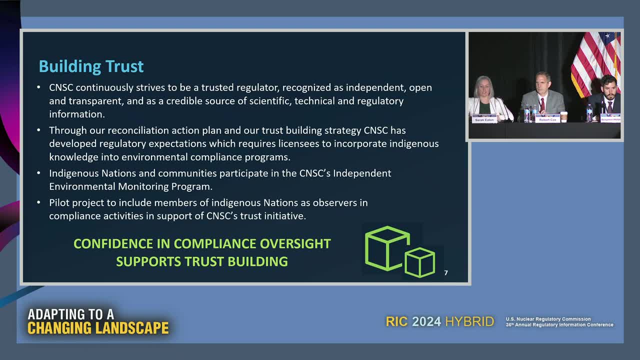 These approaches are first of a kind, and so, as scientific-based people, as regulators, we're working through how we can look at that through a safety lens. But for the public, it's brand new. For Indigenous nations, it's brand new. 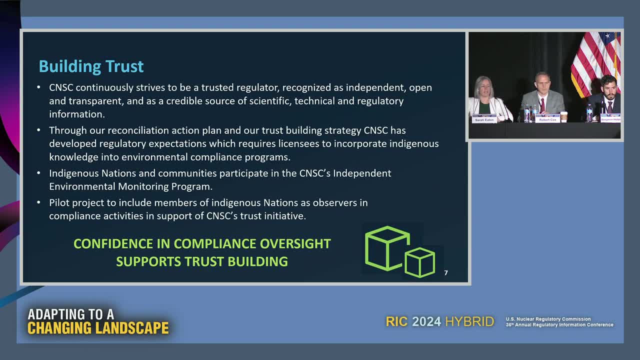 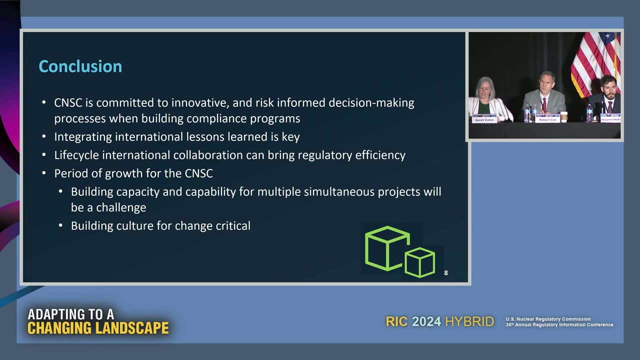 So it's really an opportunity for us to be able to share that information and to be able to include the lessons that we can learn from Indigenous nations and communities and continue to build that culture of change. Next slide, please. So, in closing, We are committed to innovative, risk informed decision making processes when building our 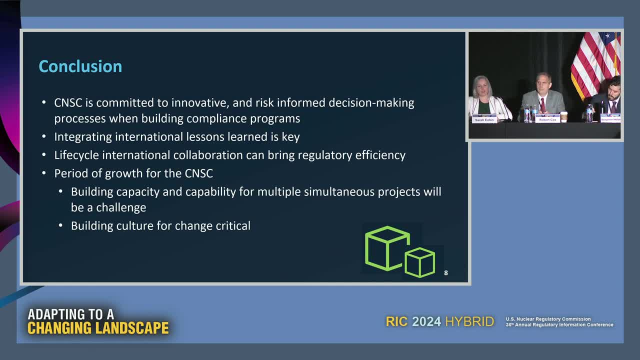 compliance programs. We don't necessarily have as much time as was shown on the NRC schedule to be able to integrate these plans and to be able to use them, And that's why, for us, integrating those lessons, international lessons learned, are key. For our perspective, international collaboration is a critical part to our work and it has 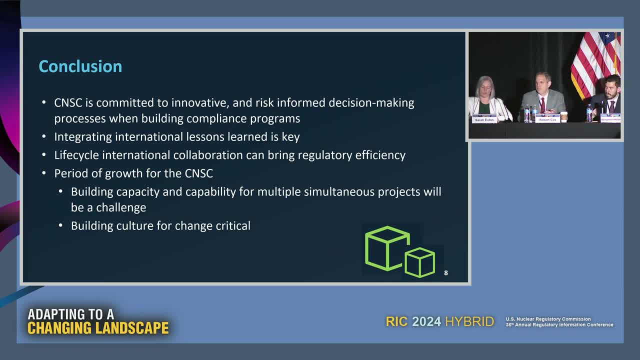 to be a lifecycle collaboration to ensure that we're able to gain those efficiencies over the life cycle And as we look at this period of time, I think that, as we look at this period of time and period of growth from the industry, it's a period of growth for regulators as well, where we have 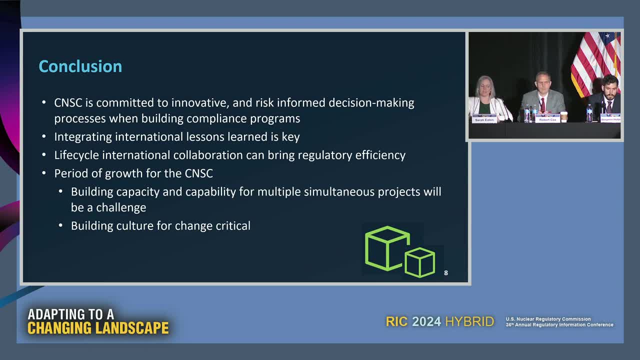 to build capacity and capability. we need to find talent in a place in a time when talent is not easy to find, and we also have to assess how we continue to assess. multiple projects, different technologies at the same time. building culture for change is critical, whether it's for advanced 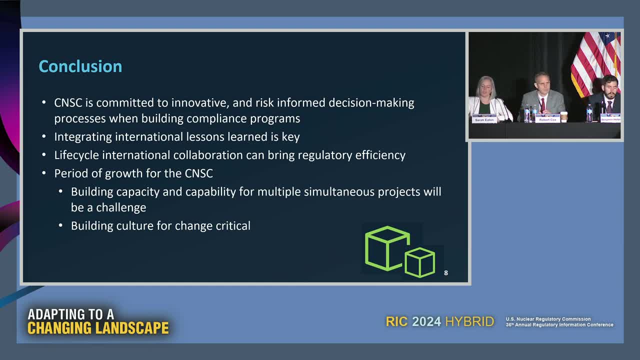 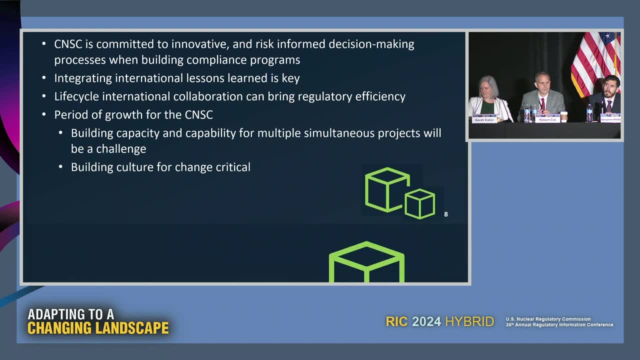 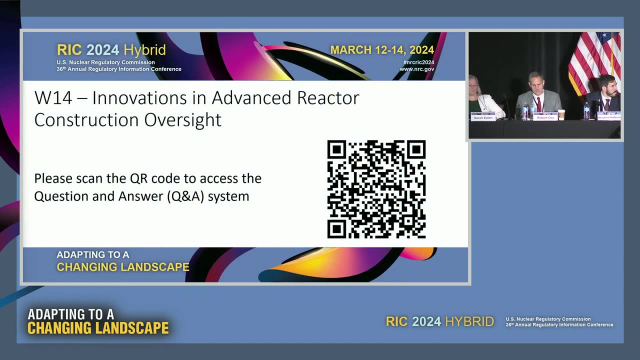 construction, whether it's for international collaboration or indigenous nations, building relationships, indigenous nations and communities. but i know that we are up for the challenge. i know we're well placed to do so, so thank you very much. thank you so. thank you, sarah, and happy birthday. and your present will be that we will not sing a happy birthday to you at this time. 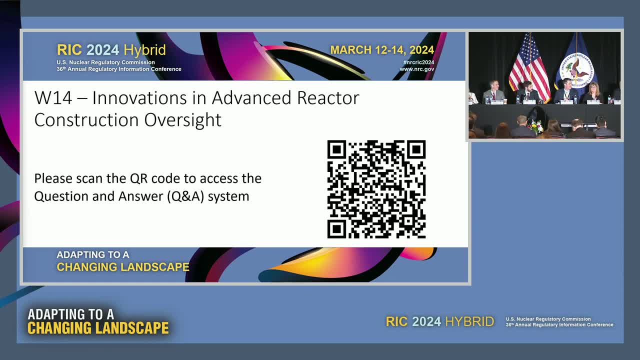 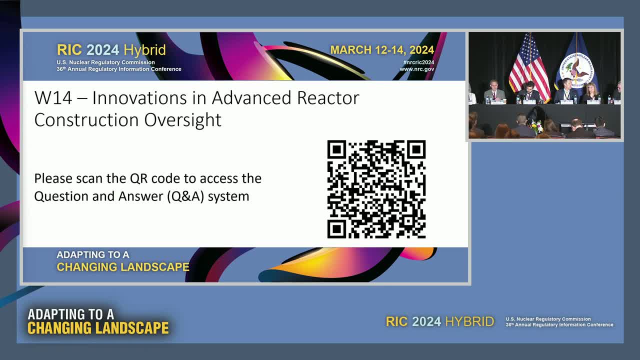 and many other countries that nuclear deployment is a global activity. now It's not just a national activity, And the more we collaborate on efforts such as these, the more we can harmonize and enable the safe deployment of some of these technologies as we go forward. 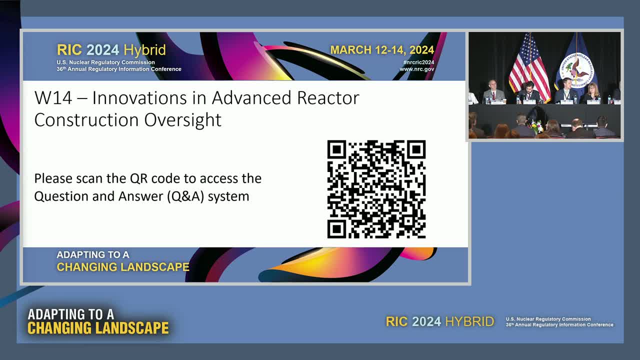 So I do wanna thank the audience. We're gonna move into Q&A. We have a number of questions already from the audience. We have 31 minutes left, so that is wonderful. I wanna thank my panelists for moving through their presentation so efficiently. 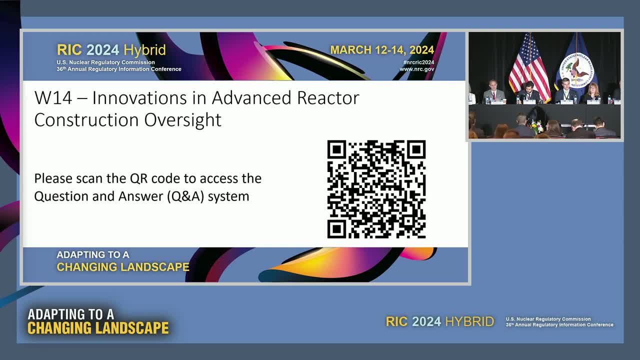 And that'll give us plenty of time to answer some questions. So if you have questions, we're gonna have some time in here, so please put them in based on the presentations you've heard, and we'll hopefully get to a number of these. 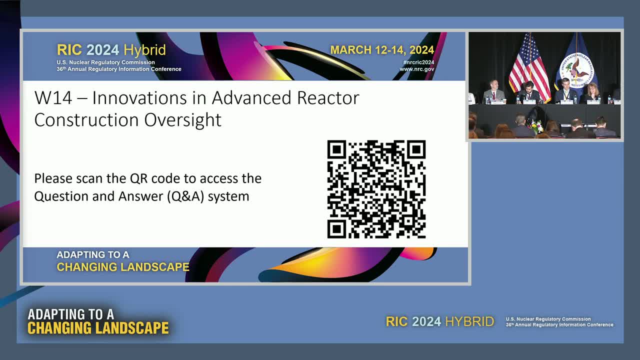 So the first one- and I think I'll send this one to my NRC colleagues and to Ben- is an important one, And it highlights a difference with what the type of technology we'll see and the type of construction we'll see going forward. 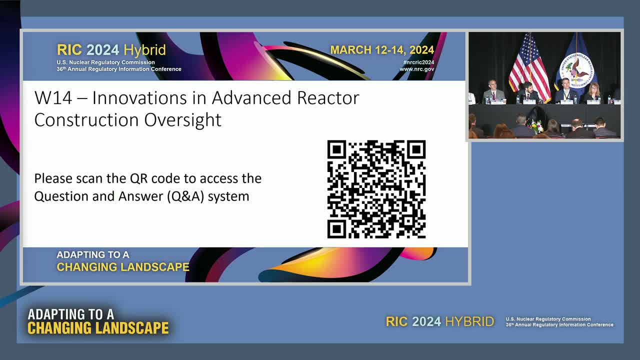 So, as the industry is moving to true modular factory-built applications approaches, how is the NRC preparing for oversight, NSE industry preparing for oversight of the modular fabrication activities completed in a central factory? Nicole John, you wanna start? 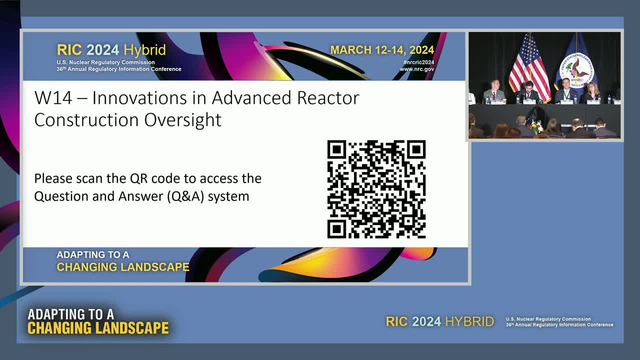 and then Ben can chime in. Sure, I'll take that It's a really good question. It does present a bit of a challenge, as Ben kind of alluded- mentioned in his discussion Our past practice, our past experience. 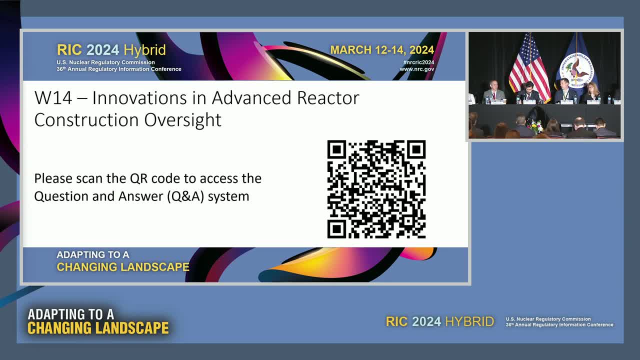 was really stick-built designs. Everything was happening under the auspices or the oversight of a licensee at a particular site. We've always inspected vendors that provide components or maybe small systems, but the bulk of the activity was done at the site and the new landscape. 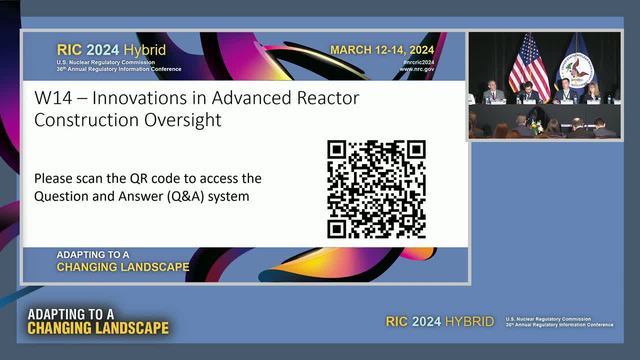 really presents a different challenge. There are a lot of similarities to how being able to inspect off-site, but being able to do it in a way that we're inspecting the right things at the right time, so that we're not you know. 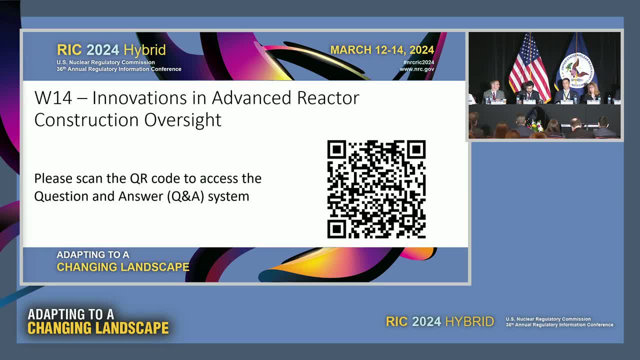 not in a position where we're just inspecting everything right. that's not where we wanna be in a risk-informed and performance-based framework. So one of the things I talked about was looking at kind of an integrated inspection scoping matrix. 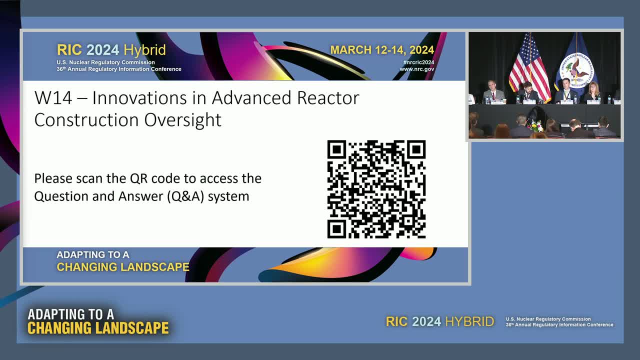 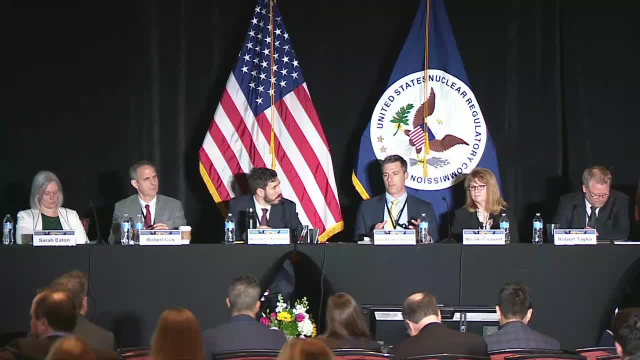 where you look at the project and you say: what are the, you know, based on this design that a licensee or an applicant has submitted? what are important things? what can I leverage from what I know? you know, a risk-informed process. 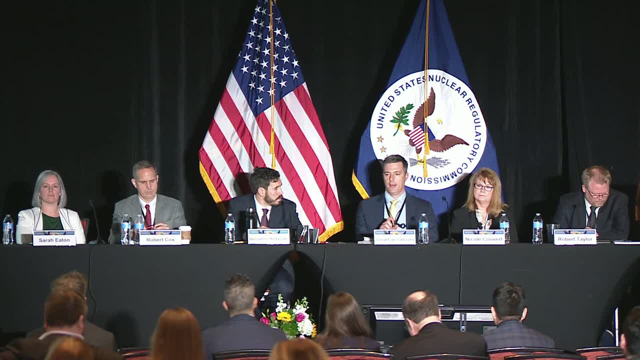 underpinning, risk-informed. Obviously, we talk about likelihood and consequence. Underpinning, that is uncertainty. And so one of the things with modular construction, especially as you go from a first-of-a-kind build, through second, third, through nth-of-a-kind- 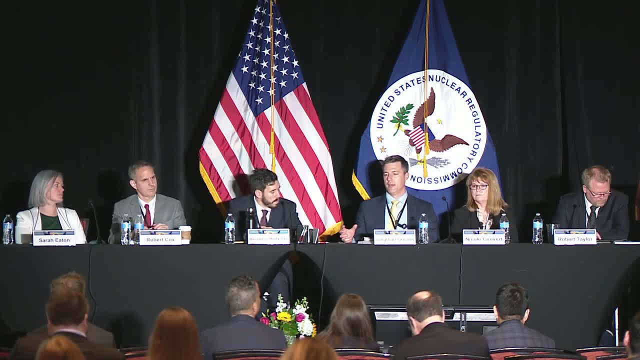 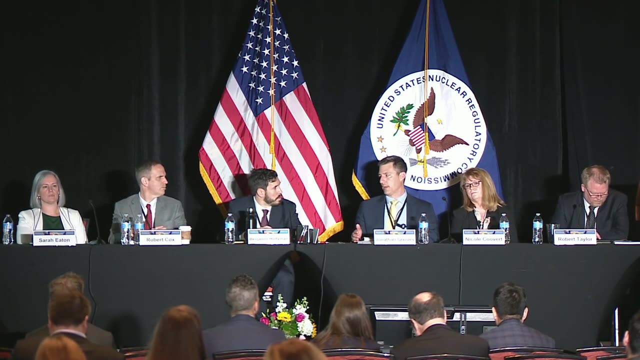 is, you learn a tremendous amount of information And we have to have a system that is able to factor that information in, certainly if the industry gets to a deployment schedule that Ben talked about, where you know dozens of reactors are being constructed in a year. we need to be able to leverage that experience. 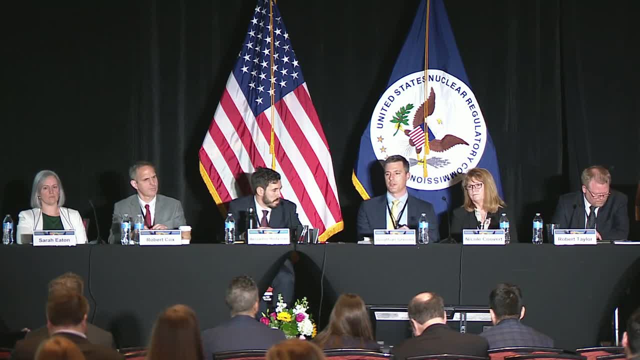 so that we aren't necessarily performing the same level of inspection for each one of those units and we're learning as we go along and scaling ourselves appropriately. So it presents a challenge. We are thinking about that, One of the best parts of getting into where we're at now. 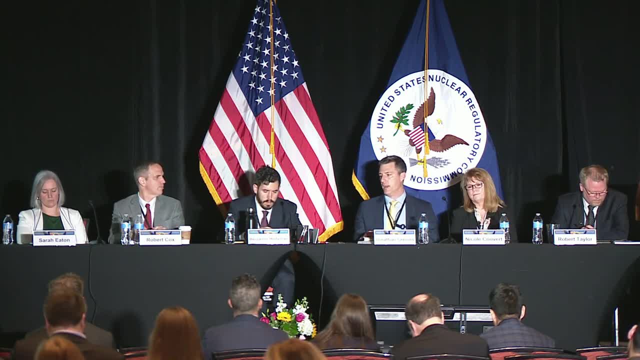 where we're starting to engage through workshops is being able to learn about the different deployment models that some of the vendors are, you know, contemplating, so that we can make sure that our system is flexible enough to adapt to any of those realities. So it's really an exciting time. 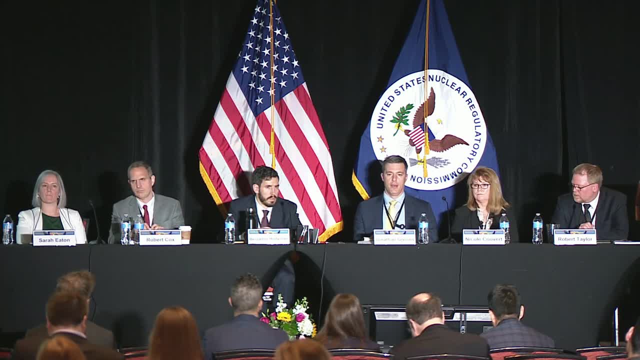 We are thinking very hard about that to make sure we come up with a program that will ultimately address it. But we look forward to continued engagement with you know, NEI, as well as any of the vendors, to make sure whatever we're coming up with. 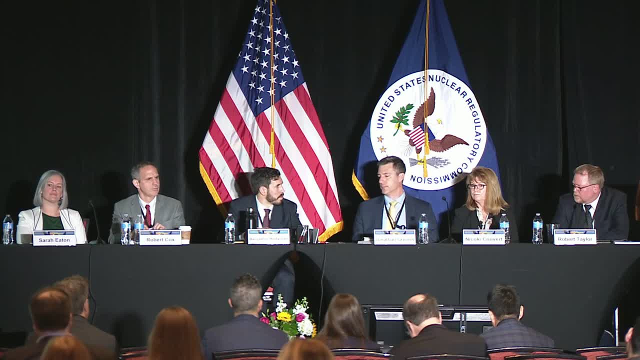 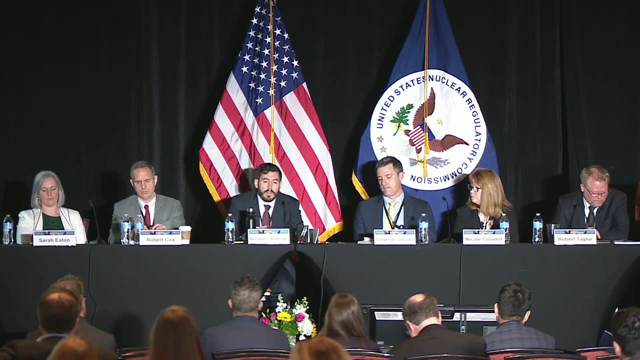 does satisfy the landscape that's ultimately going to come. Yeah, so just to add to that, I appreciate the initial comments and I think it's a good question. The challenge, of course, is that the devil will always be in the details. 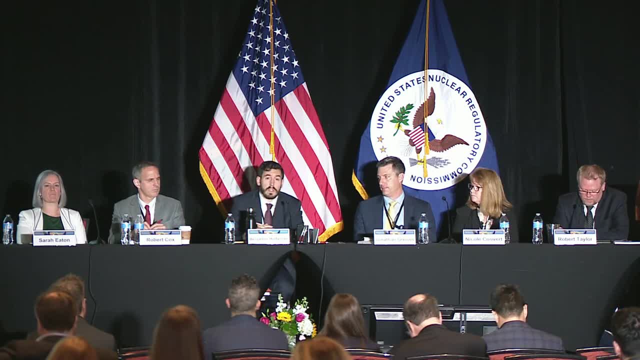 And so I can't come here and say, well, clearly, we're going to do X, Y, Z and that's going to work for every possible iteration that we're going to come up with. But I think the right framework, or the way that we're thinking about this, is right. 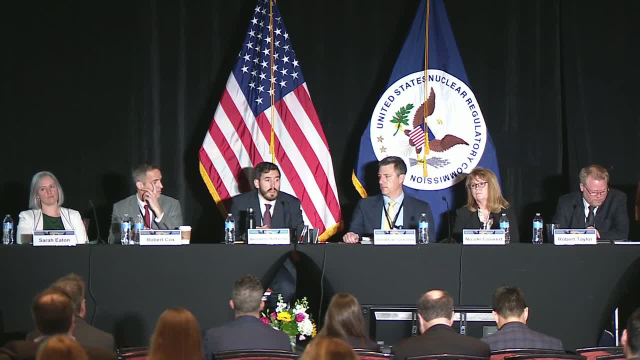 in the sense of as we're moving activities away from site. clearly, we don't want to be doing the same activities in terms of in terms of oversight and inspection, both at where this is being manufactured and then again at the site, But, depending on what we're building, 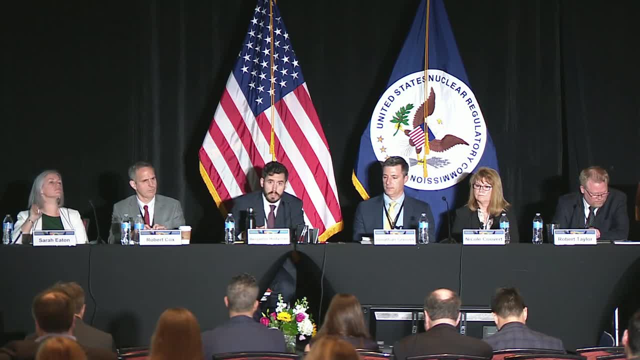 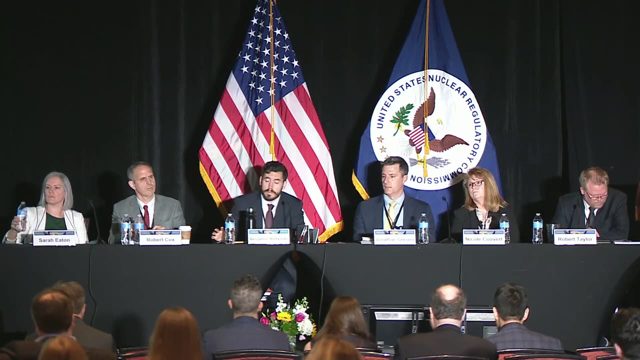 how we're building it, how accessible is it going to be after shipment? those are all going to impact when and where you can actually do the oversight most effectively. Now, of course, let's just say that on the most extreme case, it's a microreactor. it's all sealed up at the factory. 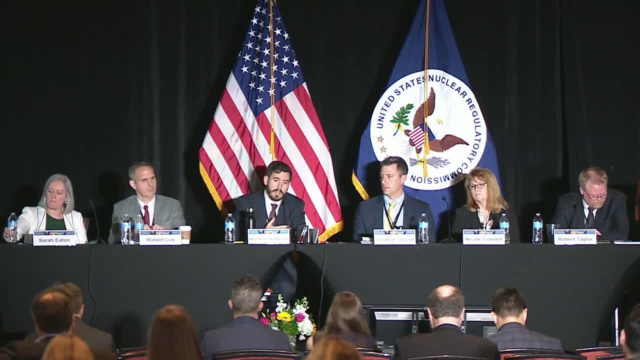 You do your inspections and oversight there. When it shuts down, when it shows up at site, there's still probably something that we have to do in order to ensure that it was received and is still in the right condition for operation once it gets there. 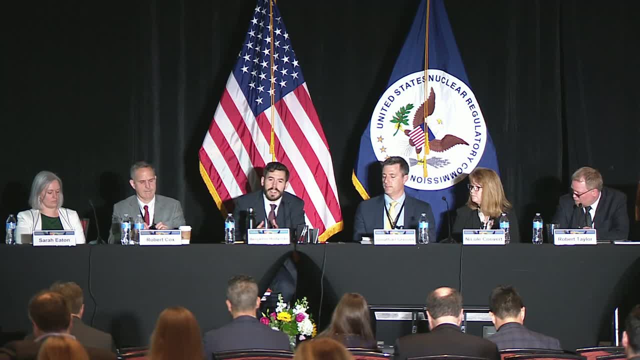 What does that look like exactly? We're working on that right. It's clear that you don't want to have a one-to-one recheck of everything, but it's also clear that you should do something to reassure that you have a reasonable assurance. 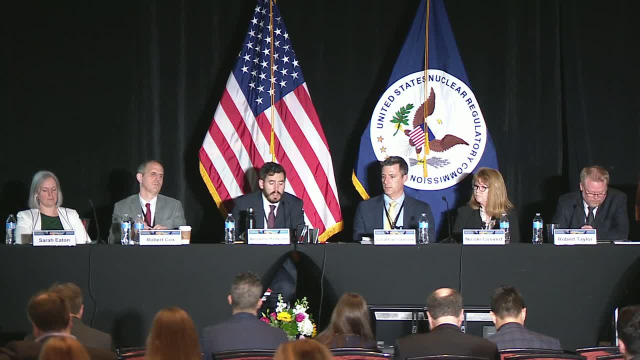 that it's going to operate and work as we think it is And I think, as we, as Jonathan was mentioning, as you start going forward and we figure out exactly what the process and what some of these deployment scenarios actually look like, we'll have more details. 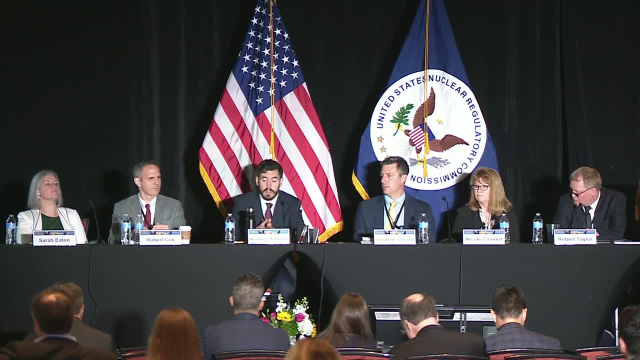 But I think, at the same time as we start laying out- here's what the strategy for this deployment actually looks like, the different designs and technologies we'll enable ourselves to kind of come up with, here is how this flexible framework is going to be enacted. 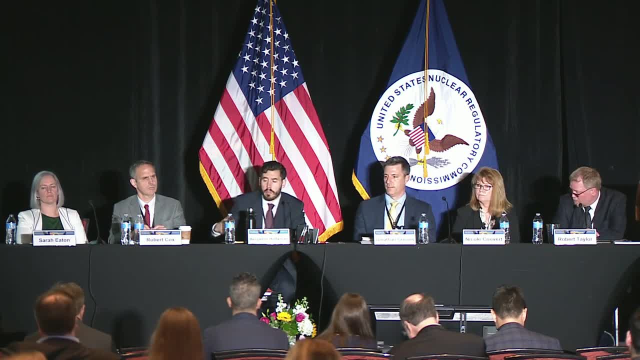 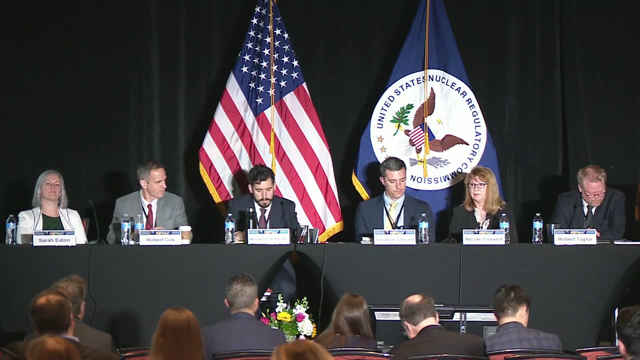 for this design, for this deployment, For this application, And then we'll be able to apply and move that forward consistently. for that design, Thank you. The only thing I would add to that is: so some of these concepts are not new to the NRC. 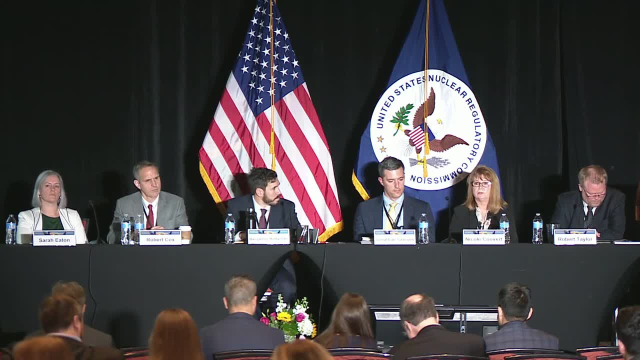 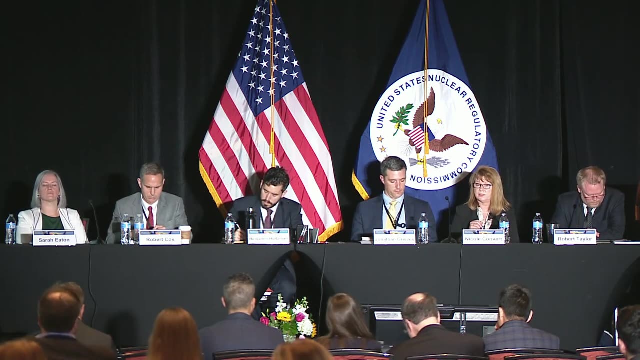 You know we have inspected modularization, We have looked at vendors, We have looked at factory acceptance testing. So some of these concepts are new, but applying them more globally across more, you know different technologies more consistently over a number of different sites. 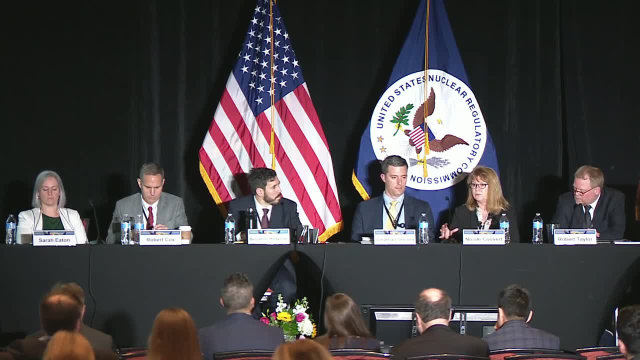 or facilities. that's where we have to be innovative And that's where our framework is looking at. How do we be scalable, technology neutral? But you know we're going to continue to use the lessons we've learned from the past. 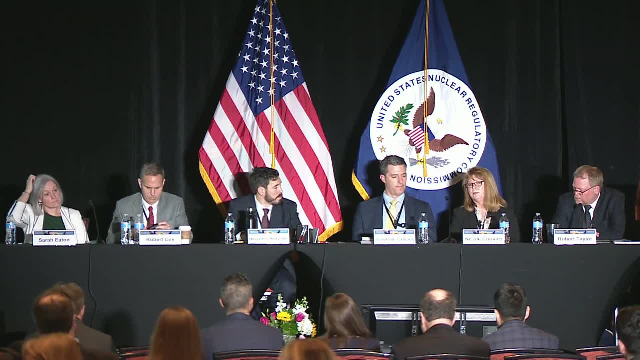 to apply it through the future. So modularization is a complex issue that we saw from both the regulatory side and then from the industry side. So there's learning, There's learning to be happening from all perspectives for you know, for the future of this, if it's going. 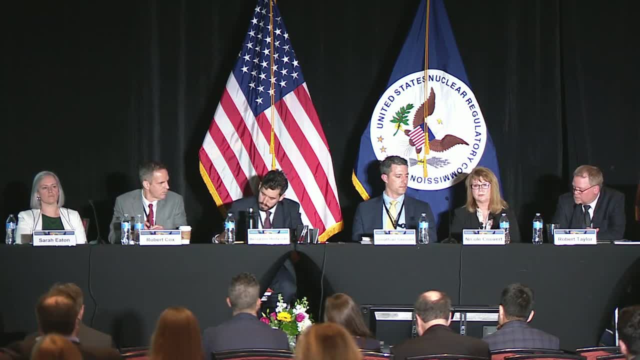 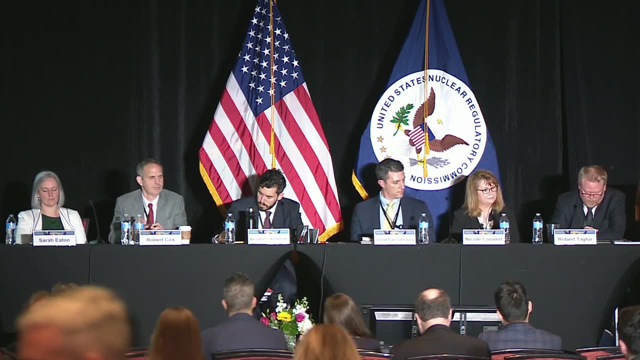 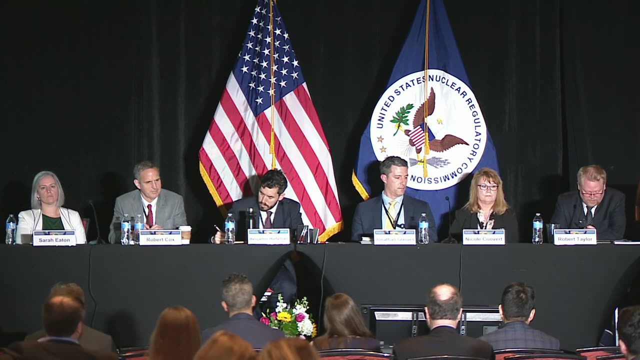 to be primarily focused in that area of construction. Thank you, Thanks. This next one. I'm going to start with Robert, Recognizing that we're looking at risk informed and performance based approaches, I'm going to specifically target this question towards the technology. 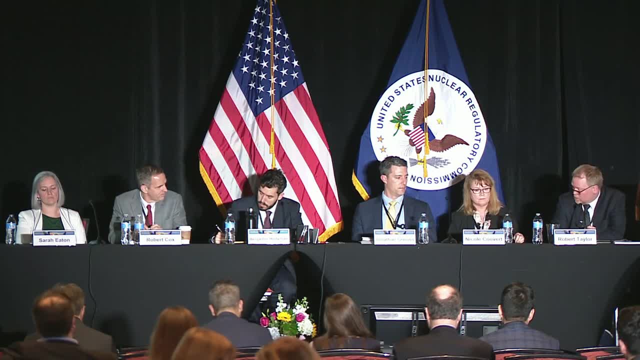 How can it be? how can the technology really benefit us in terms of cost and safety? How can it help us in terms of you know? how can it help us in terms of scheduling efficiencies for the construction of these facilities? Where do you see the biggest impacts being? 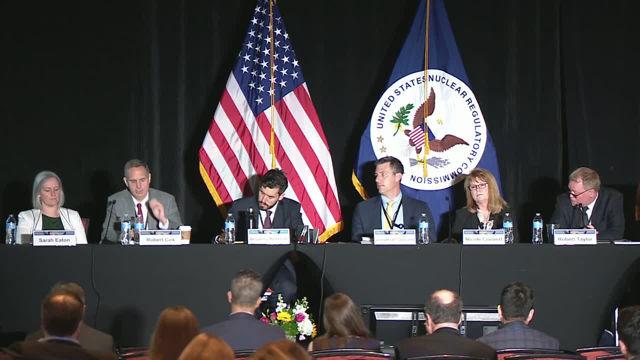 Sure, Yeah, It's a great question. I think one of the areas that we've, you know, looked at is ultimately like, as an example, we talked about these modules as they move through from the factory to the site. You know, one of the areas that we look at first of all. 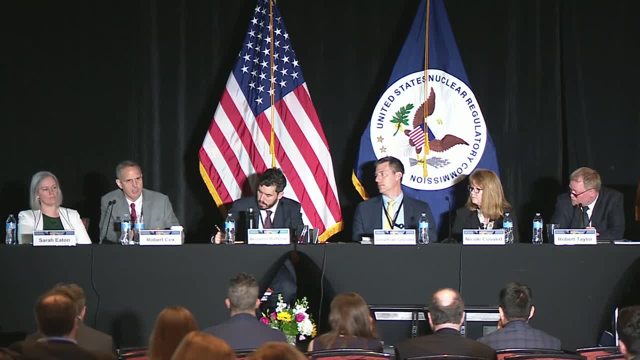 is just better document management And, if you look back at sort of past experience, all of the issues associated with being able to just again, just from a construction perspective, being able to track where is all of the information about all of the modules and whatnot? 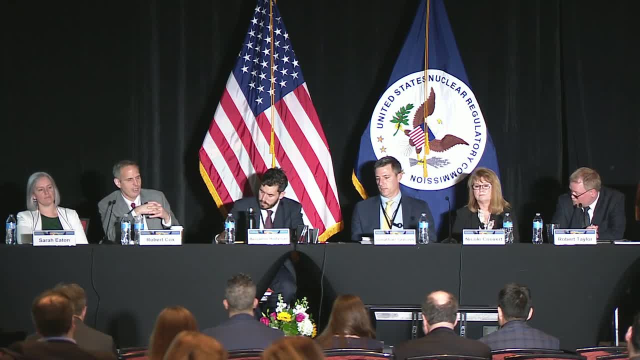 But we'd be able to leverage the technology to be, you know, scan a code on the side of the module to be able to pull up on a tablet all the documentation that you would need associated with that. So document turnover becomes better managed, for instance, 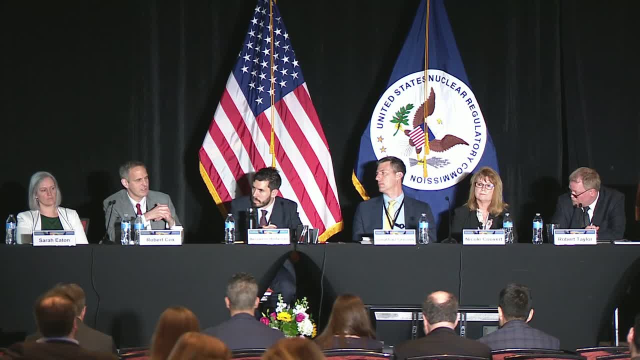 which is one of the things that's been noted as really slowing down a lot of processes in a lot of ways. You know. the other example would be- you know that I kind of you know always go back to- is things like you know. 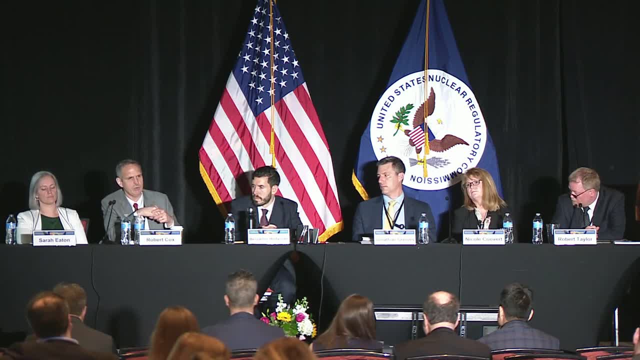 tolerance management, as you're placing, you know, modules You can begin to. you know better be able to track if something's been misplaced, what's the impact on that, And so if you have a nonconformance, you know. 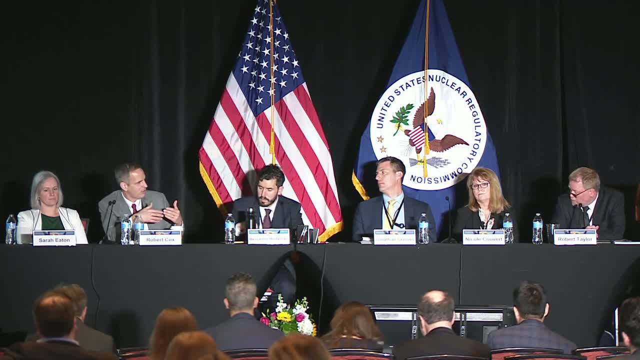 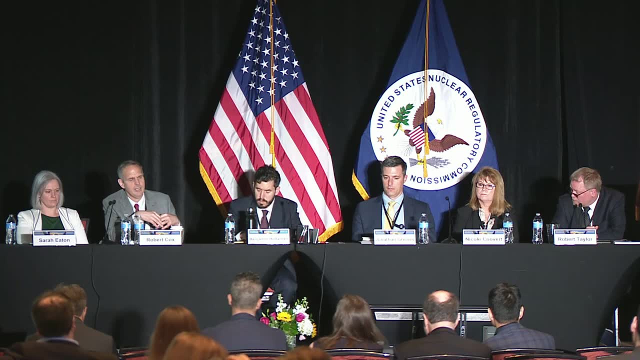 and you have to go back through and do analysis and disposition. you know the significance of that. you should be able to do a lot of that analysis a lot more rapidly And that's one of the big advantages that we see. The other element: 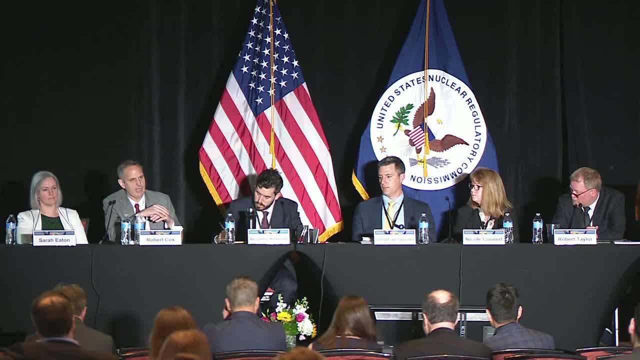 that we look for ultimately is- you know, I didn't talk about it a whole lot here- but leveraging sensor data on site. You know, for instance, one of the things that we're going to, that you have a lot of issues with. 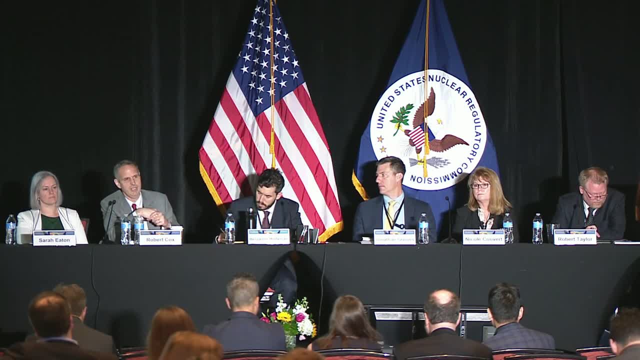 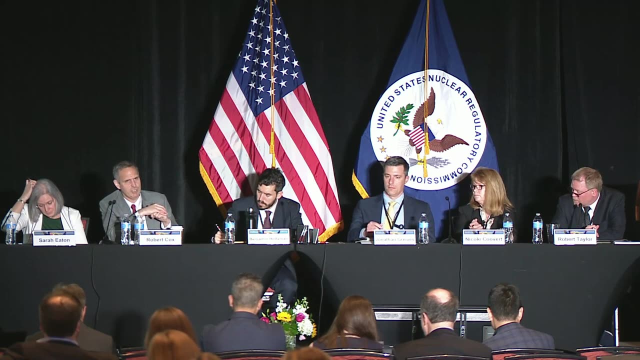 if we have underground shafts, for instance, how do we leverage sensor data to be able to sort of track what's happening throughout construction? And that's something that you know we're working on testing right now, But that's. there's a lot of opportunities to be able. 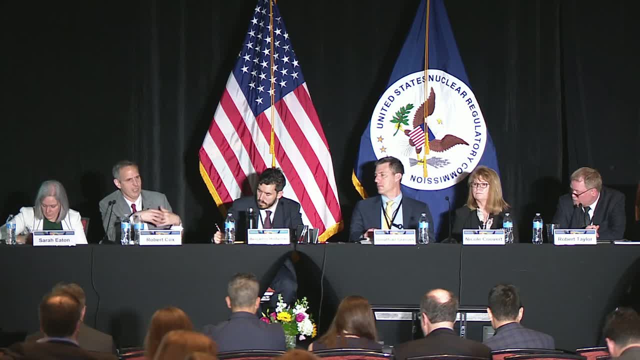 to use data to sort of, you know, to speed up a lot of the aspects of, say, underground inspection and the geotechnical side of the build. So you know, it really is a matter of being able to sort of. 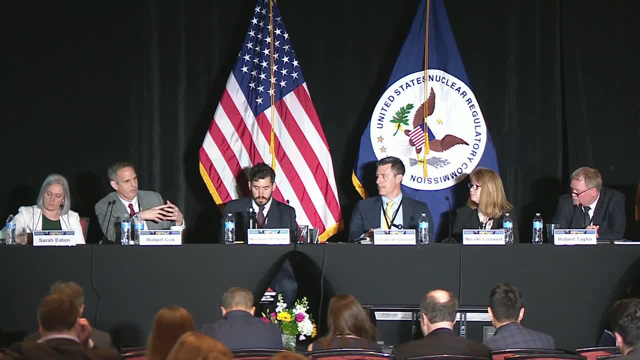 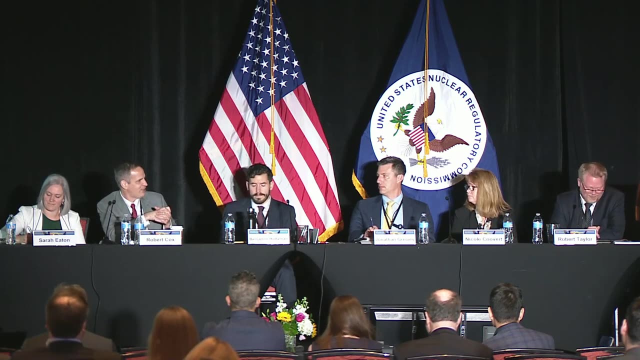 I think we talk about leveraging the modularity, but you know how do we begin to sort of better track the information, use the ability to track it and use sensor data with an understanding that sensor data needs itself to be trusted and validated on a regular basis. 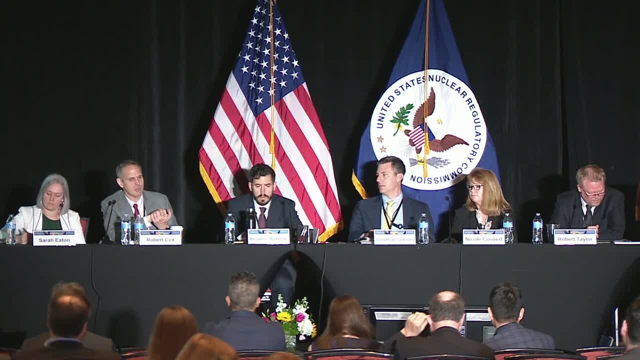 So those are where a lot of the questions lie, I think, But there's a significant opportunity, I think, to begin to, in particular, look at the notion of if something happens in the process, in the construction process, how do you do a much quicker analysis? 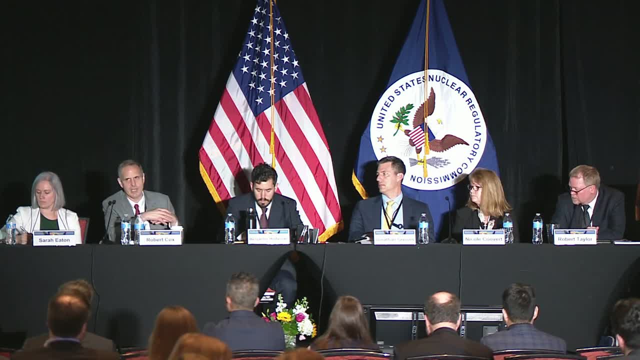 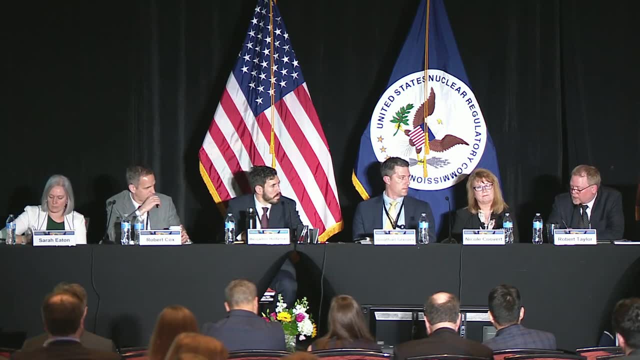 of what the issues may be associated with that and how do you better control document management turnover? Thank you for that, Robert. Greatly appreciate it. Maybe to the panel if we're a few years from now and we've implemented these activities. 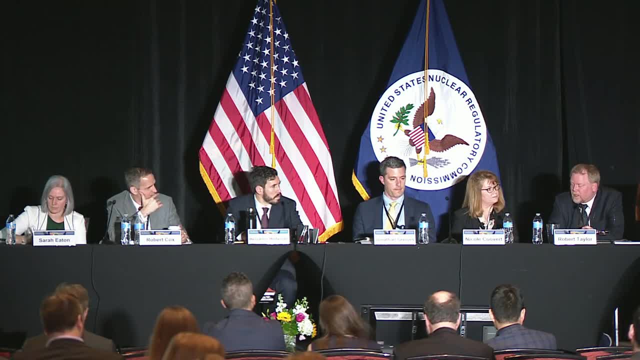 and we talked a little bit about assessment throughout the effort. what is your measuring stick for whether you'll know whether we've been successful in developing a program and one that works the way we envision it? And maybe I'll start with Ben and ask him to define success. 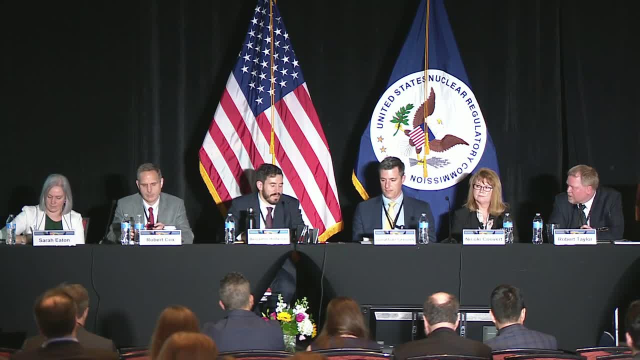 for this at the end of the day and then ask other panelists to weigh in. That's what I get for making eye contact, right? Yeah, yeah, yeah, Yeah. so I think it's a good question. I mean, where we are today, we can look at what is the oversight. 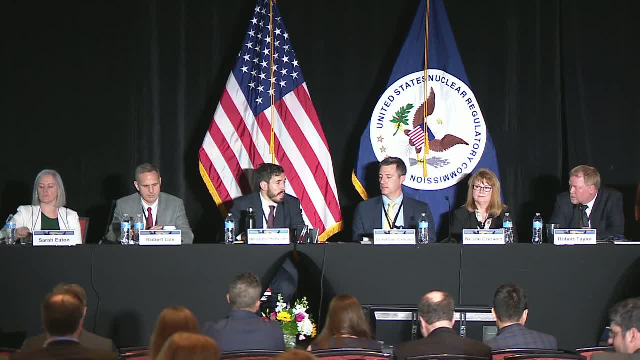 and program. look like for Vogel, for example- And Vogel was, I think, five inspectors and several thousand hours worth of work- And if we say, okay, we've developed this program and you know what, that's where we are. 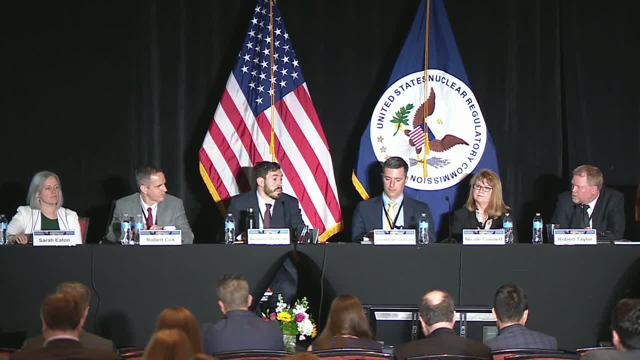 We have no measurable gain. Well, clearly that was a problem. We didn't succeed at that one, We didn't assess, We didn't assess and implement a risk-informed process. I think, if we can look at it and we say, yeah, this. 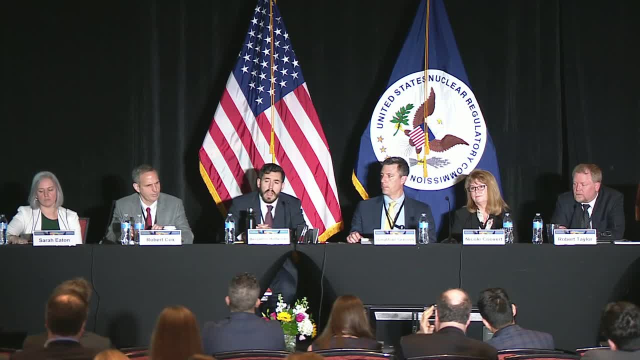 we can see how designs that have less risk of public health and safety have less oversight associated with them. we were accessing this in the right framework. One thing I think that we would want to see in this program is the differentiation of protection of public health and safety versus the protection. 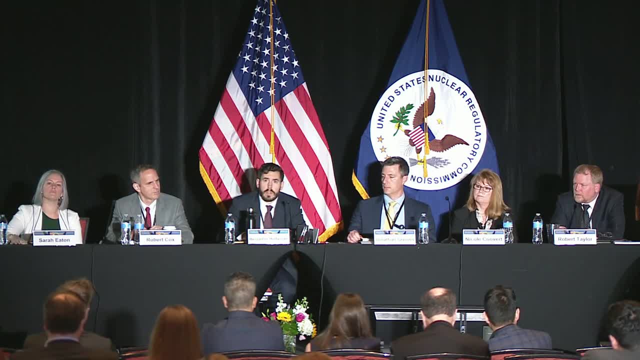 of the asset itself. There is a difference right between having saying that we have a design and if we turn it on there's a problem and we're going to have a radiation release or some dose or something that's going. 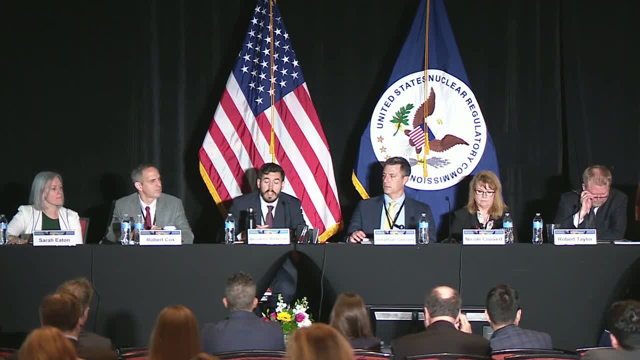 to go wrong and saying, well, you've destroyed your asset, It's not actually going to be able to operate, But there's no real risk to anyone, It's just you're not going to make any money. I think figuring out how to differentiate. 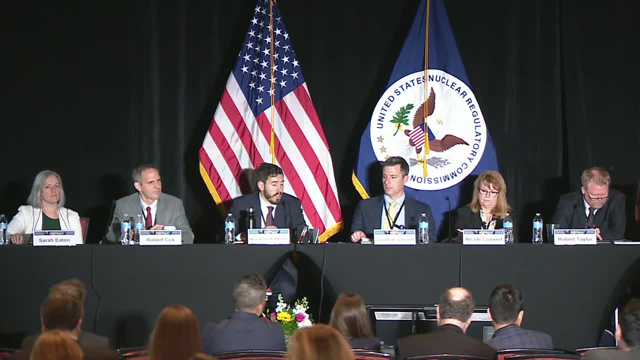 and specifically target. you know how do we ensure the? the adequate protection of public health And safety for will be a key enabler of whether or not we have a successful program. Great Others on the panel Want to weigh in. 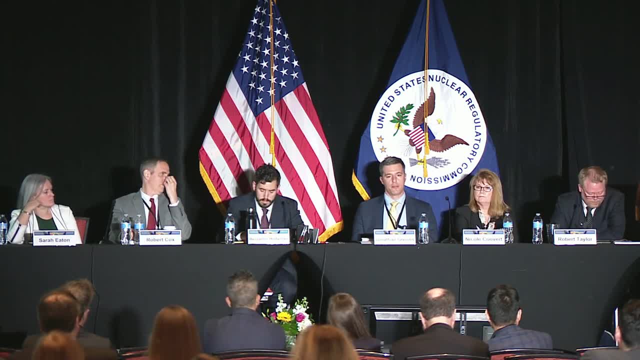 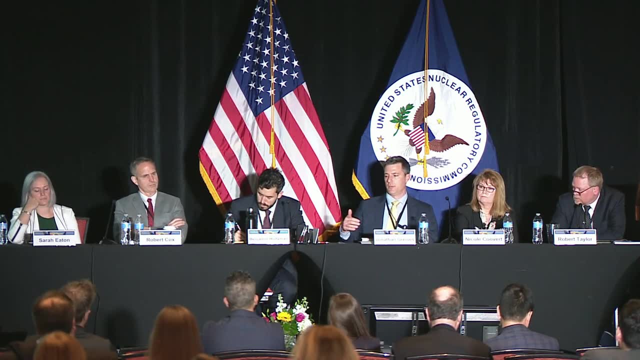 So maybe I would add: you know when we're designing the program. typically, when you think about an oversight program, you come up with: okay, here are a list of inspection procedures we're going to execute and we're going to do an X number of samples. 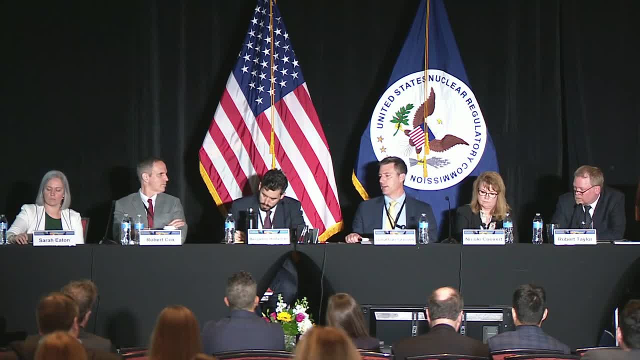 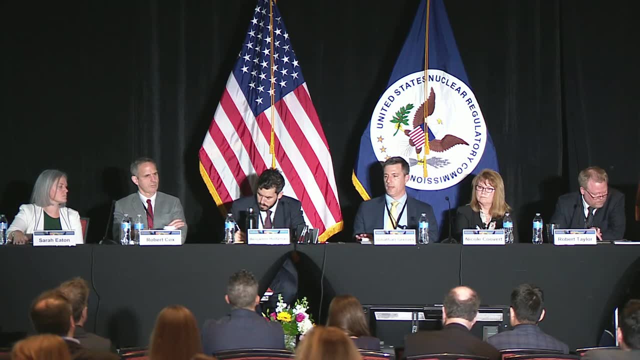 and that's going to result in X number of hours of inspection. What we're designing, I think, is a little bit different because maybe you know, complementing what Ben just said, each of these designs is going to present a different risk profile, a different level. 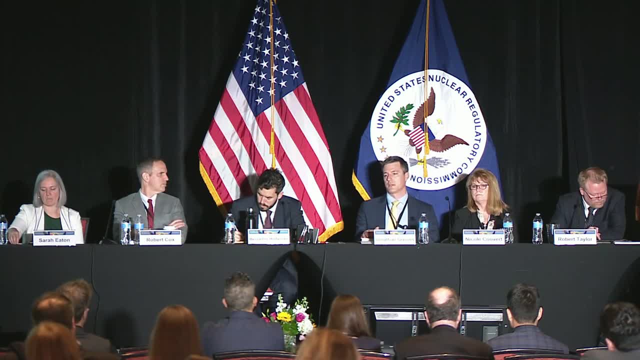 of complexity- passive versus active systems, number of systems, number of ITACs. So we need to design a decision-making process that stands up to the rigor, so that when we receive a new design, a new application or a new, you know. 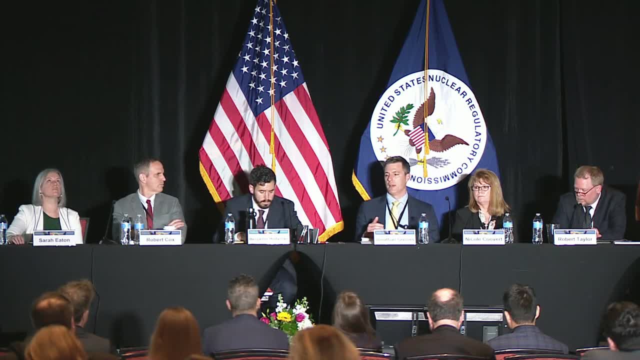 design, certification, new, you know, manufacturing license, that we can implement that decision-making process. engage with the applicant to make sure that whatever oversight framework looks like for that particular design, that it's right-sized to that design and appropriate to the circumstances and withholds. 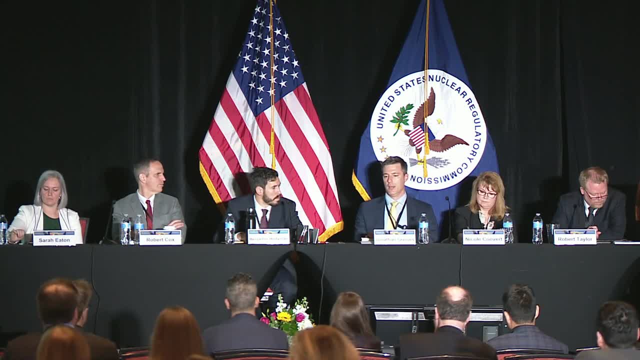 you know, holds up to the scrutiny that it should. So I think that's where, you know. success for me is we've developed a decision-making process so that we can right-size, develop a scaled inspection footprint and we have the appropriate decision-making. 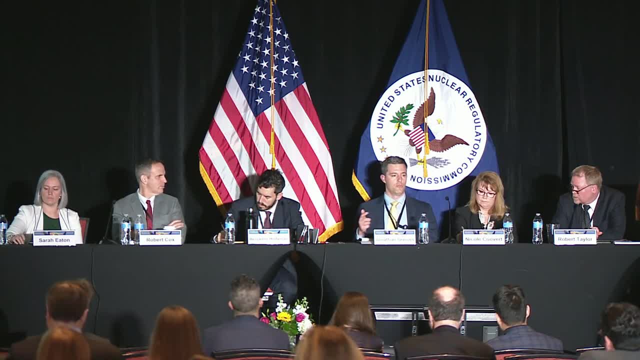 processes that we need. Thank you, And that's what we're trying to do is we're trying to build a system that's consistent with the principles of good regulation So that we can continue to evolve that inspection plan for future builds and consistent with those principles. 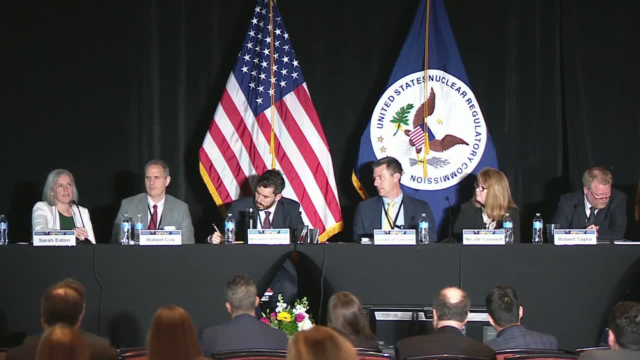 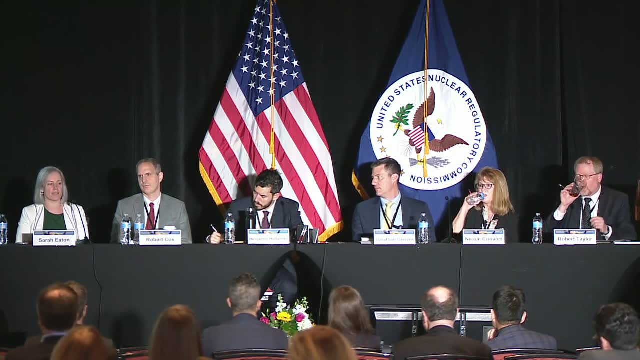 and our principles of good regulation. I think that would be success for us. Sarah, you want to weigh in? Thanks. I think I'm going to define my success a little differently, And I think it's because we have a scenario where we could have constructions at this site. 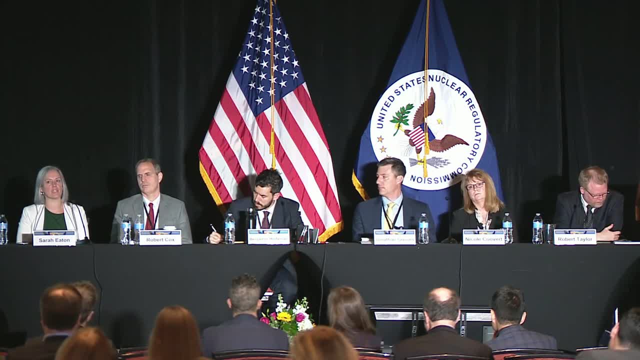 in Canada starting in 2025. And so, from our perspective, we would look at the early measures of success was: was the project able to be executed correctly, you know, safely, according to timeline and schedule? Were we able to do the inspections that we needed? 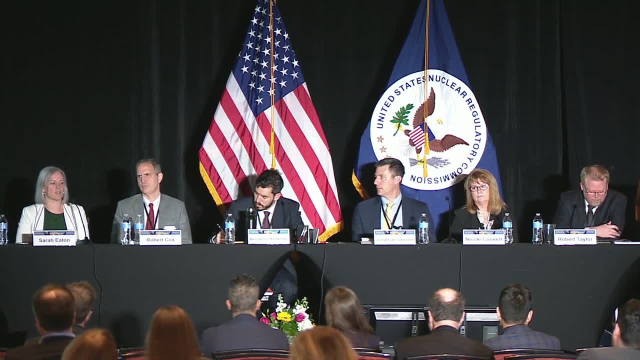 Did we get the information we had we needed And then to do an assessment after that to say, okay, what would we need to do for the same unit, You know, if there was to be unit two, unit three or this unit in another location to be able to look? 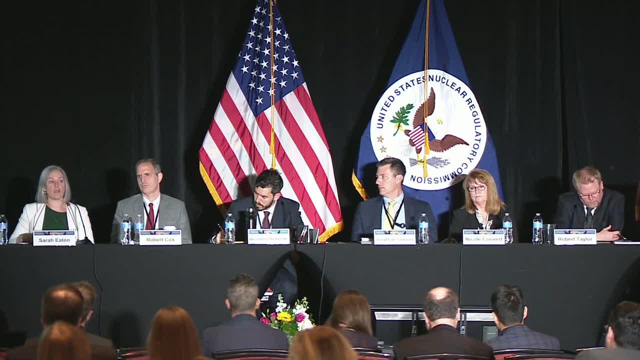 at it that aspect. I think it's important that we can plan for every possible scenario, but we need to execute on the one in front of us, And so we certainly are focused on executing on the one in front of us, while acknowledging 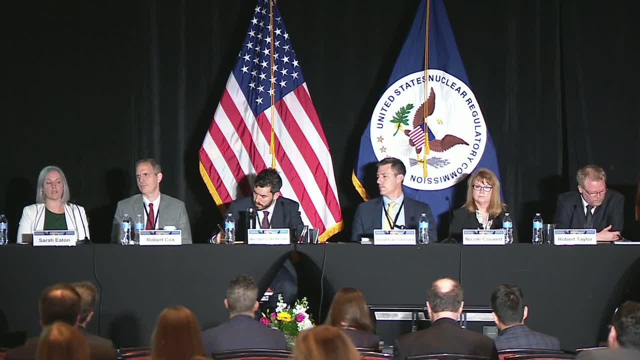 that there's definitely work to be done. There's so many interesting deployment scenarios And I think Ben's part about the models is totally true. Who knows what's going to happen? But for the ones that we have in front of us, we have to focus our energies to make sure. 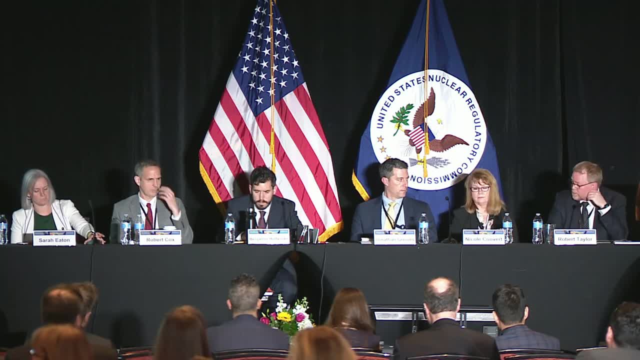 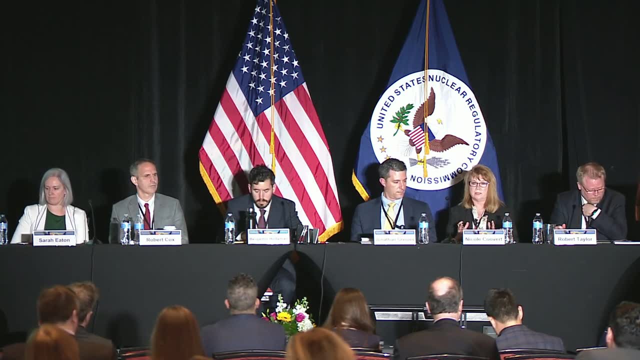 that we're doing those right. Thank you. If I can add one thing, Sure, please. So what I would note is: you know from the NRC's mission statement, you know our success measure is public health and safety. 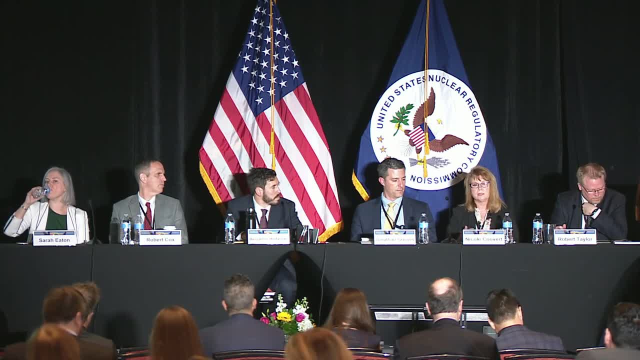 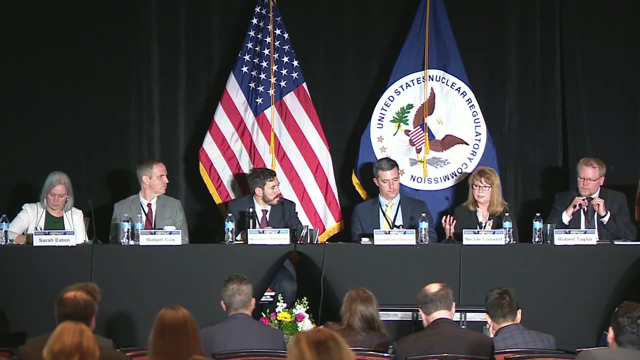 Protection of the environment and security of these facilities. There are some challenges out there that. what does that look like with these new- and they're questions, They're not necessarily challenges, but the actions that we have to work through- What does it look like for a potential mobile reactor? 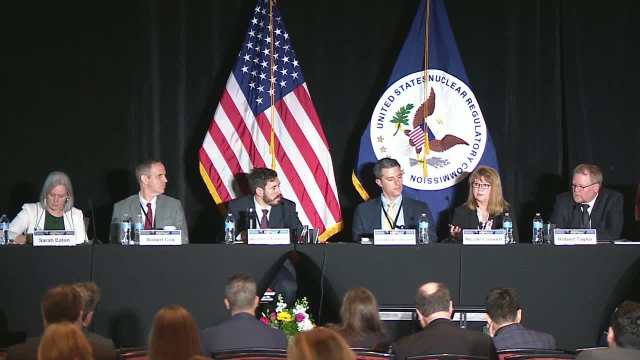 What does it look like for the environment? What does it look like for protection of public health and safety? So you know, to me, the success measure is that the regulatory decisions and the licensing and inspection oversight that's done provides reasonable assurance, while continuing. 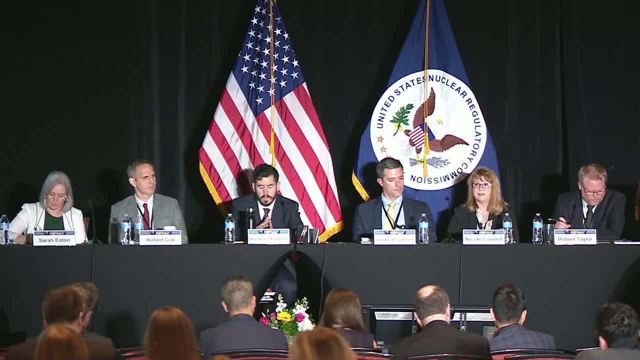 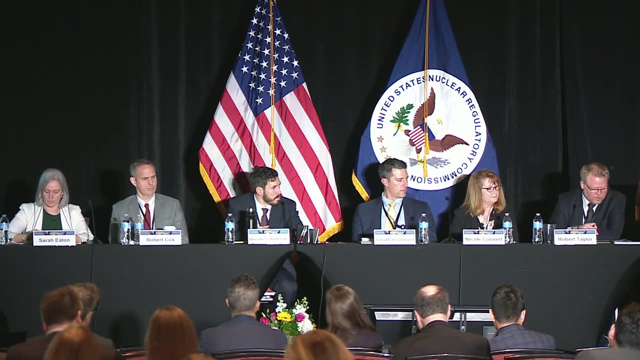 to make our mission And there's because there's new questions in the future. we don't know what those needs do, And working through that is going to be of the highest importance. Thanks, So John was touching on something that I think is important to follow up. 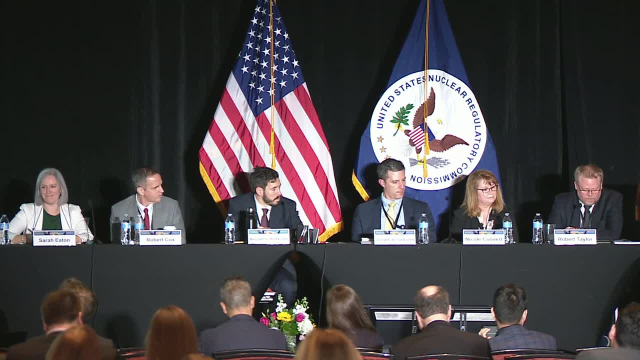 And we had a good question here from somebody. Maybe it would be good for the panel to elaborate on their vision related to this. So, considering the huge design differences between advanced reactor designs, will there be separate R-COP guidance for each type of reactor or will the guidance be so general? 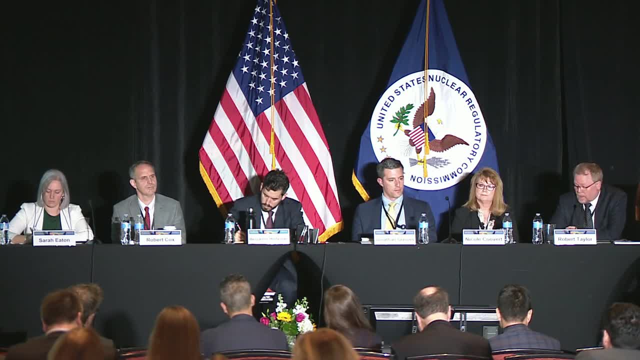 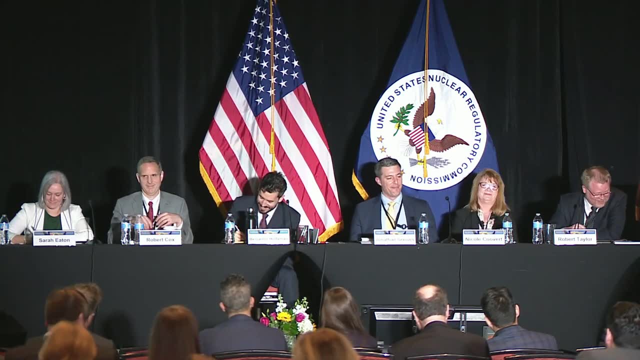 as to potentially not be useful. It's an honest question. It's an honest question, It's a fair question. So I think you know. so I'll point to two things. So one of the things when we're developing or thinking, 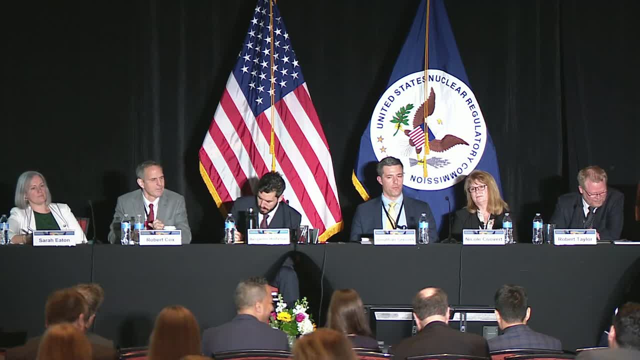 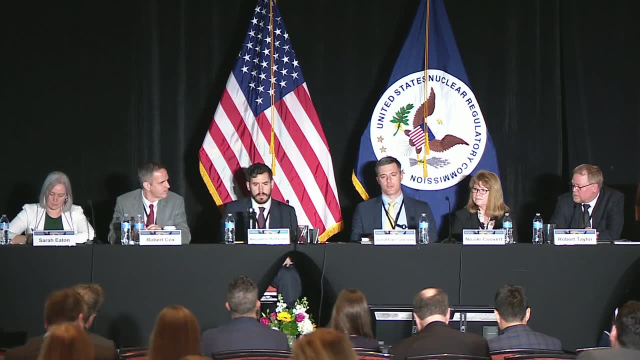 about a technology-inclusive framework. we really need to think about what's common across all the designs, And there are some things that are common, So certainly what systems, structures and components are used to satisfy- And I talked about the fundamental safety functions. 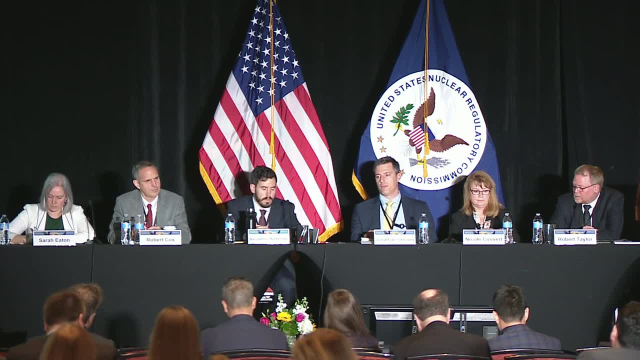 Each designer is going to, you know, use their or develop their design to ensure that they control reactivity, remove the heat, remove, you know that's generated, and they control radionuclides. But then, underpinning all of that that I mentioned was 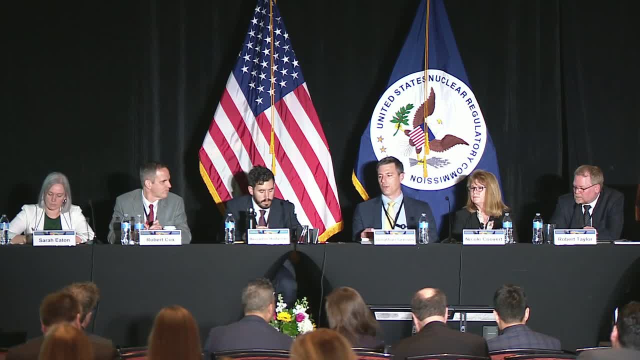 every designer, as they go through construction, is going to need to implement quality assurance program attributes, And so if we're inspecting and looking at how they're building their SSCs, but really what we're looking at is how are they implementing their quality assurance? 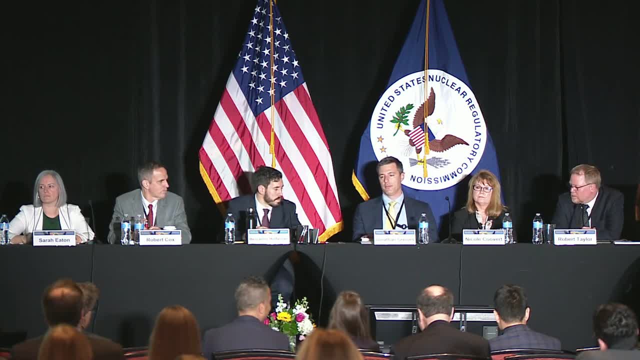 programs and then can use that level of inspection to draw conclusions about things that we're not there for. Right, We do a sampling-based inspection program. We're not going to look at every single component that's constructed, But they're using the same processes, procedures. 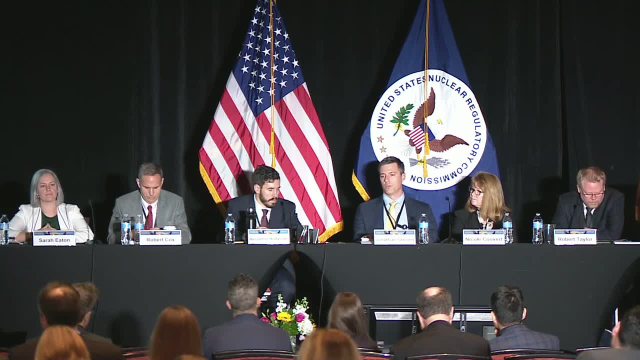 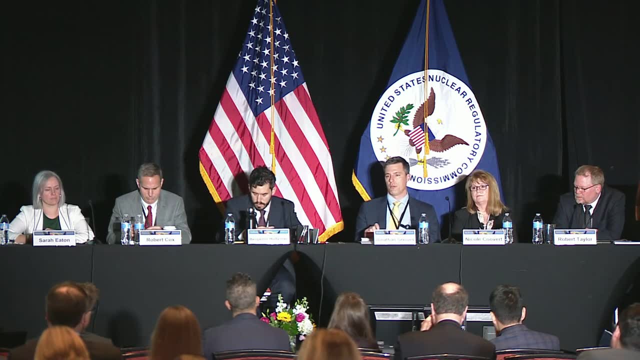 and programs to affect the results that they're looking for. So I think that's a common. you know, regardless of technology, you know quality assurance programs. they'll define what that is and that'll be approved in their application. But that's a good basis and generally common. 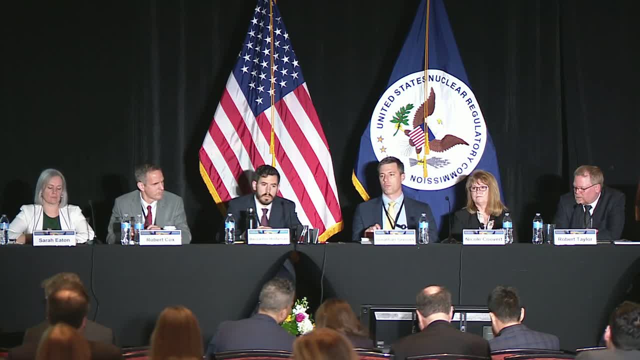 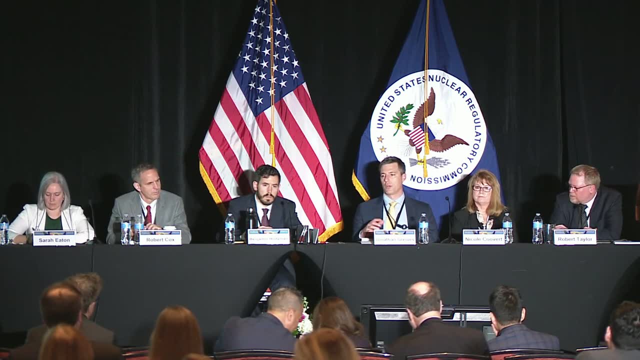 that I think we see. So when we develop inspection guidance, what we would really want to be looking at is: how are they implementing their QA programs and is it resulting in a quality outcome? Is it a quality output? you know, a quality component. 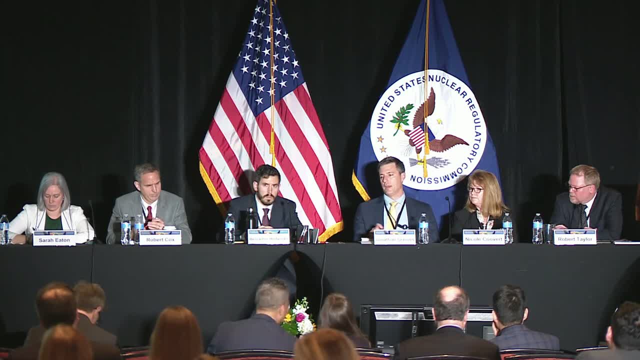 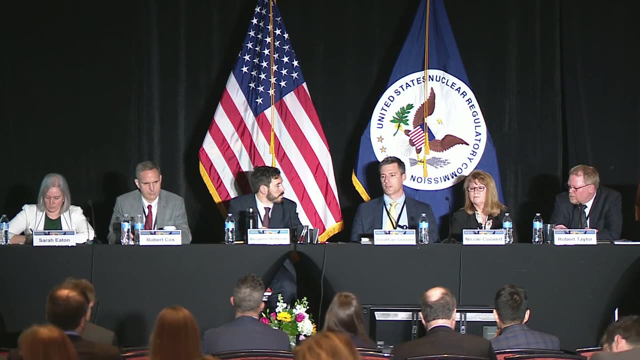 quality system, quality plant, And so if we focus on that, I think we can get some common threads that'll give us good guidance, regardless of design. Certainly, I think there are some different aspects that we'll have to create specialized inspection for Right We may need to look at. you know how you know. 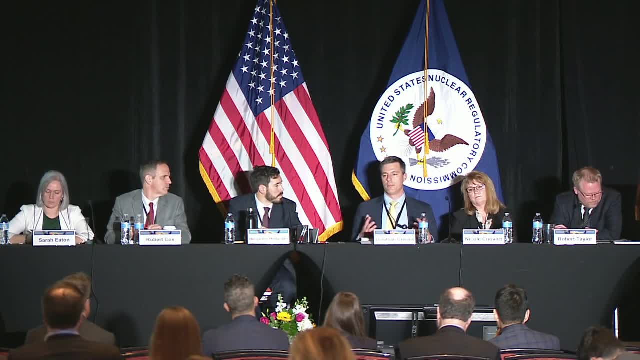 salt content of. you know if it's a molten salt reactor right, there may be some aspects that are specific to that, that may warrant some specific guidance and we can address that on a case-by-case basis. But underpinning that there should be quality assurance. 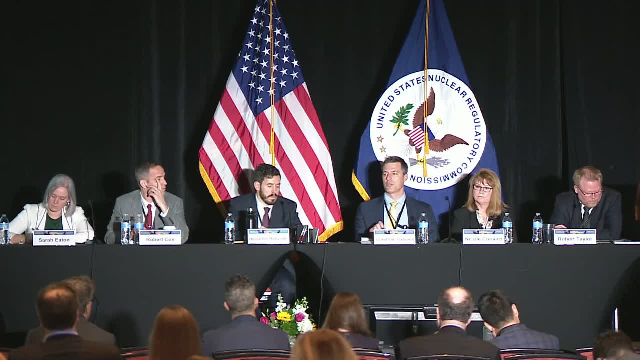 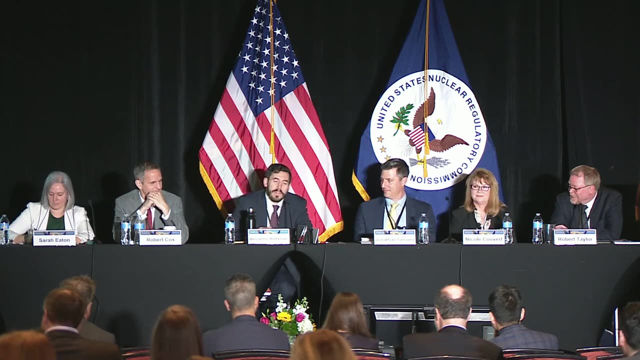 attributes that are ensuring that they're meeting. So it's still largely very similar and then we can look for what specific design differences warrant specific information for our inspectors. So I'm going to do a very dangerous thing and slightly disagree with you And the reason I'm saying. 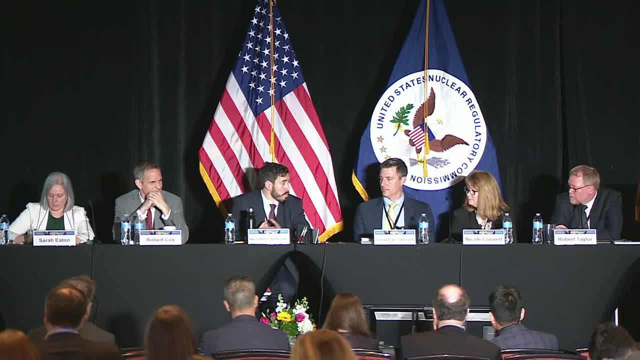 that I want to say. that is, I think the question, which was a very interesting question, is missed, an opportunity for a third choice. Okay, And the third choice I think that we're missing is, you know, when we described the system? 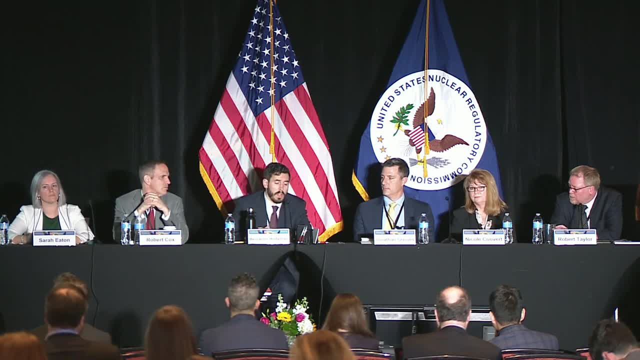 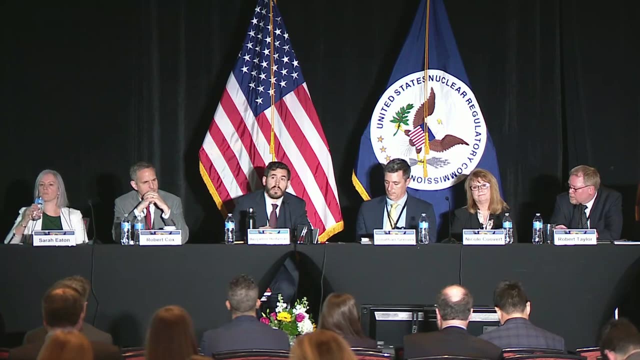 when we described the oversight program of what we're trying to set up here. it is a risk-informed, performance-based, technology-neutral framework And if we set this up correctly, it works for all the different technologies because we we have principles that we apply to that technology. 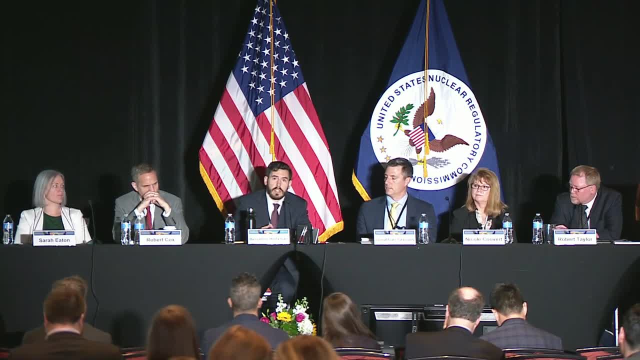 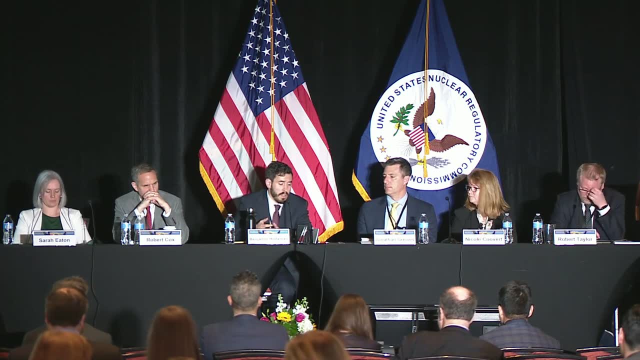 and it yields a different answer depending on what your technology looks like. This is the same process that we've been working with NRC. we industry have been working with NRC on for many years now the licensing modernization project And we've already had several successes already. 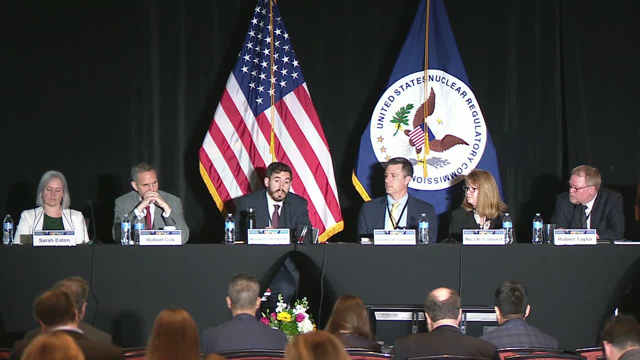 under our belts in the development of different guidance, And industry is using this to develop topical reports, to develop applications, And I think this is just another step in that, using the licensing modernization, technology-neutral, risk-informed, performance-based approach. 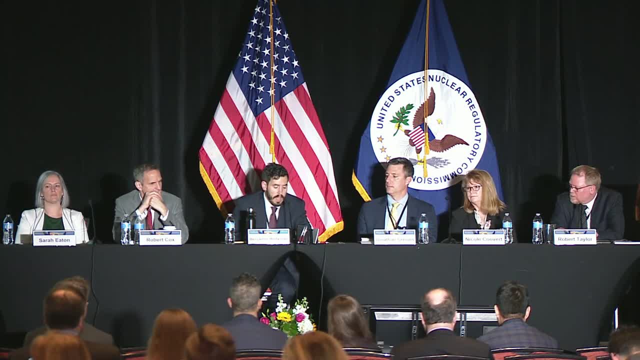 And so I don't necessarily know that we'll need to have specific guidance that will have to be overly prescriptive or something that's so general that we can't use it. I think we build the tools and then the tools will be applied. 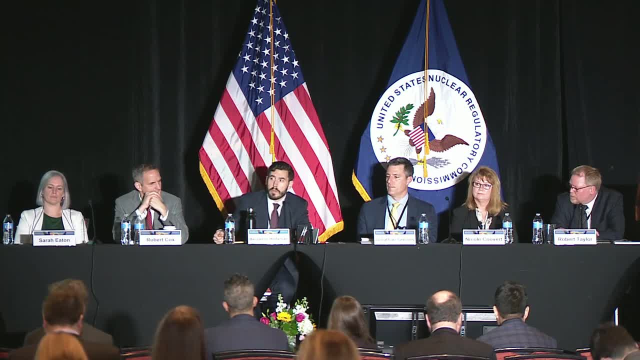 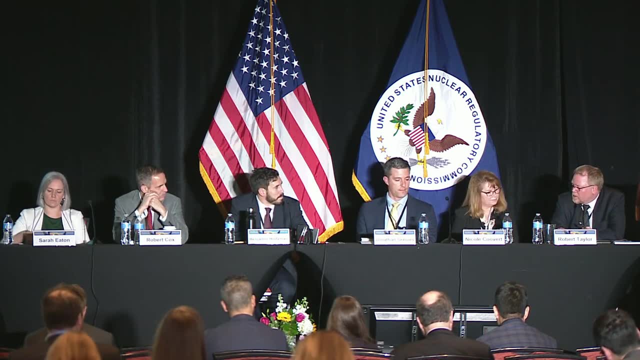 to the different technologies to yield an acceptable and workable solution. Said maybe another way. I think we share a common vision is that the tool, if built properly, will focus you on the right things to inspect, And those will be different depending on the technologies. 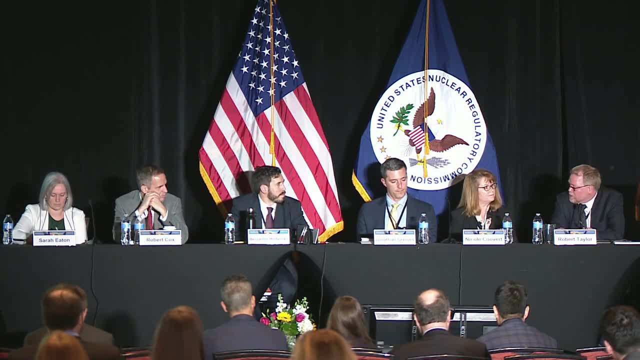 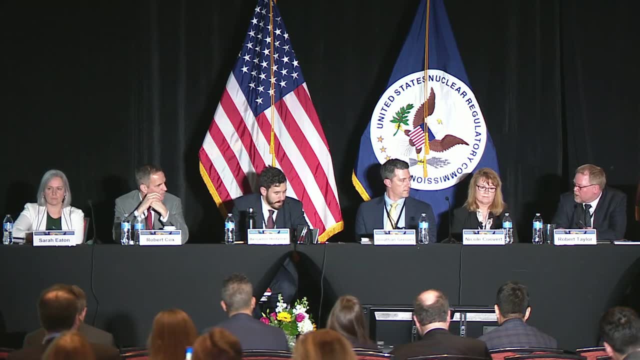 but shouldn't build it overly complex for one technology versus another. And you want to test the program over and over again with sanity checks to make sure it's focusing on the right things. That's part of the assessment program. Yeah, Yep, great. 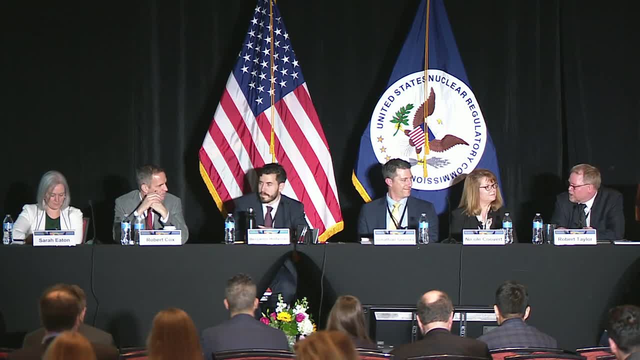 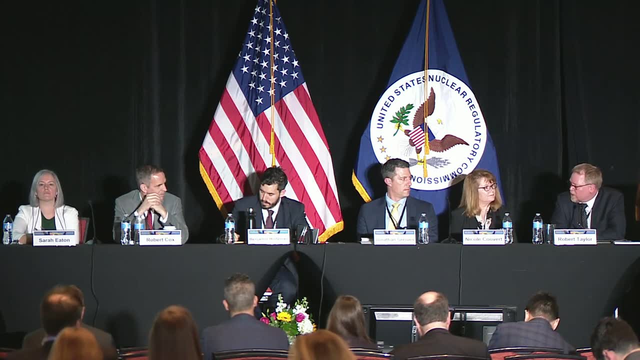 Robert, love the technology. Yeah, Love the idea of leveraging the technology. I had the opportunity to work on Vogel and Nicole did as well. We saw a number of challenges with the first-of-a-kind construction that Vogel was going through. 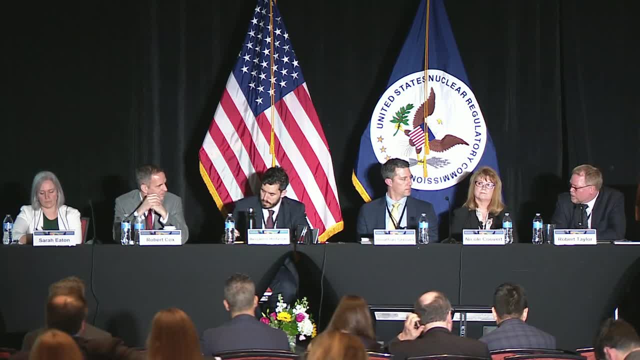 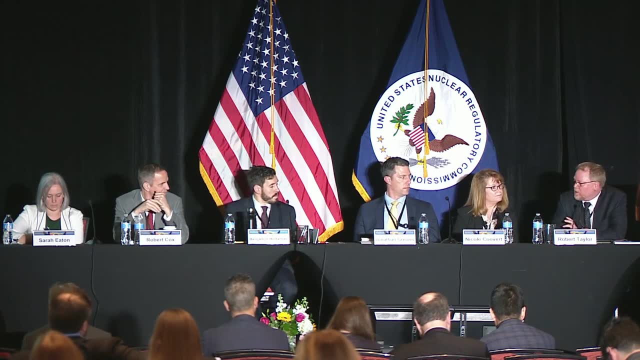 And we saw with Unit 3, they encountered some challenges. they learned from those and then they applied them to Unit 4, and construction went much more efficiently. How can the technology help us avoid those first-of-a-kind challenges for new construction builds? 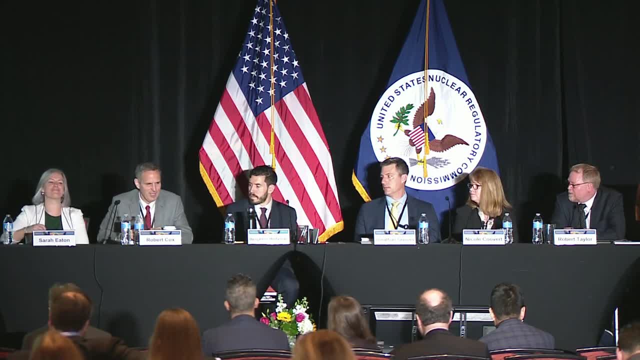 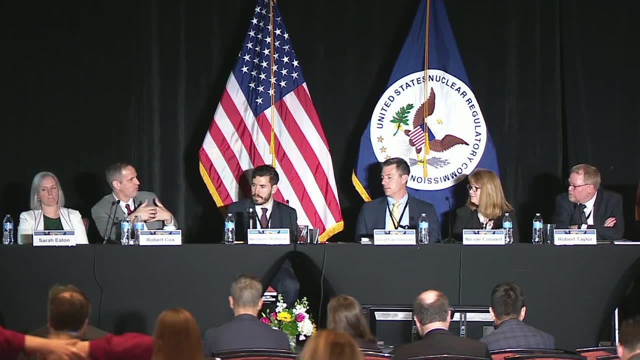 Yeah, Well, that's a good question. You know, where it really begins to help is when I do second-of-a-kind right, because you have the ability to carry the information through and you don't have to rebuild everything in the same way that you did before. 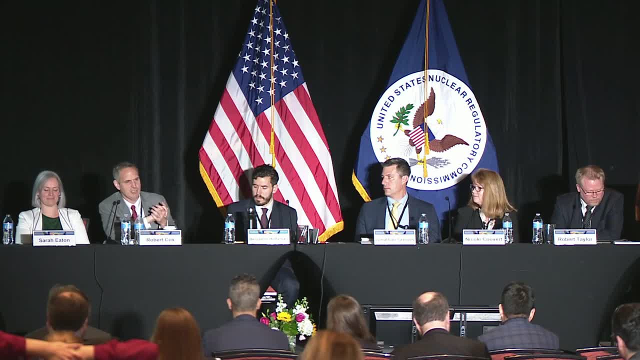 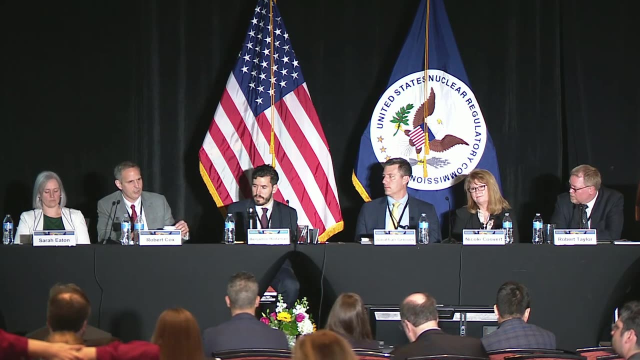 Effectively. you're building twins, I guess, if I use that, continue with that terminology, You know, I think, as it relates to the first-of-a-kind technique- again, I think a lot of it is- we need to begin to look at how we leverage the technology to build, you know. 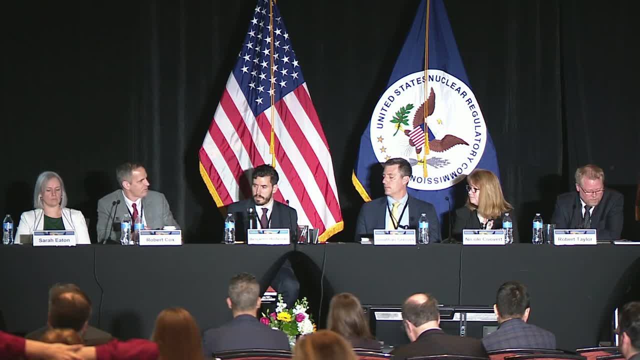 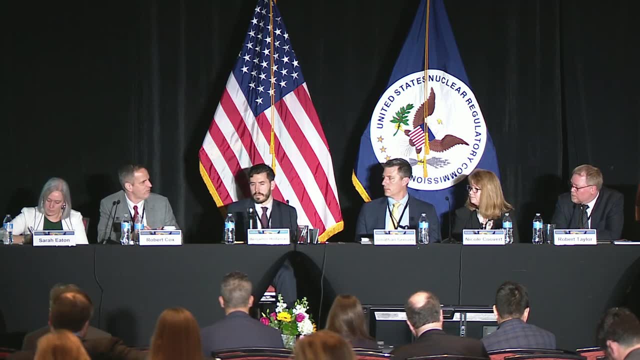 to build out better QA processes right At some level. that's really a lot of what the tool is able to, or tools are able to do, is to leverage those technologies. My fear is, what's going to happen is that, as you do, first-of-a-kind technology is going to be both costly. 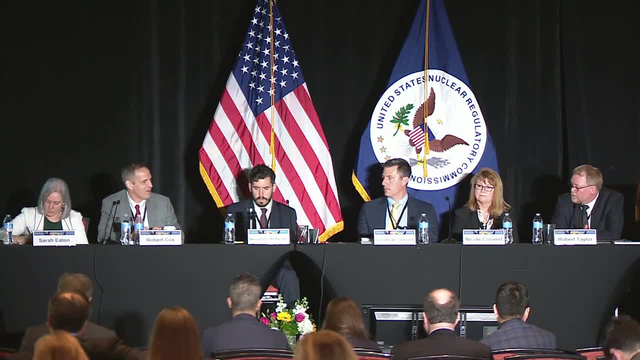 and potentially slow things down, And that's the fear that I think I have with a lot of the use of technology, that the advantage is probably going to come further down, Okay, Mm-hmm, And so that's something that I think that needs to be worked. 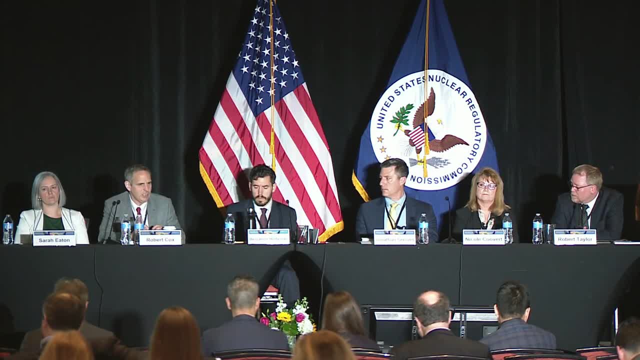 through for sure. but you know, it's clear that you know particularly for, you know, looking at, you know, for instance, some of the things that we've seen with in talking to folks at Vogel: the opportunity to be able. 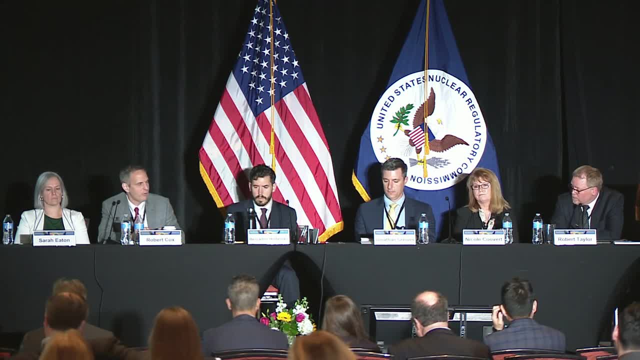 to leverage technology for QA, QC. I think that's where you know, I think we see a lot of the advantages and opportunities For first-of-a-kind. I think that's where it really does get to be challenging, Because my fear is that it could slow things down. 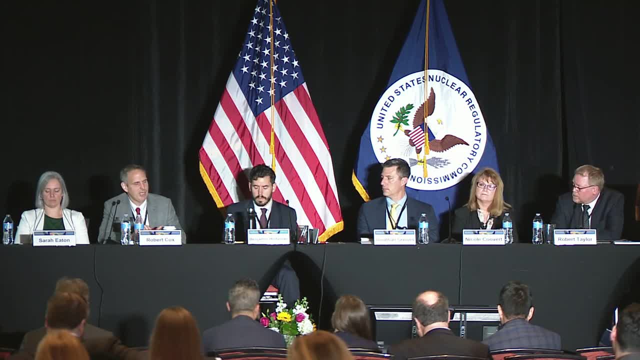 when you're testing and piloting things. But I think you know, I think it's, once you break through that, I think you're going to see that the benefits are exponential as you begin to move to two and three and beyond. 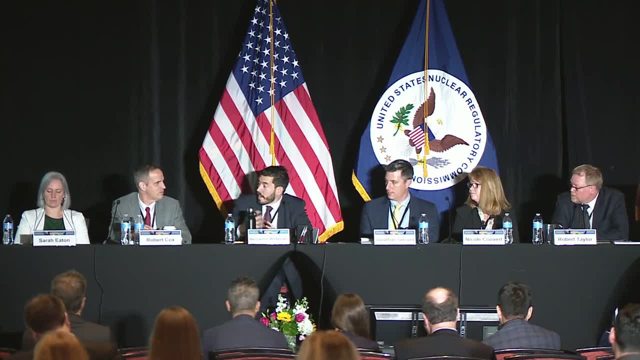 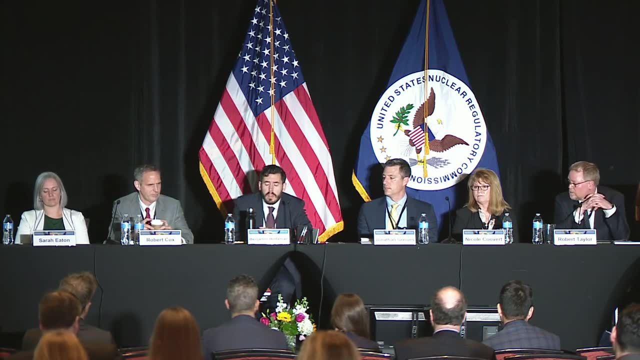 So, Ben, you want to weigh in. Yeah, I want to add to that a little bit, I think that. so I think certainly you're very well stated that you know, in order to when we build the models, when we put all the pieces in place, that's additional cost. 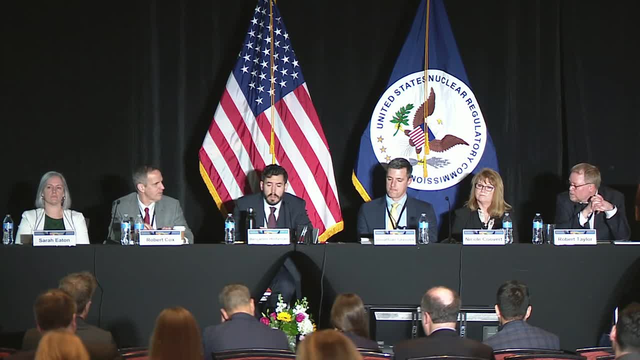 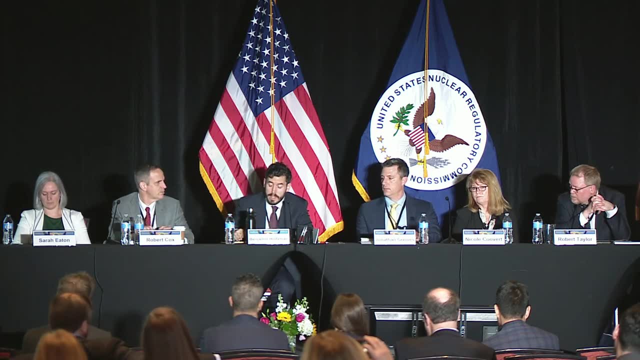 and there's additional effort in order to do that. I think one of the things that these tools will help us do is there's some aspects that I think the tools will help us do, and I'll come back to that in a second- But I think the sheer act of ensuring that we have all 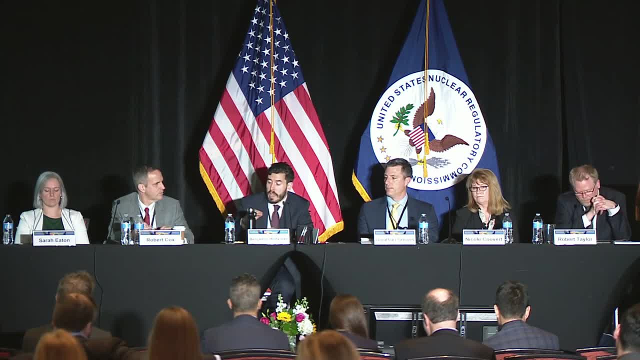 of the information to the level of detail that we could use. the tools will help us a lot for the first-of-a-kind deployments, Right, And I think the challenges that we've seen are not related to okay. well, is the tool itself going to cause challenges? 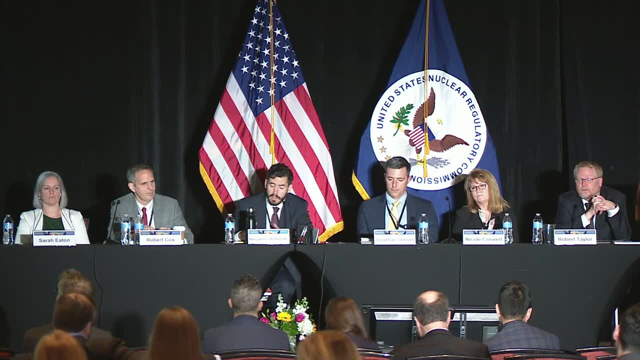 But it's related to well, we didn't have the design finished enough And we weren't able to have. we didn't actually have the supply chain set up to have this piece come in And the work when we had the workers actually doing the. 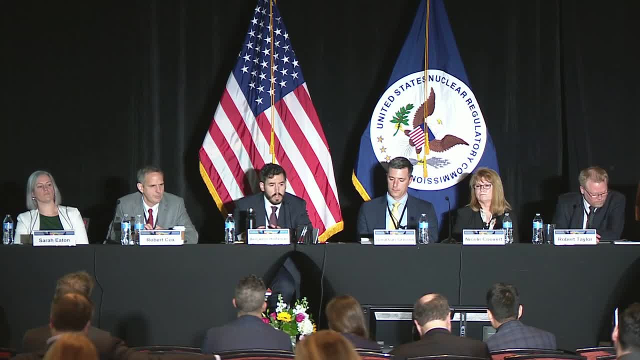 construction activities at the site we didn't make, we didn't realize that we had an issue, and then we weren't sure where those were, And so I think it's really important for us to be able to make sure that we have the tools that we need. 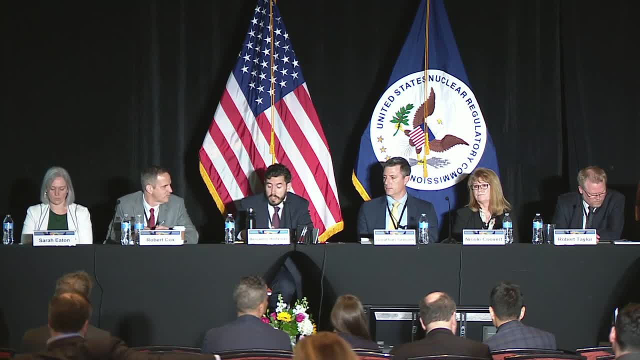 to make sure that the workers were going to be able to go because they couldn't do the activity that we originally had them planned for for that day, And some of the tools. some of the advantages of setting up these advanced tools is that now, 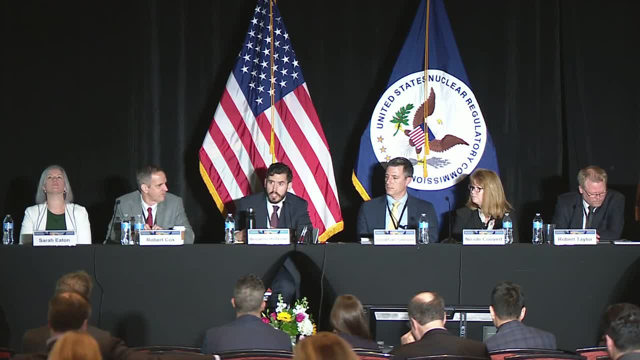 because I can see better the totality of the project. I can say, okay, well, this was late And, yes, that'll improve as we move down the- you know the- from first-of-a-kind towards end-of-a-kind. 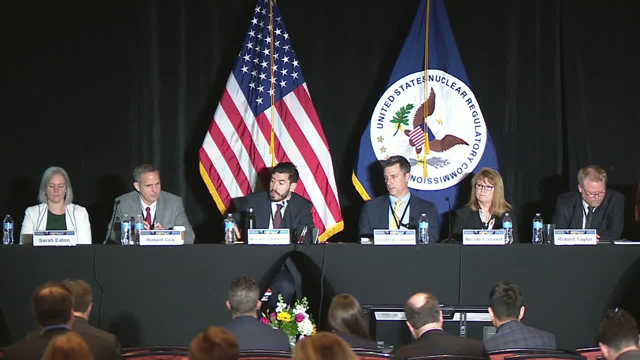 But if I know, okay, I can move these workers over here to do this other activity, because all of these components are available. even though that's not necessarily the thing that's most urgent on my schedule today, that enables me to still move projects forward in terms of completion. 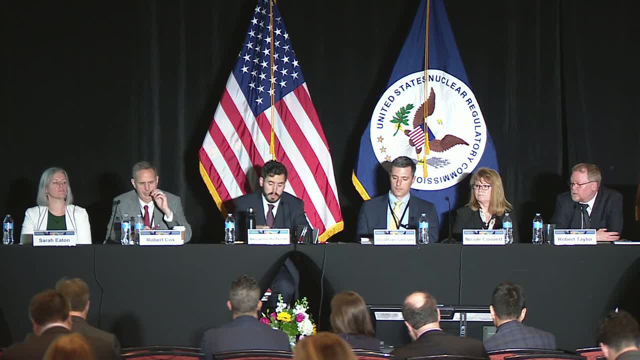 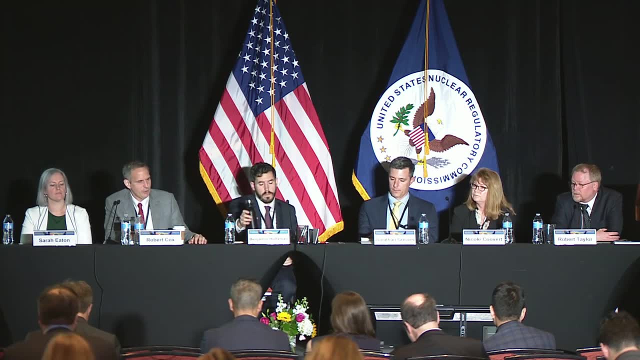 So I just wanted to add that to your response, but I think that was, And I just I don't. I mean, those are a lot of the driving principles that you would look for And I think, just the notion that you would be able to. 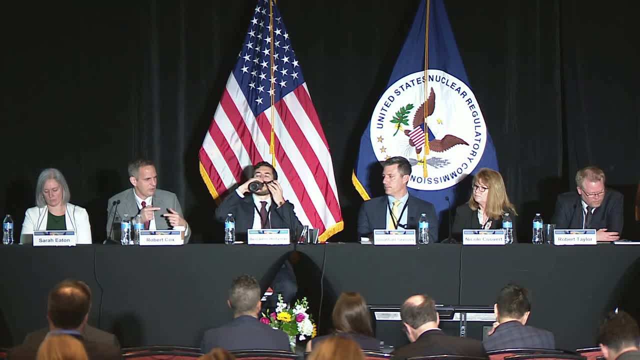 you know, in nuclear I think it's always, you know, is the design finished? You know we want to be done. done is always the term that I hear, but you know you have much more of an ability to be able to do a lot of these what-if scenarios. 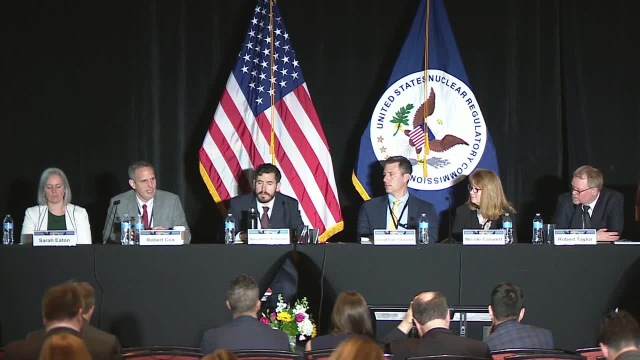 in construction that Ben was talking about, And I think the challenge, you know, is really just to say, once you have that ability, you can start asking a lot of questions, And I think the fear that I have for the first couple is: 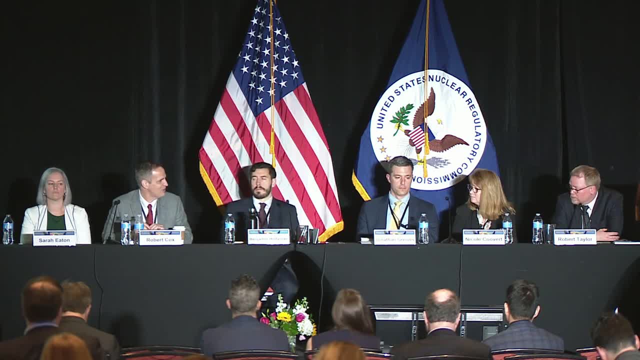 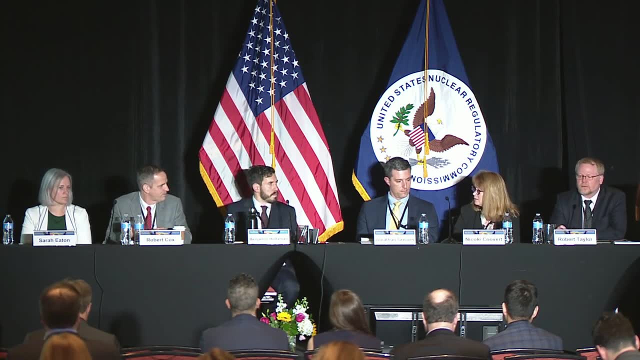 if you begin to ask too many of those questions, does that ultimately slow things down? Yeah, And I would say that the size and flexibility of the projects will have a big impact on you know the impacts of first-of-a-kind issues. 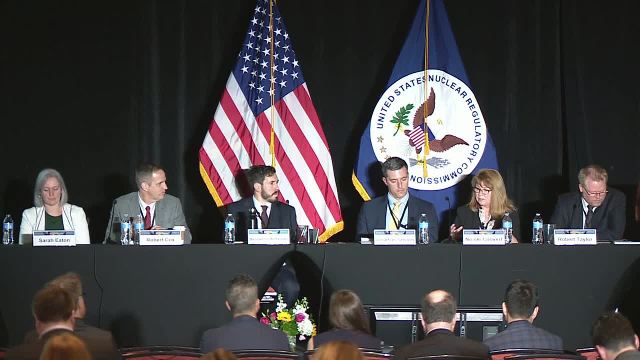 You know when you're talking about a design that is robust, that has, you know, less significant safety welds or components or systems or testing. you know those kind of if you have learning growing pains as you're working through these systems, it's not going. 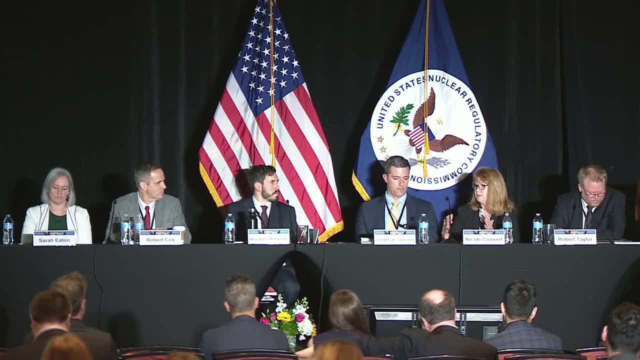 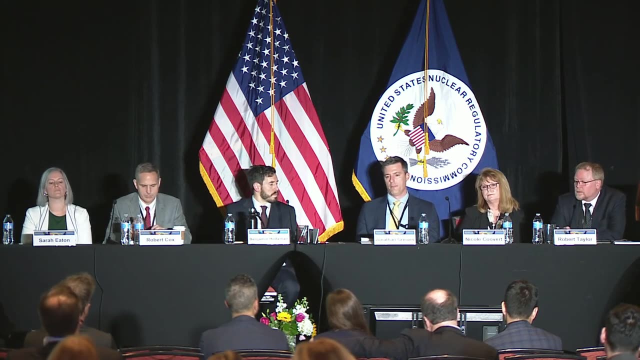 to have the significant resource timing scheduled delays that you would for a large light water reactor. So you know there's going to be some pros and cons to this new type of technology. Also, you know, maybe to add from an oversight piece too. 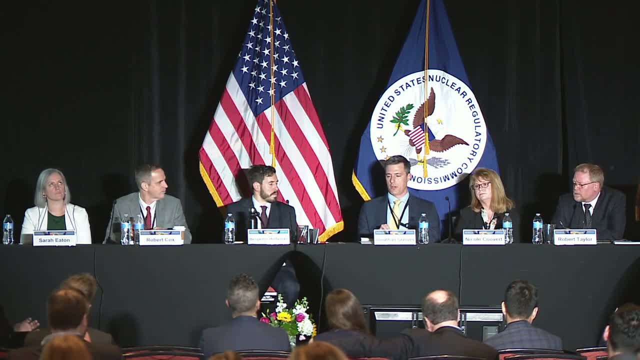 I think digital technologies, you know add. There's when we talk about risk-informed, I think design risk is fairly well understood. This component, this you know vessel has, is of such and such safety significance because in this accident scenario it performs this function. 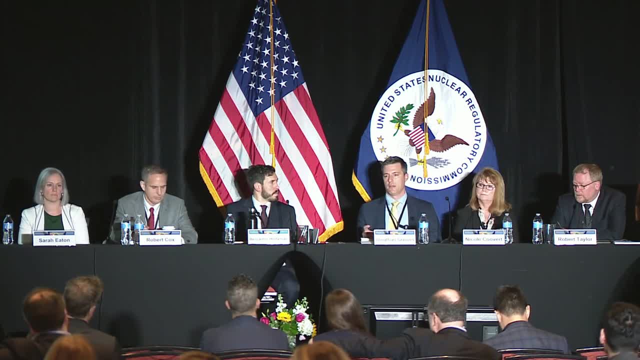 But the other aspect of risk, you know, the other aspect of risk-informed that we think about in construction oversight is construction risk And the way we talk about that is what's the likelihood that a deficiency would make it to operations, And I think some of the digital technologies that allow 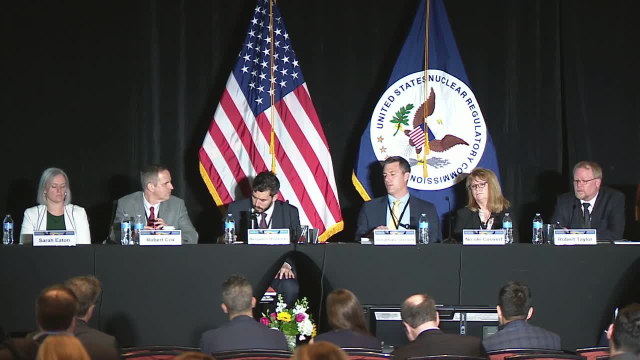 for self-checking. you know, one of the features in a lot of digital IFC systems that are being deployed is because you can eliminate a lot of different testing because it's going to self-test all the time And if there are technologies out there that are being deployed, 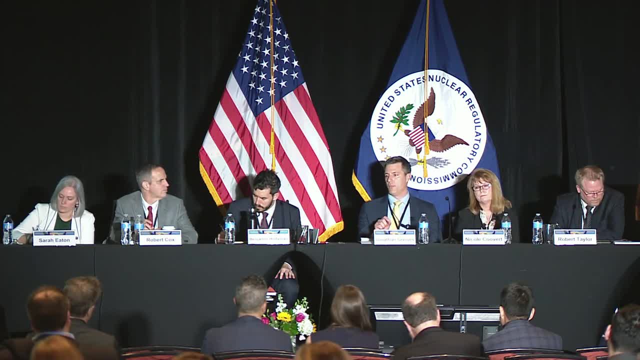 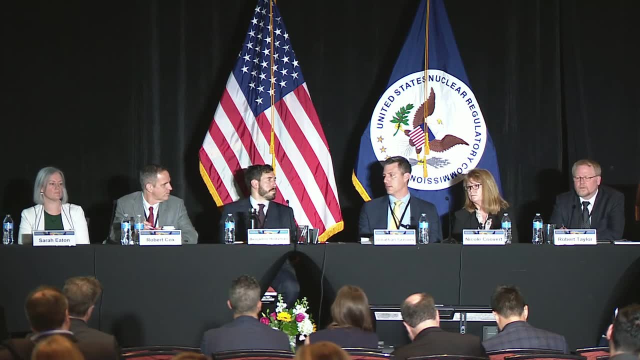 that ensure that deficiencies are, you know, recognized very quickly and then can be brought into the models and resolved. that lowers the construction risk right And we need to be able to factor that into our decision-making to reflect that right And so we shouldn't necessarily need to inspect. 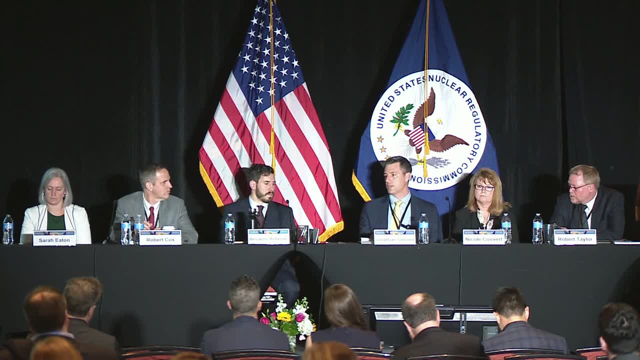 to the same degree, if the system's inspecting itself, And maybe what we're actually looking at is, you know, part of the QA check is well, what sort of self-checks and you know QA attributes are being employed at that level? 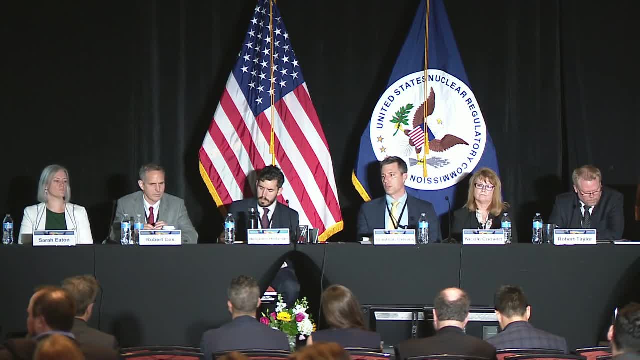 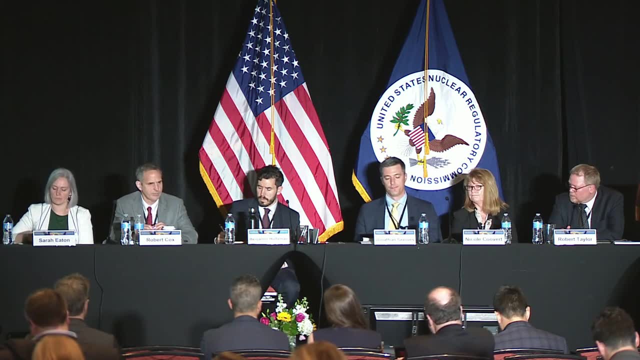 So I think you know, even on first of a kind, I think those are things we need to be aware of and certainly make sure it's factored into our decision-making. Great, So we have three minutes left and I want to get one last question in. 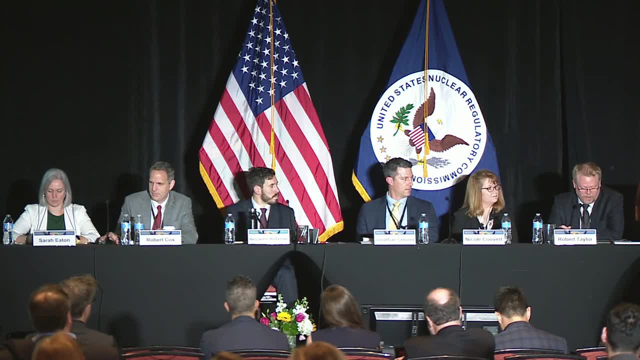 because I think it's an important one and it gives us an opportunity to talk about something that we haven't had a chance to touch on. So I'm going to direct it to Nicole and John just a little bit here and invite others to weigh in. 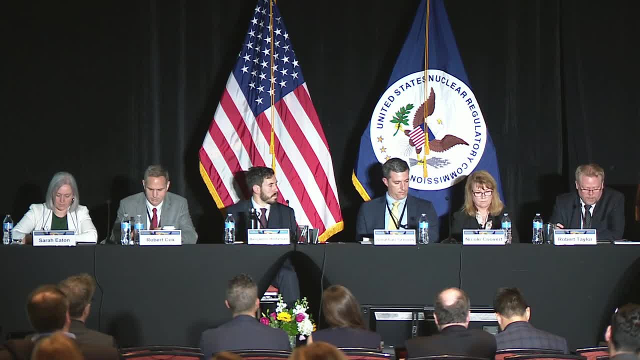 Some new reactor designs claim that the fuel cannot fail, which serves as a key assumption for the overall safety case. With this assumption, there seems to be a heavy reliance that fuel design and manufacturing is of the highest quality. What are we doing with fuel manufacturing oversight? 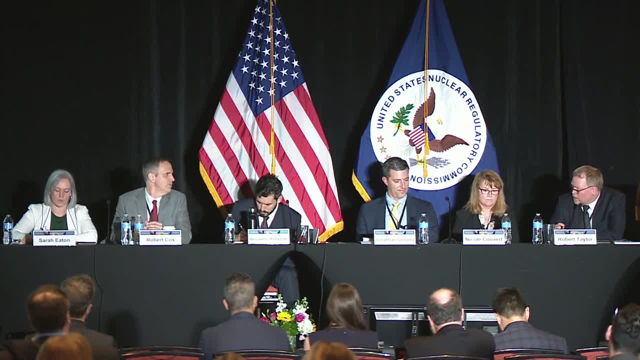 to ensure the safety case is met. Can you guys elaborate on how we're interfacing with those building the fuel cycle oversight program, going forward and making sure that we're integrated in our approach to overall safety for the facilities? Yeah, thank you, Rob. 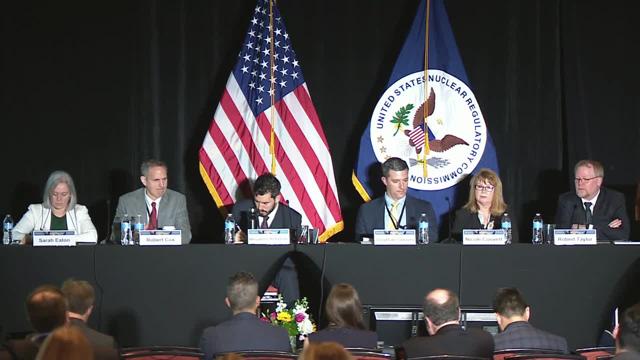 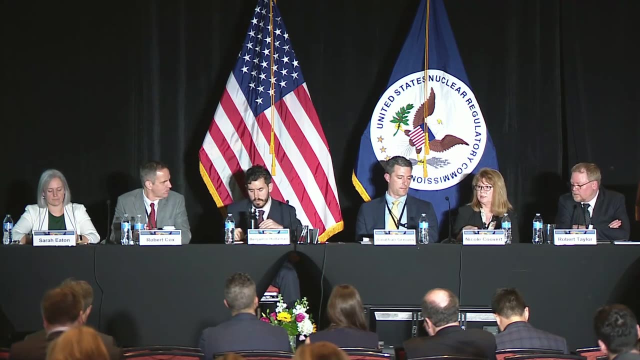 I think that's a great question because when I talked about earlier in the presentation, about a holistic approach, this perspective on oversight framework development for scalable, flexible, technology-neutral, this is not isolated to our comp. This is for fuels, fuel facility. 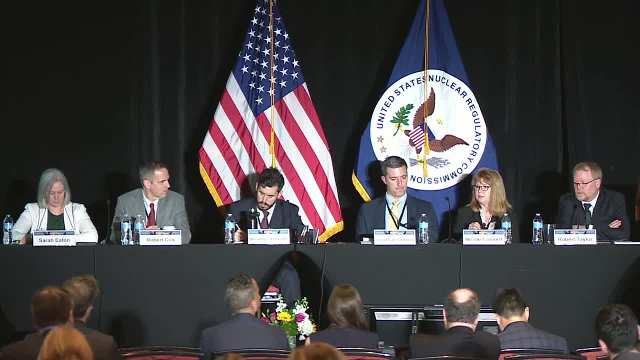 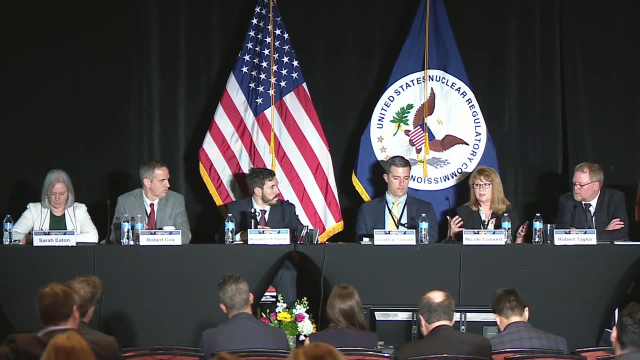 This is for the non-power production utilization facilities. This is the fuel cycle, the life cycle of the fuel system. So what's happening is with fuels, because it's the first to be developed. we're working with the program office. the same folks are working. 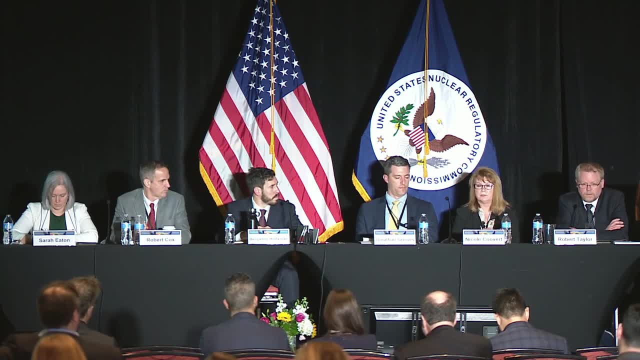 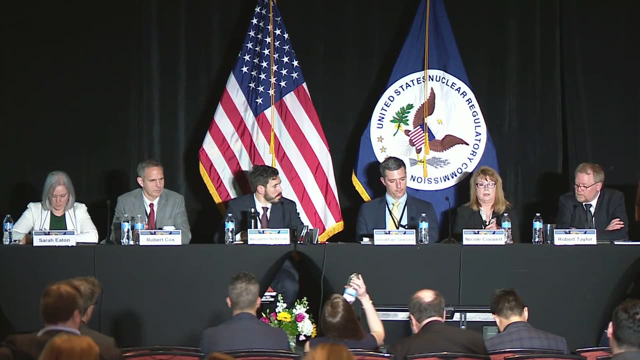 with the program office to ensure that our inspection guidance is scalable, is flexible. it's able to consider the different fuels that are going to be built to support these new advanced reactors. We're also going out, we're working with the program office and the licensing application- our applicants. 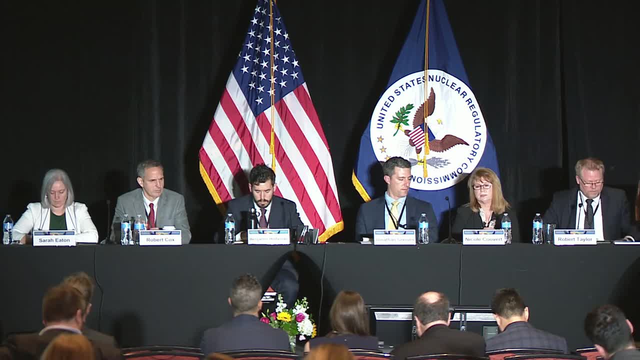 We've had several public meetings, the same as John mentioned. As John was talking about for the R-COP, the workshops having open platform communications to have these dialogues, because they're also asking the same questions from you know, fuel cycle perspective. 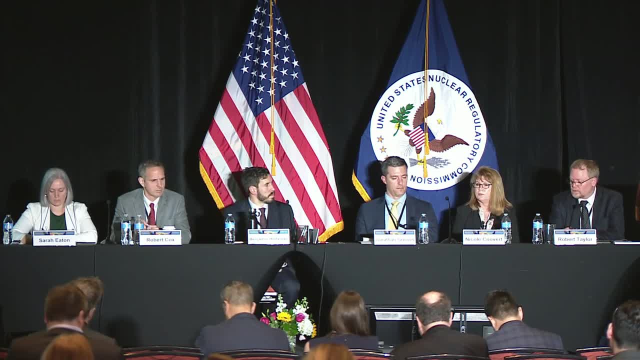 So it's an important time for the regulatory framework and we're trying to be at the forefront of this new, this new generation of advanced reactors, advanced fuel And the fuel cycle is absolutely part of that key program. Great, So we have just under a minute. 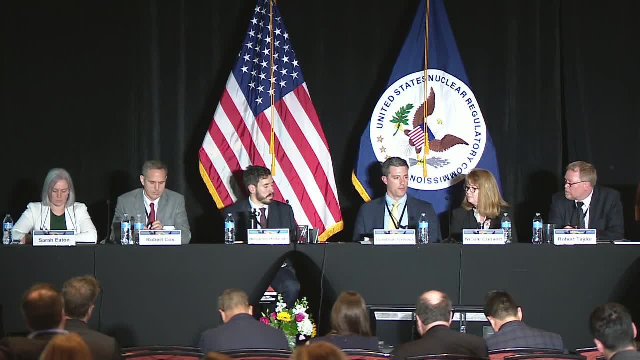 Anybody else want to add to that? I would probably just also add in: you know, we certainly are leveraging and partnering with the research and test reactor oversight which you know. as Ben mentioned before, some of these new advanced reactors are 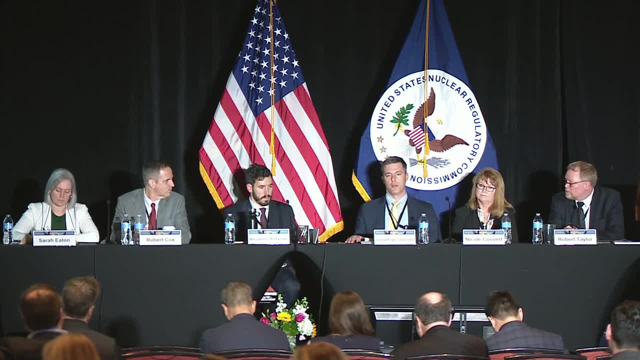 going to from a risk standpoint, may look a lot closer to what a research and test reactor. So although they, you know they have a separate oversight program, we certainly need to learn from them, leverage their experience. It's a good opportunity to benchmark and look. 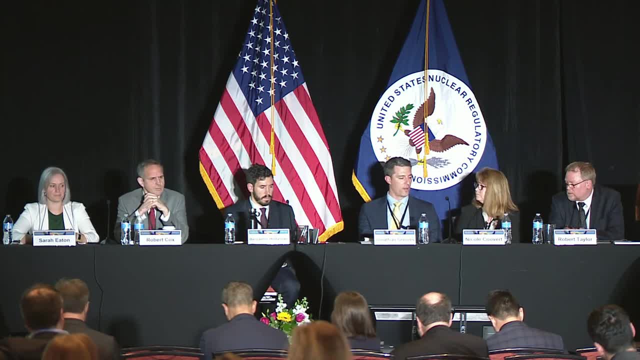 at how our decision making process, how would it apply to an RTR and is it right sized? Would it give us a right sized approach or not, And then go back and adjust? So that's another program that we're certainly stayed tied in. 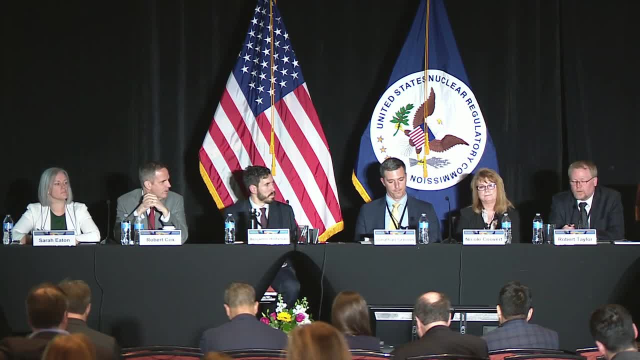 Yeah, that's absolutely included in the overall framework. Well, great, So we did not get to all the questions here, So if you did not get your question answered, we'll be around here shortly after this, So please come up to us, talk to us. 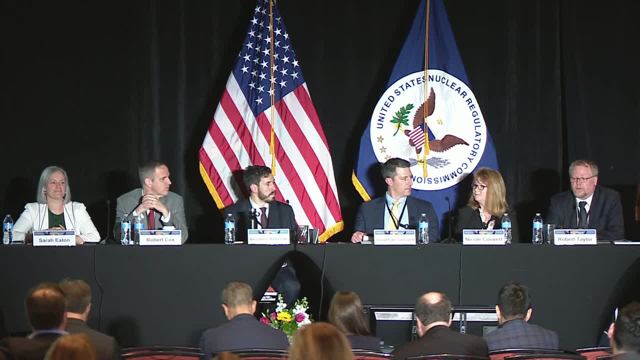 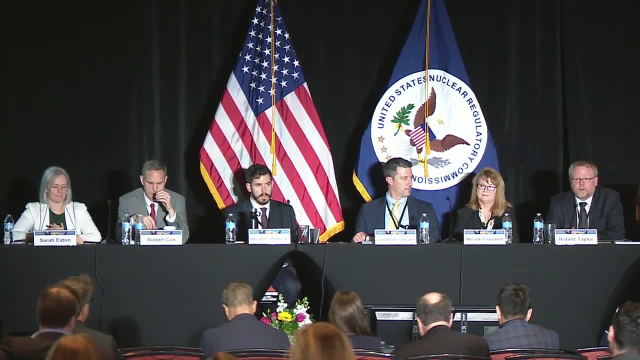 and we're happy to elaborate, Or if you had a question you didn't get a chance to put in, please do so. So with that, I'd like to ask the audience to join me in thanking the participants in the panel and their contribution. 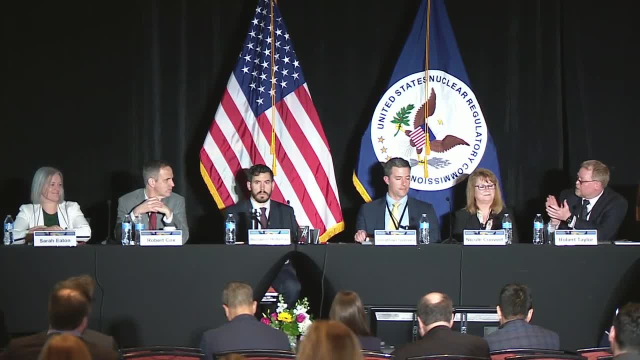 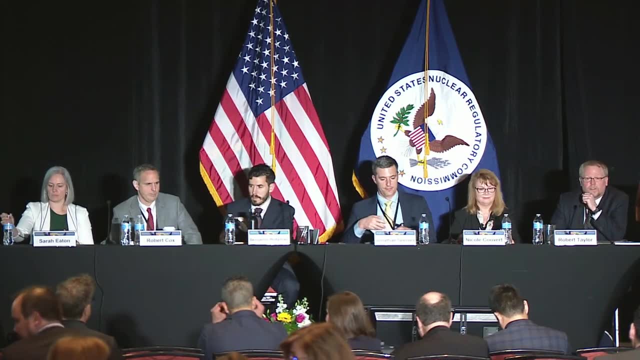 and their efforts on this very important topic. So thank you guys. With that, we'll close out the session. Thank you all.